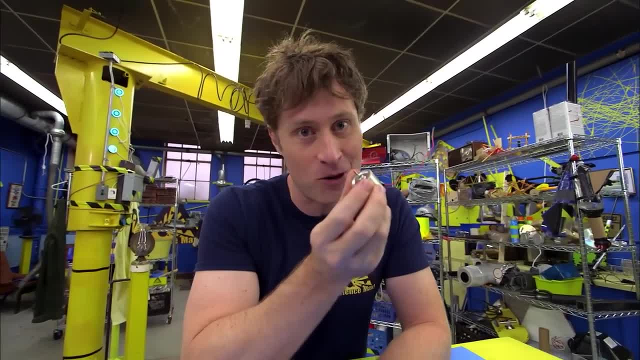 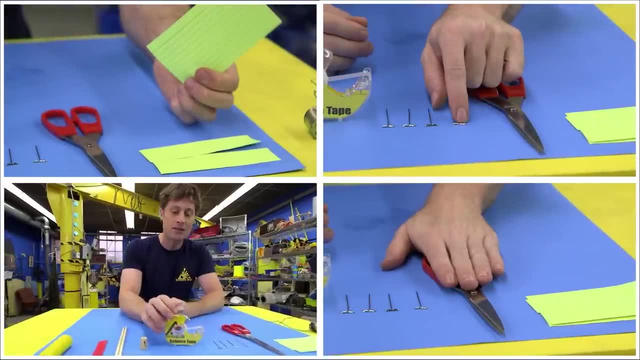 Just make sure that the toy is broken and that the broken part isn't the electric motor. Here's what you need: Index cards or construction paper, scissors, push pins, science tape. It's the same as invisible tape, except I use this one for science. 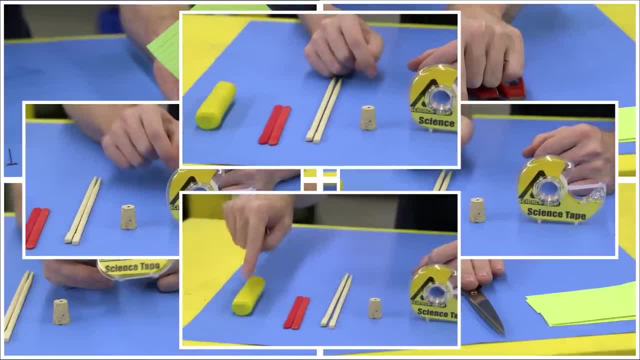 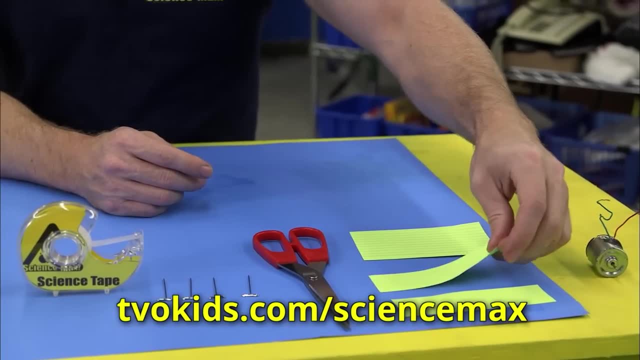 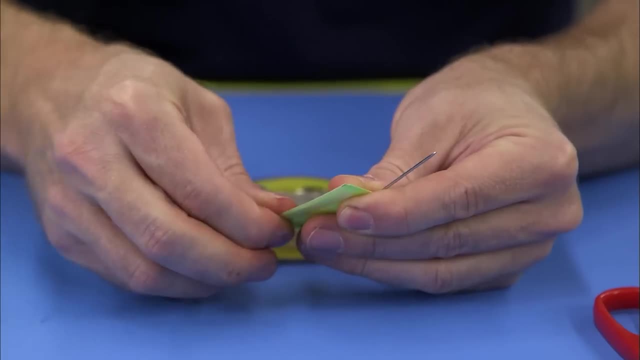 A cork chopsticks, craft sticks and modeling clay. And remember, all the steps for this experiment are on our website. To begin, cut the index cards into strips and tape down a push pin so it sticks out. Then fold over the index card and tape it together. 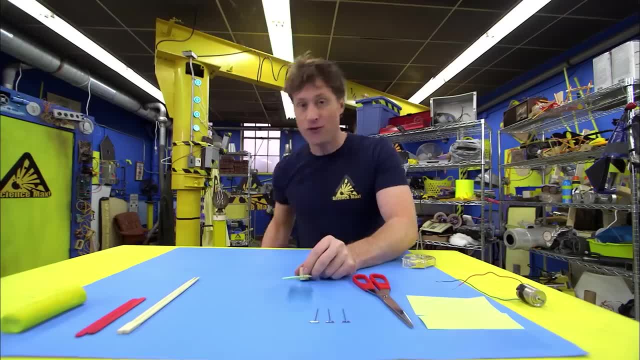 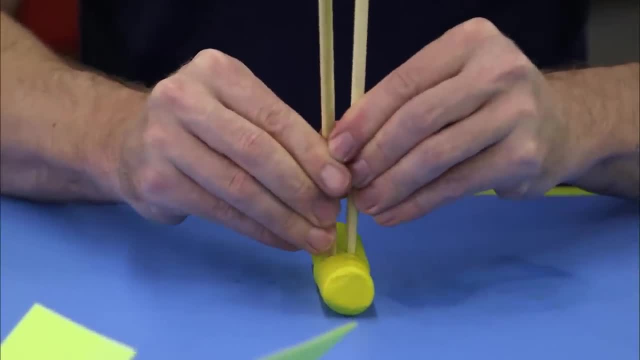 Then stick the pin into the cork and repeat that step. If you want as many blades as you can get on your fan, you're welcome to do that. Next, take your modeling clay and stick the chopsticks in, Then tape. the craft sticks in between with science tape. 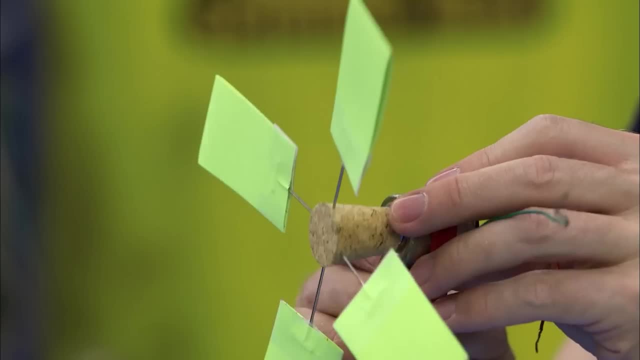 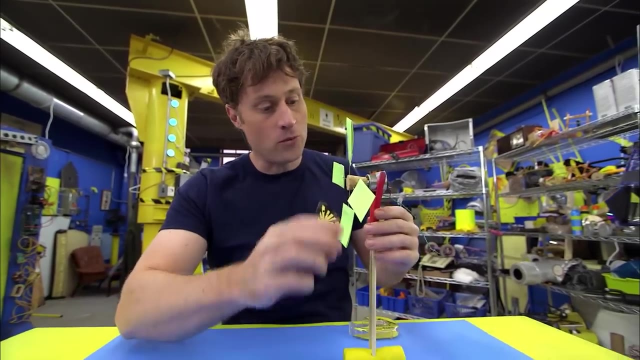 Then take the motor and stick the cork on the end. Then wedge the motor in between the craft sticks and tape it down so it stays put. And there you go, A fan that will spin in the wind. You want to adjust the fan blades? 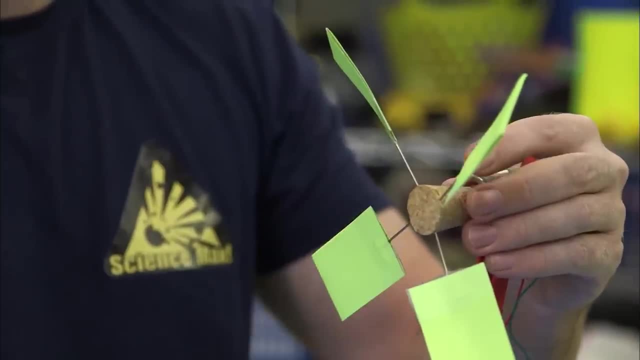 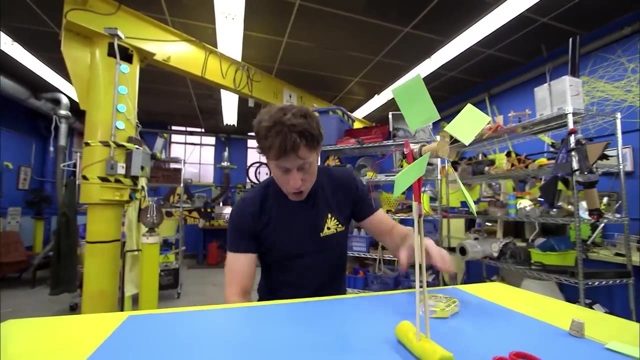 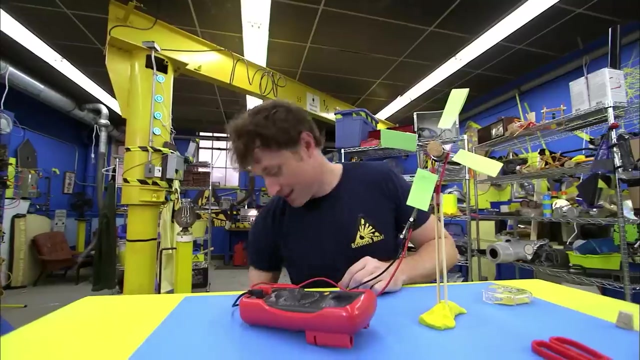 so they all face on a bit of an angle. That way they will catch the wind and spin. There we go Now. when it spins, it will create electricity. I'll show you with this. It's a multimeter, And a multimeter measures little amounts of electric current. 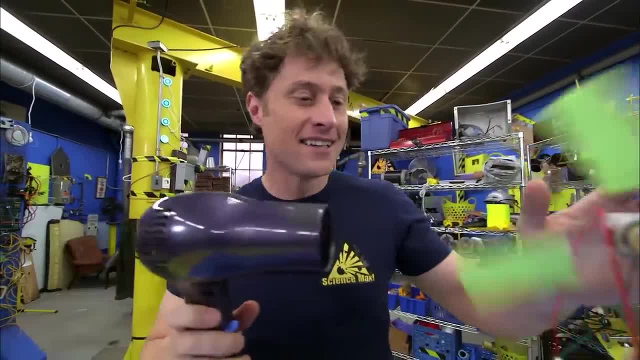 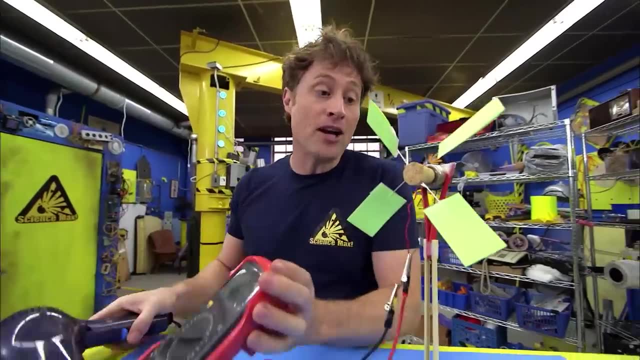 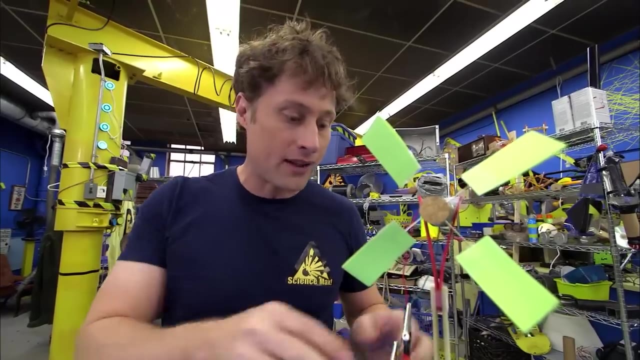 There, The hairdryer makes wind, spinning the fan blades, and we are creating electricity. Now, pretty much all electricity that you make comes down to turning a generator. A small motor like this isn't going to produce a lot of electricity. 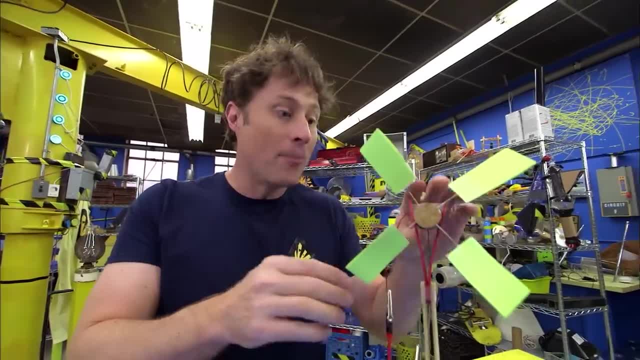 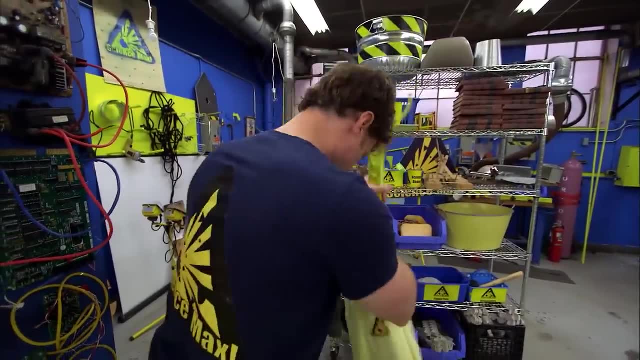 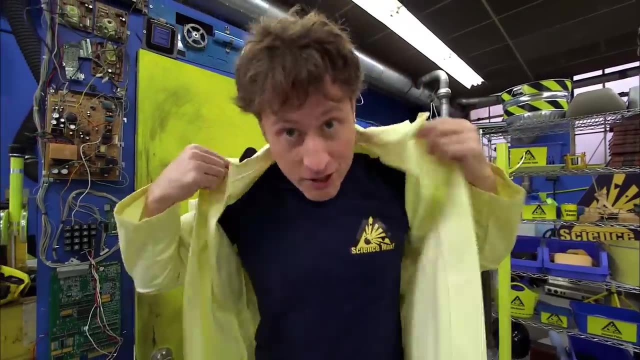 barely enough to power one tiny little LED. but it's a start, And a good start is all we need, because Today, on Science Max Experiments At Large, we're going to look at all kinds of different ways of generating electricity. Plus, I want to find out just how much electricity. 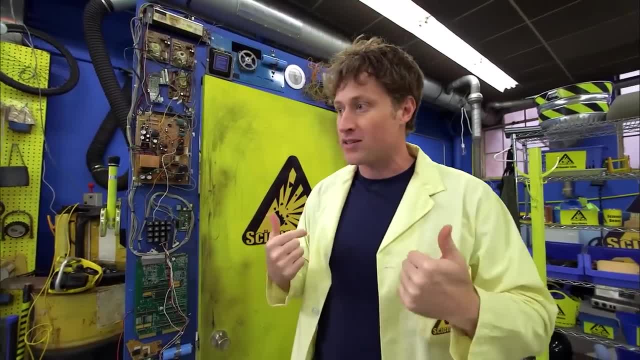 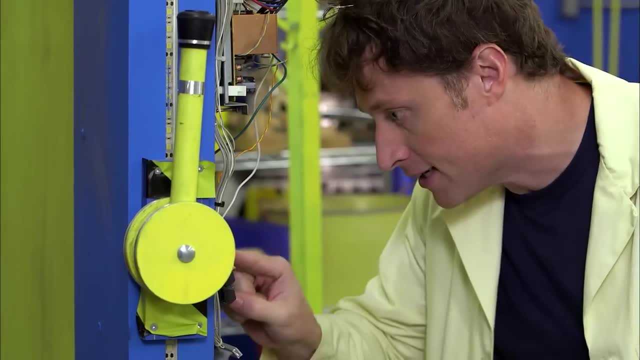 one human being can generate. Although one human being is going to be kind of lonely, I'm going to need an expert. Oh, I know Anthony from the Ontario Science Centre. He can help. I wonder if he's busy. Well, come on. 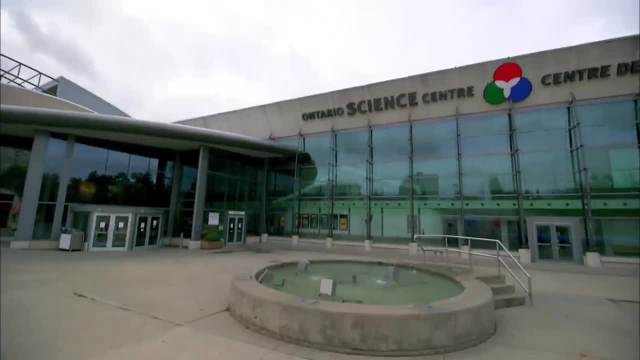 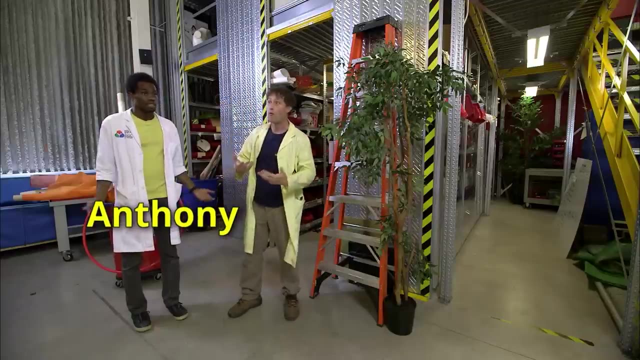 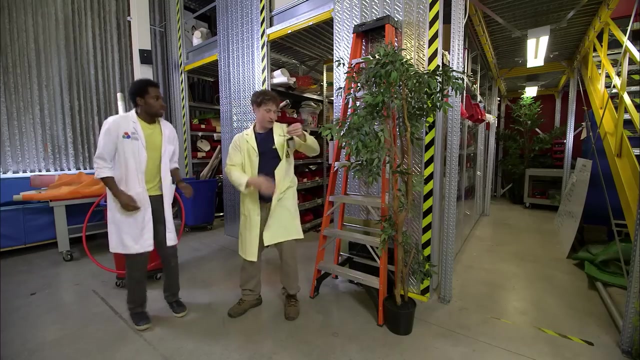 Let's go. Oh, Anthony Phil. So I was wondering if you could help me with an experiment. I want to generate as much electricity with human power. What do you think? I think that sounds awesome. Okay, great, Let's go back to Science. Max headquarters. 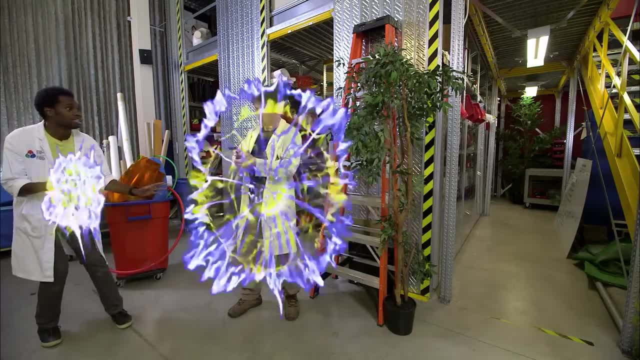 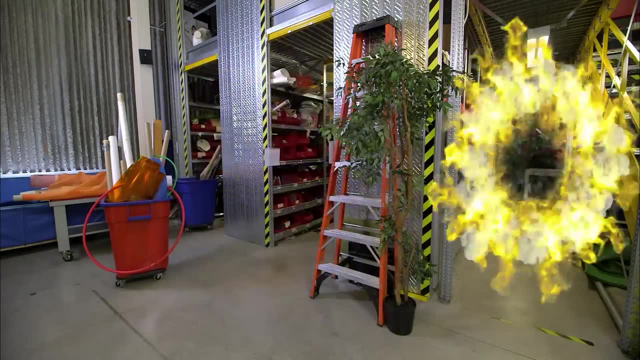 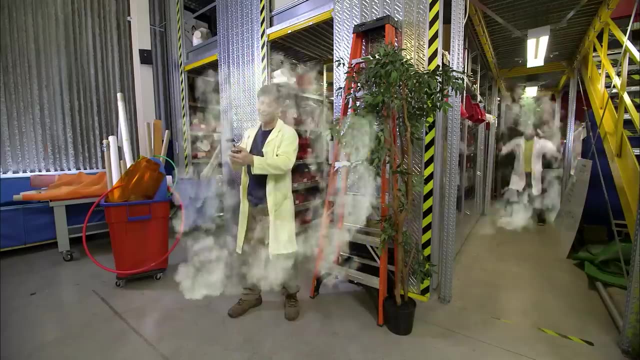 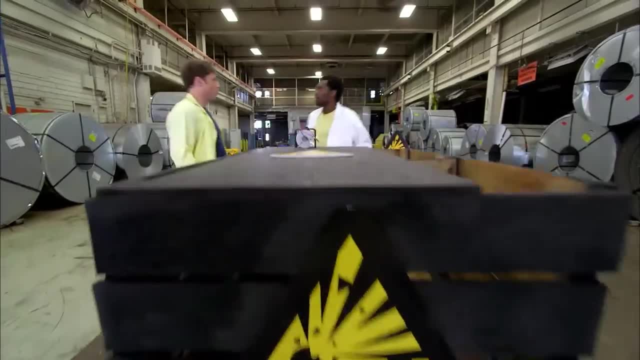 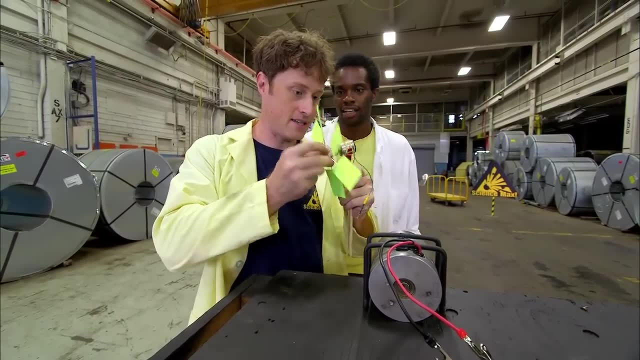 That's not. No, I know what it is. It's this: Where did you end up? I was in the vents. Oh, I ended up in the bathroom. Well, now that we're here, Okay, so this is what I started with, and this is just an electric motor, right? 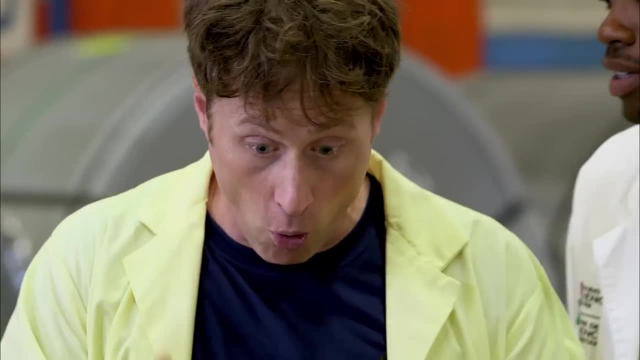 Right, So Right, Right, So you can generate electricity. you spin it, So I figured, in order to generate more electricity, you get a bigger generator. Exactly Yeah, The bigger the generator, the bigger the magnet, the more the copper. 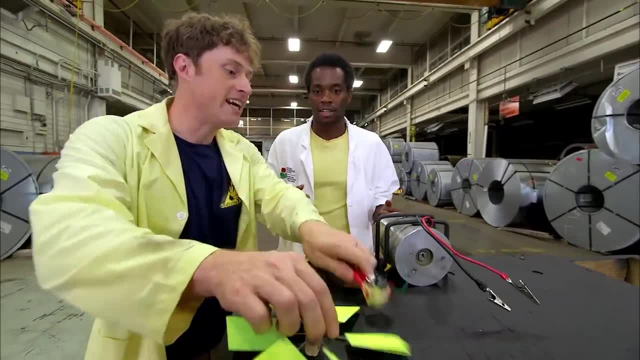 the more the electricity. Oh well, you know, what we should do is we should just get an even bigger one, like a giant one that they use in like at a power plant or something, or Not quite. That would be too big for a person. 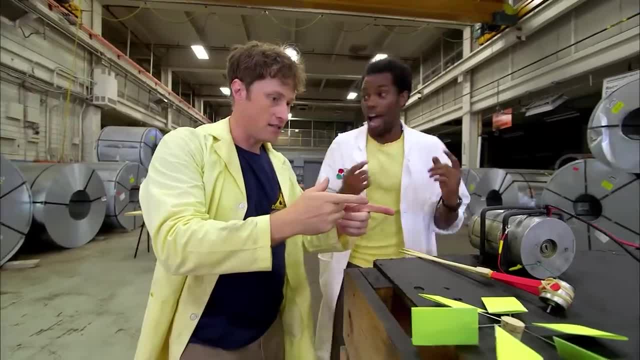 to be able to turn. It'd just be impossible. So you think this is a good size. I think this is a great size. Okay, so that's good. This is called a multimeter. We're gonna hook up the wires. 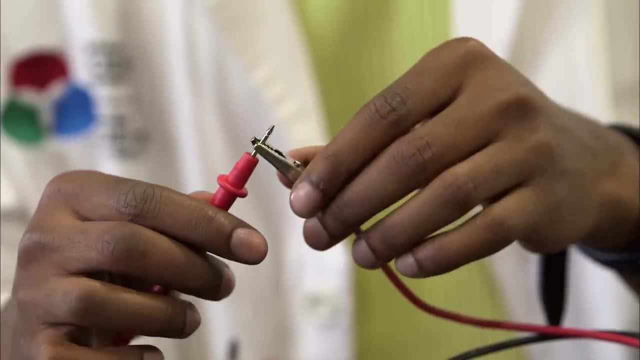 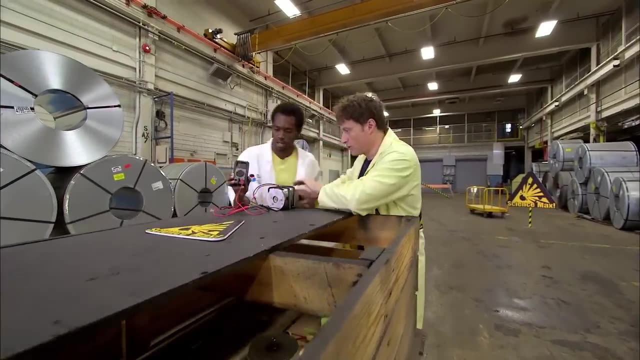 I'll do black to black, Black to black Red, And as you turn our generator, we can see just how much electricity we're generating. Okay, so Here you hold on to that And I'll turn the generator. Now it's time to play. 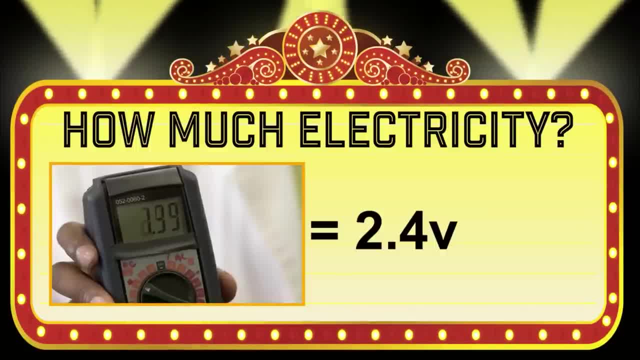 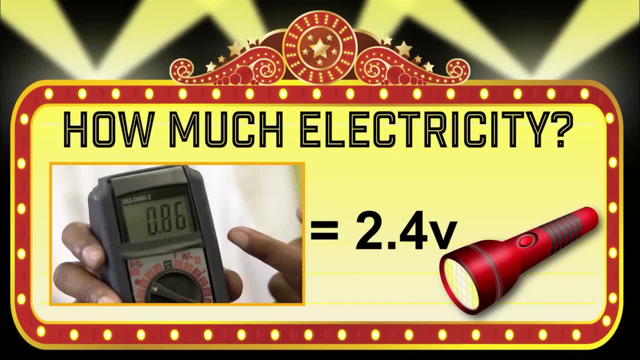 How Much Electricity Did They Make? 2.4 volts, yeah, it's not bad. Oh, 2.4,. yeah, it's not great. That's just enough to power a small LED flashlight. Better keep trying, boys. 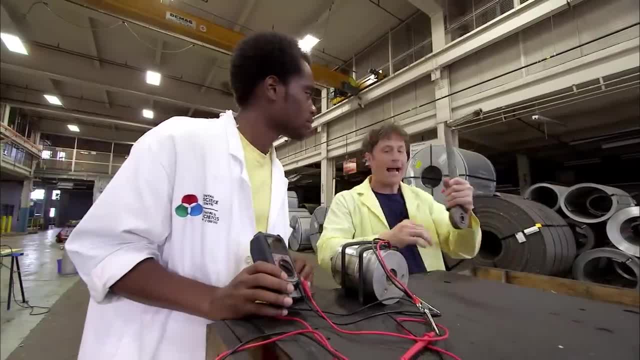 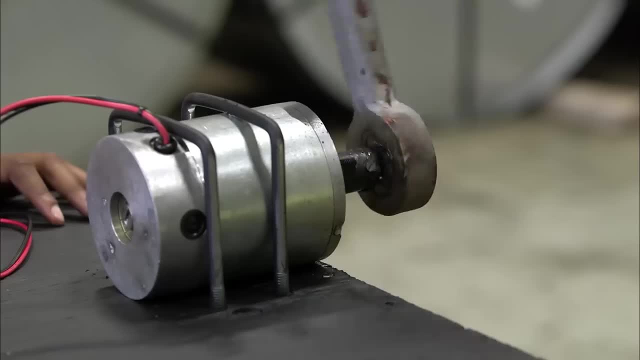 I got some handles here that we're going to attach- Ah, that was perfect- to the end of the generator so we can spin it. Okay, let's try. Huh, No matter how fast I crank the large handle, I couldn't make any more electricity. 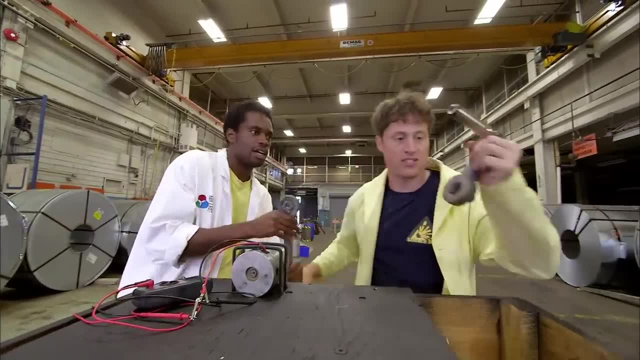 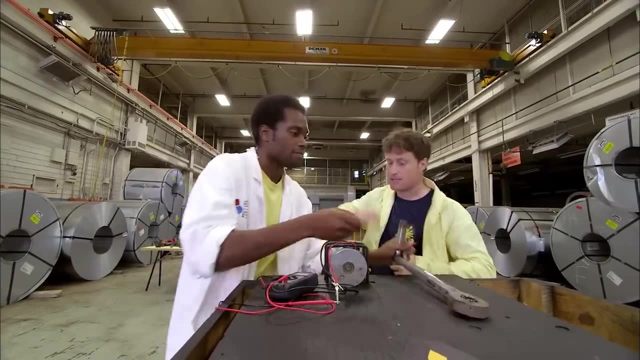 than before. Okay, let's try something else. I bet it's a smaller handle. Perfect, okay, yeah, That's good. Yeah, well, maybe it'll let us get more spins in. Oh yeah, because I don't have to make as big a circle. 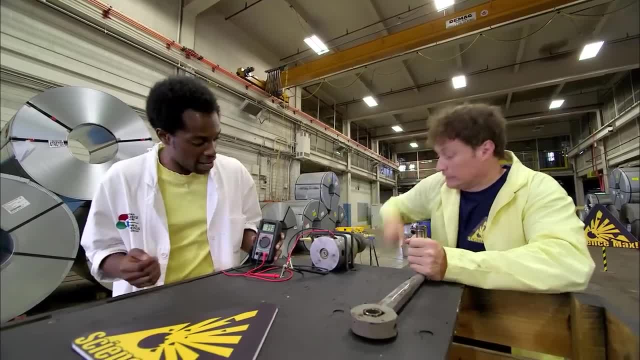 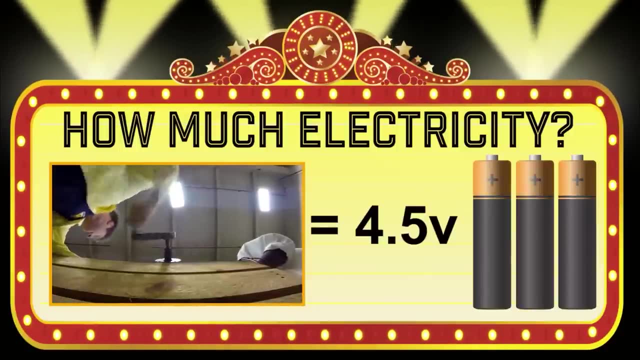 Exactly. Yeah, it's working. already We're up to like 2.5.. Now how much electricity is Phil making? 4.5.. That's the same as three AA batteries. Maybe enough to power a toy car. 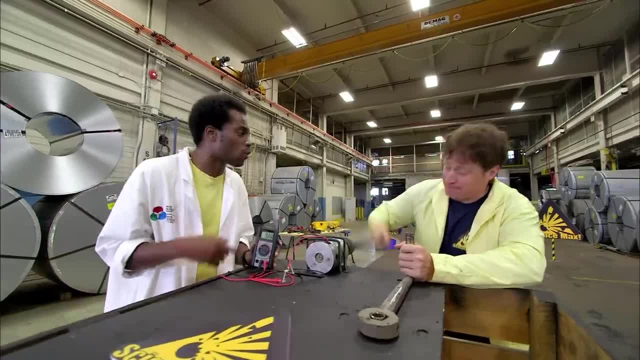 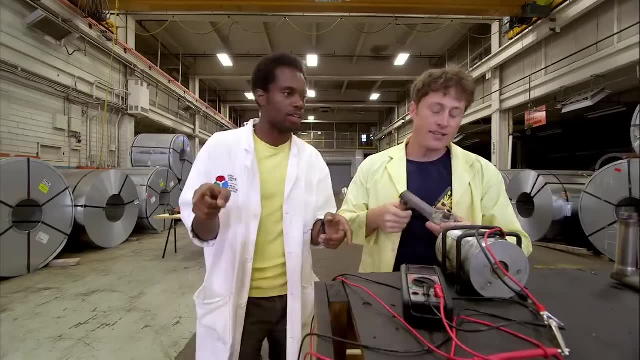 Still a long way to go. Yeah, it's a lot higher with the faster spins. Oh, all right, all right, You okay, I'm okay. Maybe we could use, like, some gears or something like that. Oh yeah, you know, that's a good idea. 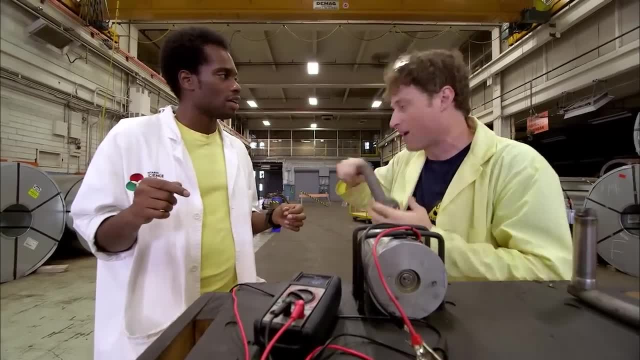 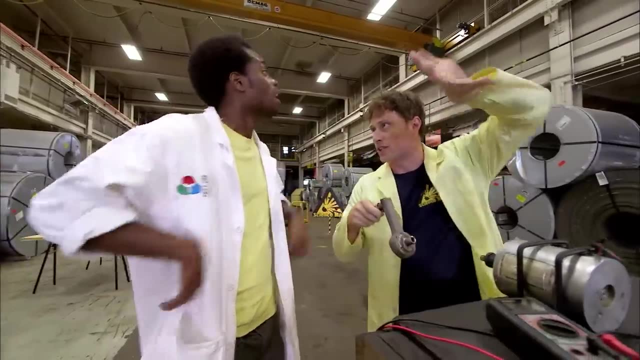 because the circle that I'm making here I can only go so fast, Yeah, So maybe with gears you can do one circle here equals like ten circles on the other gear, Exactly, Yeah, Okay, so kind of like the gears on like a bike. 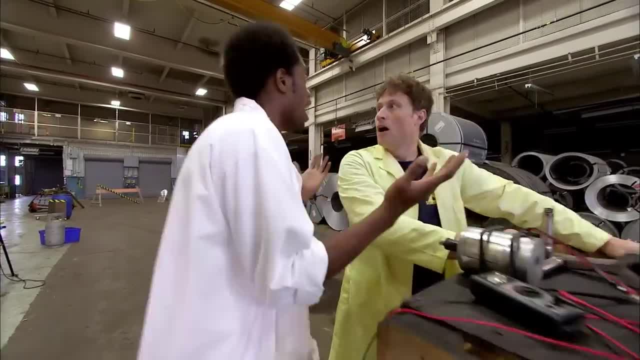 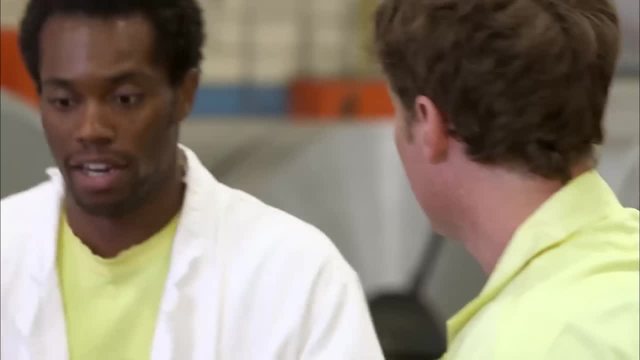 Yeah, the gears on a bike, or something like that. A bike, Of course, Yeah, so okay, so we get a bike and we attach the, the back tire, to the generator, The generator, and then you can use the pedals of the big gear. 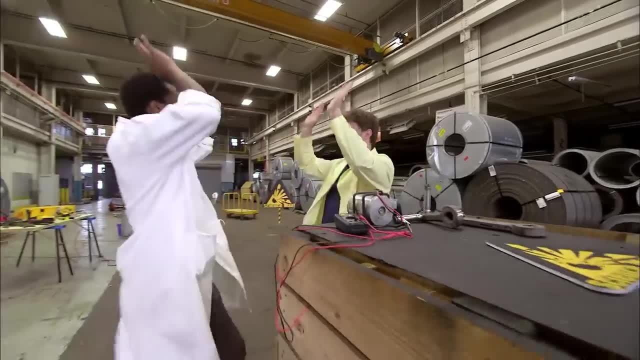 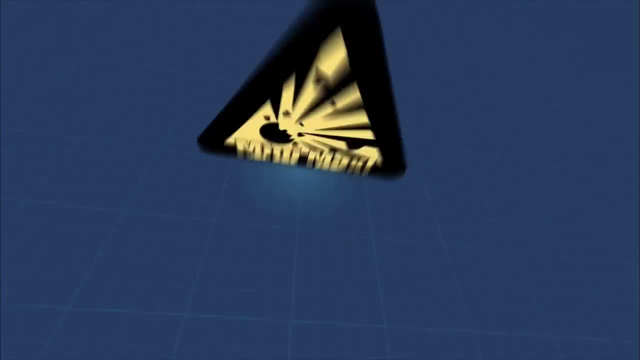 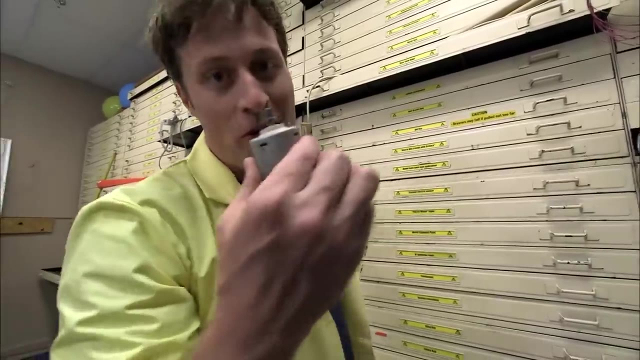 to power the small gears. Okay, great, We'll go get a bike. Yeah Yeah, high five, All right, All right, Oh right, they're over here. This is a generator. It generates electricity when you spin it. 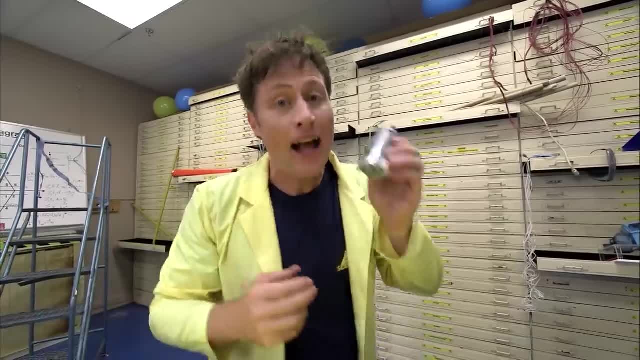 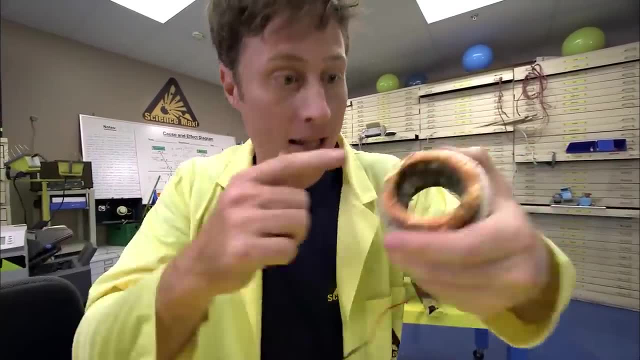 But how does it work? What wizardry is inside? Well, actually generating an electric current is fairly simple. All you need is two things. First, you need a conductor, like this coil of copper wire, and you need a magnet. 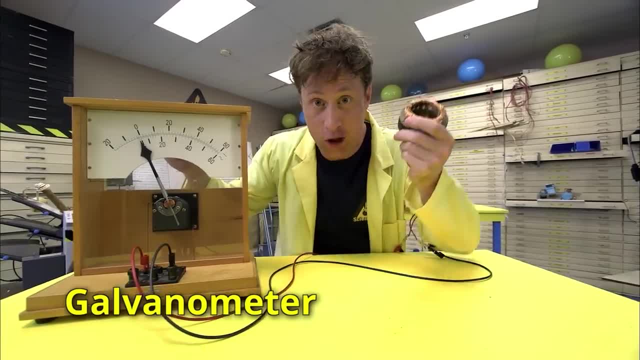 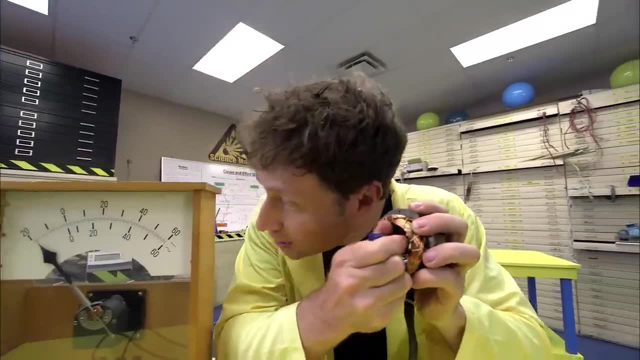 Now, this is a galvanometer. It measures small amounts of electric current and I have my copper wire attached to it. Watch as I put the magnet inside the copper, I get a little bit of an electric current, and then I take it out. 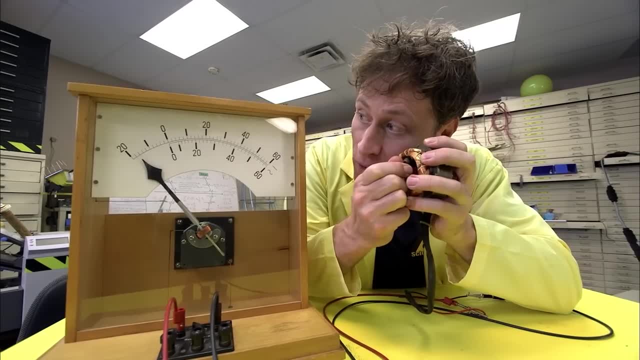 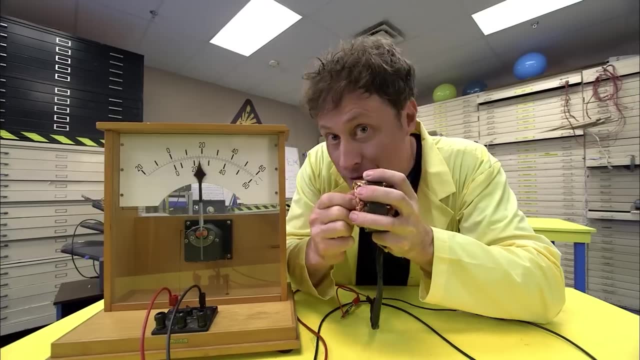 It goes in the other direction A little bit, going this way, and then I take it out A little bit going that way. Positive negative, Positive negative. This kind of current that goes back and forth is called alternating current or AC. 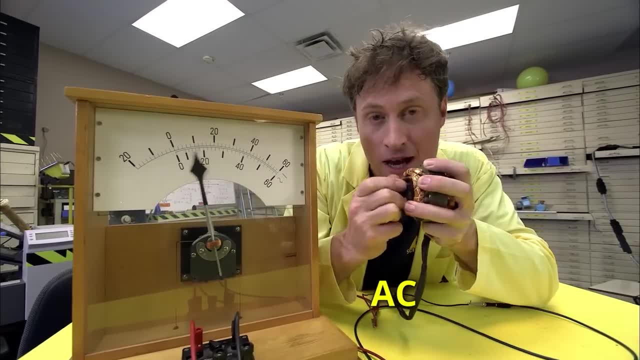 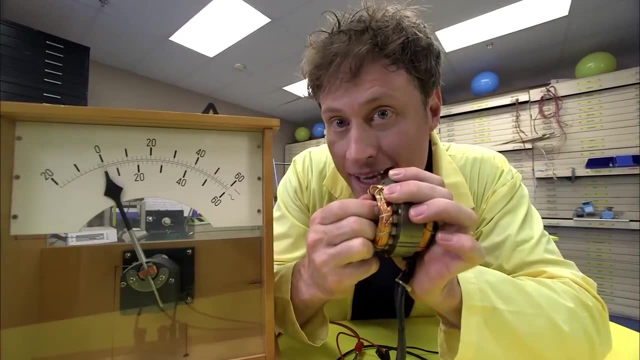 It's the same kind of electricity you have in your house. But here's the cool thing. Watch this: I put the magnet in and I leave it. It goes back to zero. You only get electricity when you move the magnet. All right, so let's create our generator. 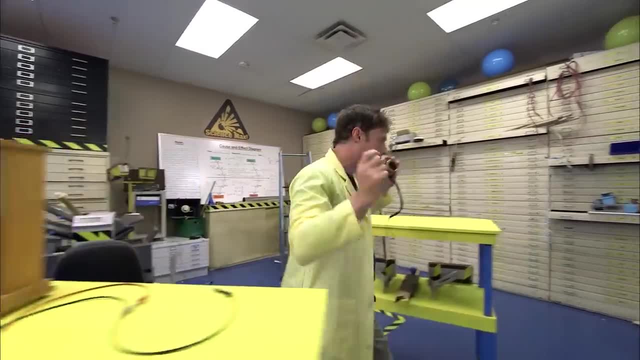 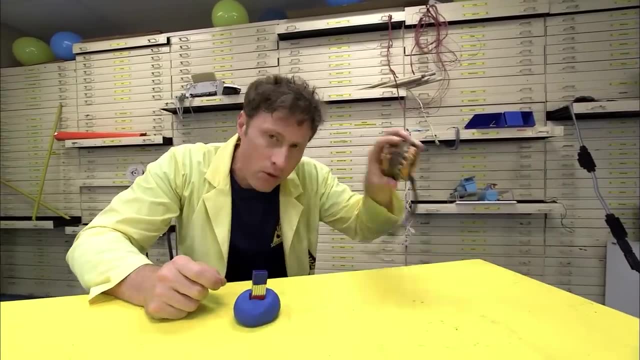 Instead of starting with a copper wire, let's start with a copper coil like this: What if we just had the magnet and we have it staying still like that and we move the conductor past it like spinning? Hmm, It's good but not great. 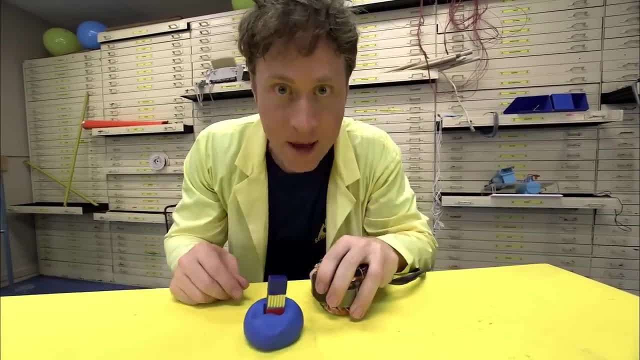 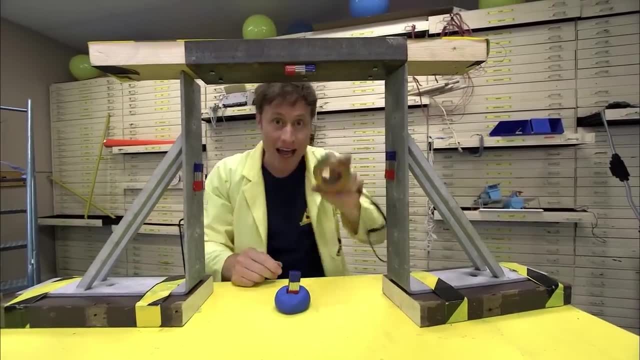 because we're only getting a little bit of electricity as it passes. So let's make it more efficient. Let's put in some more magnets, one on either side and one on the top- And now when we spin it, it goes past all of these magnets. 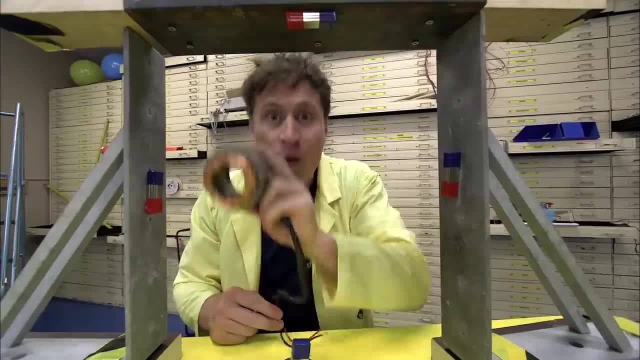 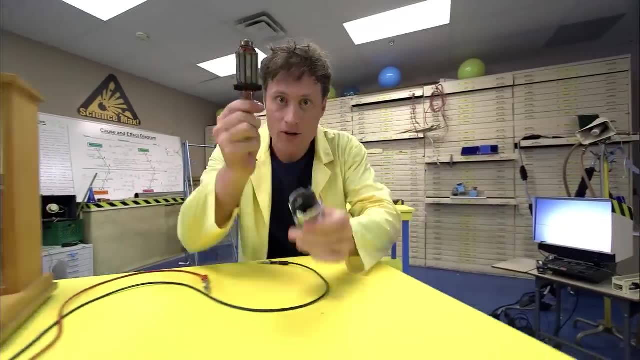 and every time we get a little bit of electric current. Well, this is how a generator works. If you take an electric motor or a generator apart, you can see there's a coil of copper wires on the shaft and it spins around like this. 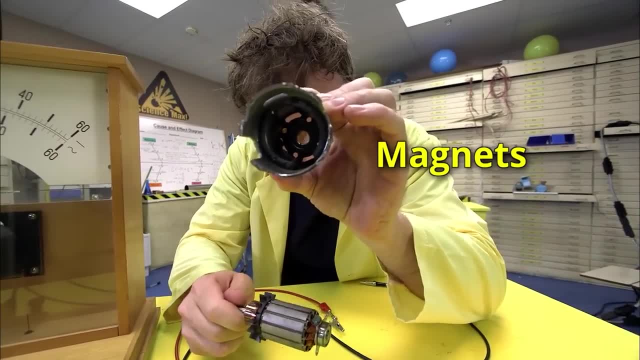 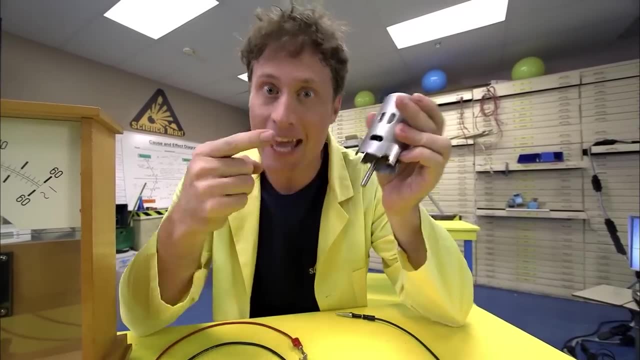 And on the inside there are magnets. So there you go. When you put it together and spin it, you get an electric current. Or if you put an electric current in it, it will spin just like an electric motor. And that is how a generator works. 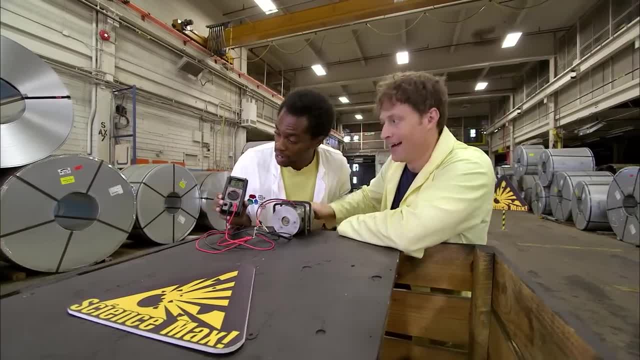 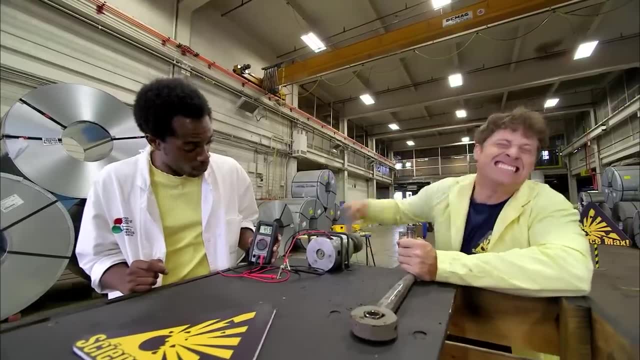 Anthony and I are trying to create as much electricity as we can using just human power, But so far it hasn't been going so well. It all comes down to how fast we can spin the generator. Maybe we could use like some gears or something like that. 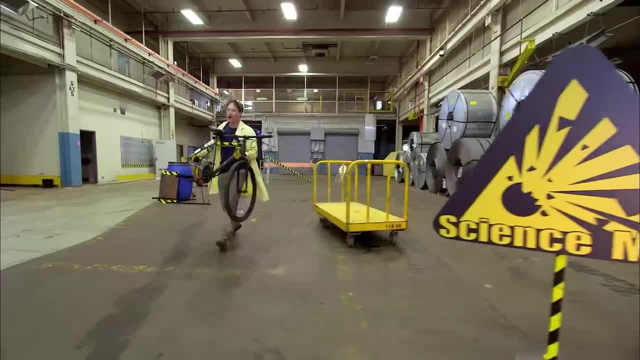 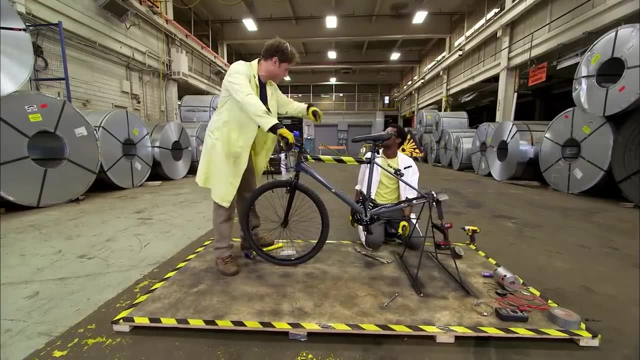 In order to get it spinning really fast, we're going to use a bike. It's just a matter of getting a bike, taking off the wheel, putting it on a stand. It is now a stationary bike. It should be even more stationary once we screw it down. 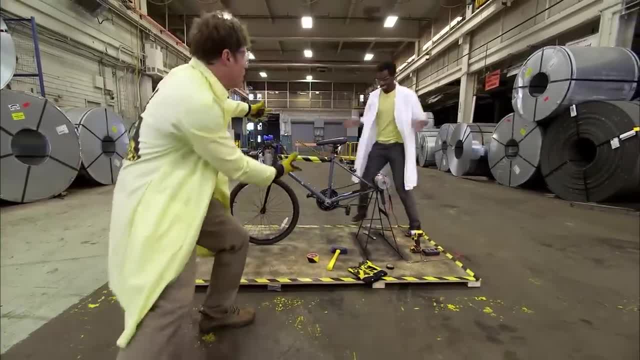 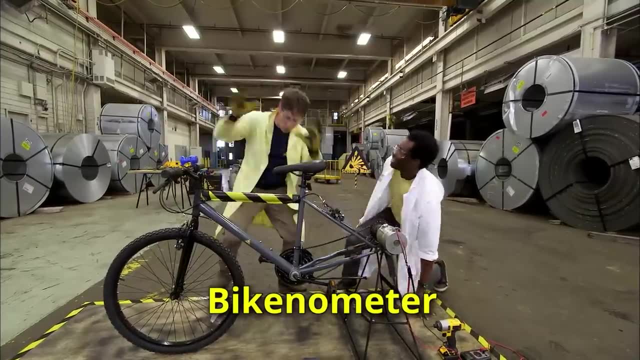 and attaching the generator. All right, The bike generator, Bike-erator- What should we call this thing? Uh, bike-na-nator, Bike-no-mator- I like it So okay, let's go over what we've got here. 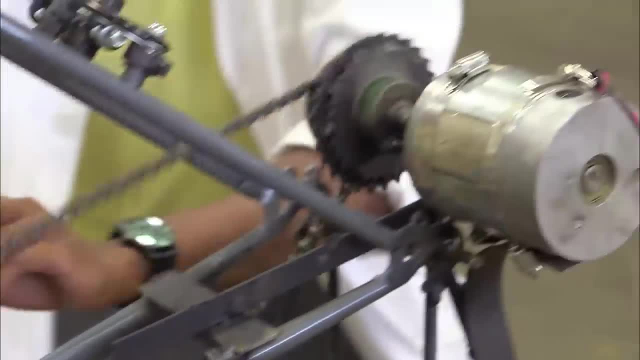 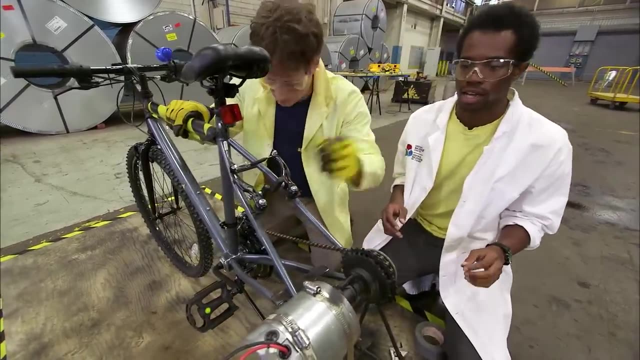 Okay, so we've got two gears: We've got a big one, we've got a small one. We turn our pedals and the big gear turns the small one. So this is the whole point of this build is so that we can get one revolution here. 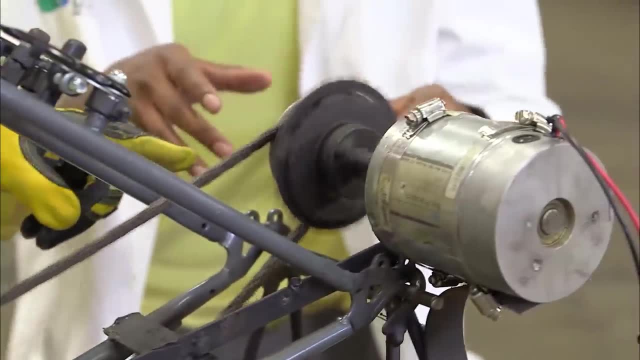 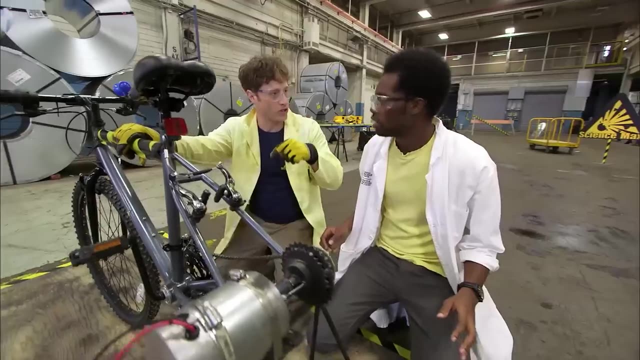 means a whole bunch is spinning there. Exactly Right, right. The more we get here, the more our generator spins and the more electricity we get. We get tons Awesome And uh, obviously using bike, because you're using your legs. 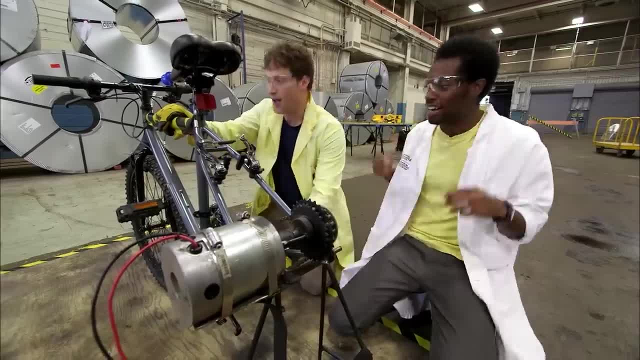 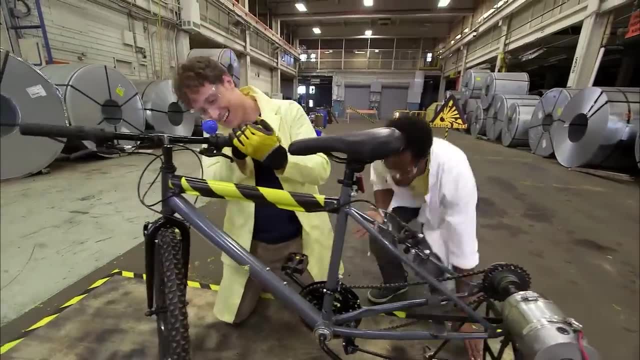 Uh-huh is the strongest muscles in your body. Awesome, Uh-huh. Okay, so now what's with this horn? Oh, that is a loud horn. I know, I know, I tried to warn you. That is great, I love that. 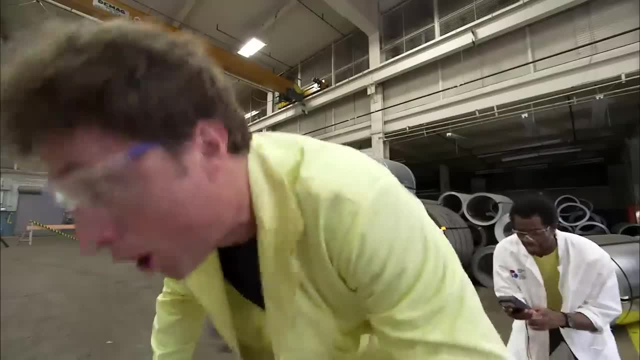 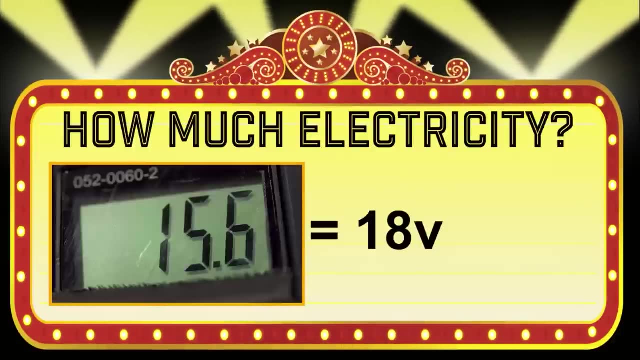 So Anthony and I hop on and give it a pedal. We pedal as hard as we can and we produce a pretty good amount of electricity. How much electricity did they produce? We got up to maybe like 18 there. We did a pretty good job. 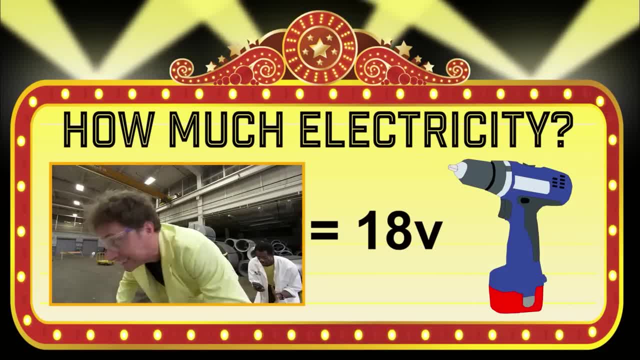 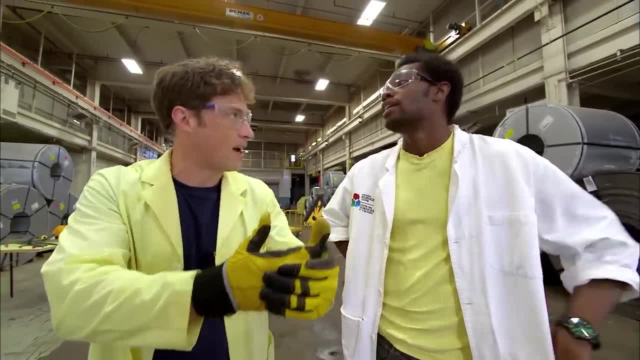 That's enough for a power tool like a drill. It's good. You know what. This works well, I think, for keeping a good number for a long period of time. Yeah, So we can get up to like 18, 20.. 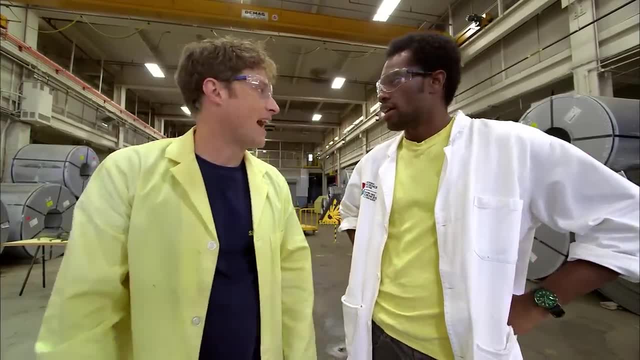 Mm-hmm, But it doesn't. We can't really get any higher than that. Yeah, you know, what we need is like one really hard pull like all of a sudden. That way you can get like a spike. 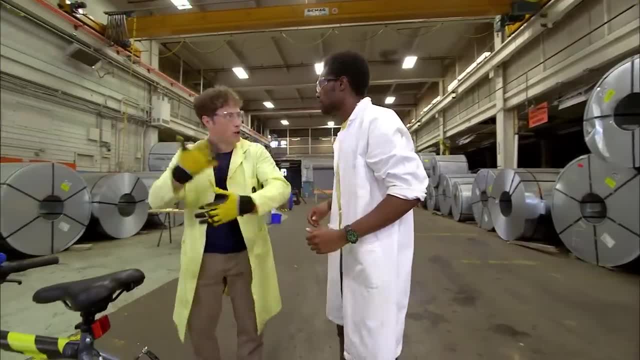 Yeah, you're right. So it's like, instead of putting all that effort into going for a long time, you put all the effort into one quick motion, Exactly. Yeah, good idea. So you wrap a rope around here and then you just pull it. 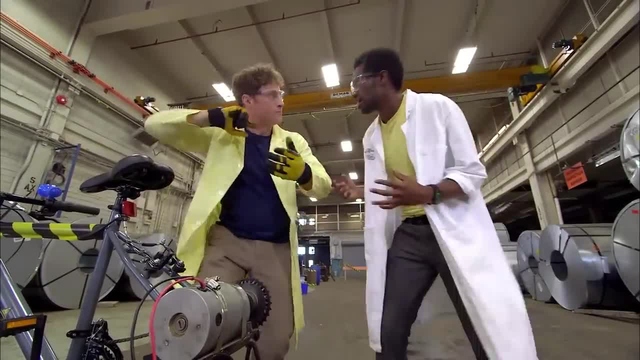 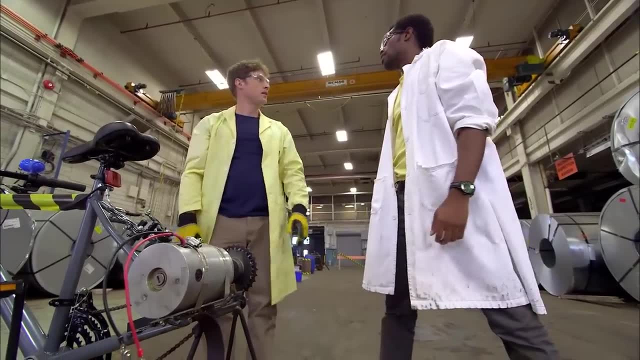 Exactly exactly, And that would be a really fast motion, Uh-huh, Spin it really quick and get a very high number, High spike, exactly Okay, You know we're gonna have to take the bike apart, though, Okay well, 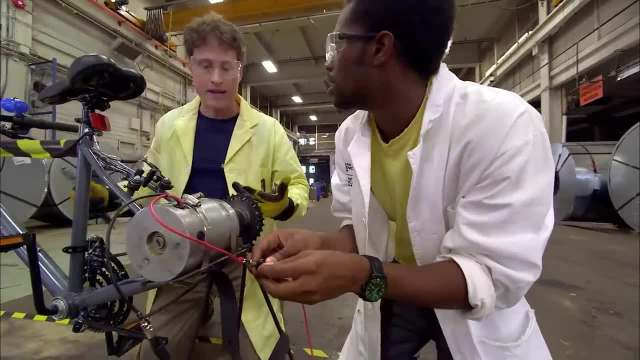 Well, it's science, Okay cool, So I'll just get. Oh, you know what? We actually don't have to take the whole bike apart, We just have to take the generator off. Oh right, Okay, hang on a sec. 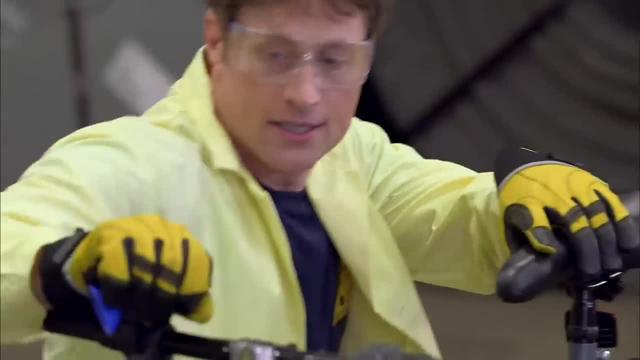 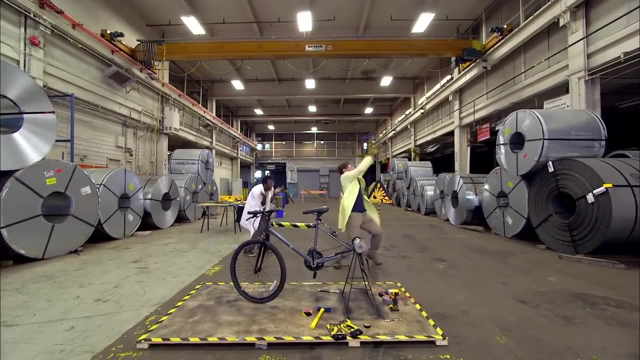 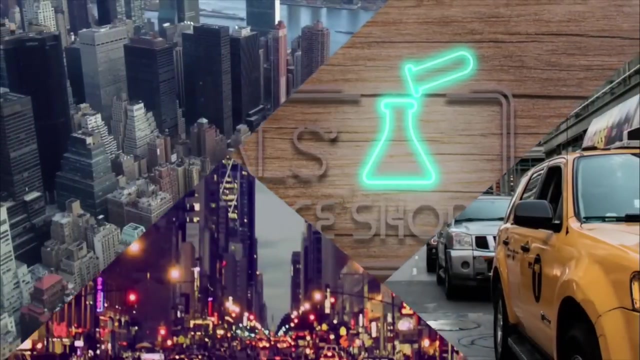 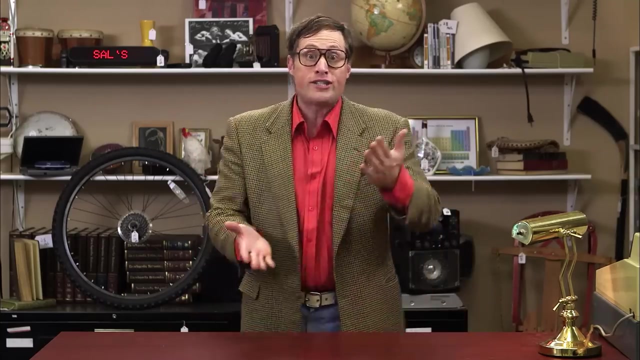 I got it. I need to attach the horn to the next thing too. What are you? No, Turn it off. It's so loud. So you want to generate some electricity. But what do you choose to generate that electricity? Hydro. 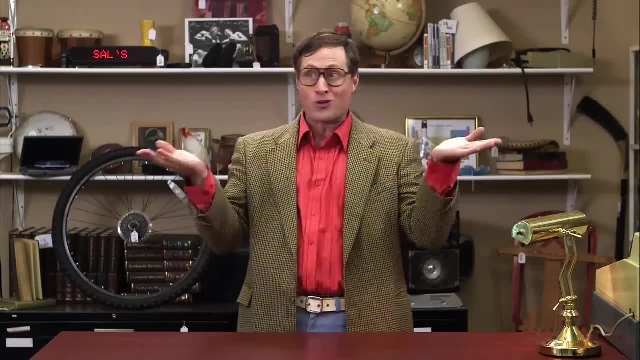 Nuclear, Coal, Solar. Who knows? I do, I know, And soon so will you. In order to generate electricity, you need to turn the generator. Turn the generator. One of the most common ways to turn the generator is to use one of these. 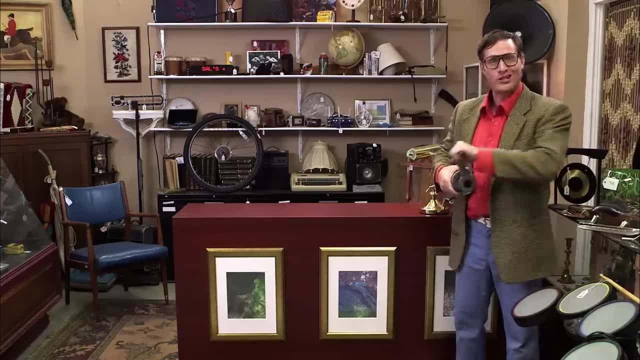 It's a steam engine. Usually they're a lot bigger. You see, you heat the water to boil it and turn it to steam, which works a piston which turns the generator. Huh, Pretty amazing, right, But what it really does is it turns the generator. 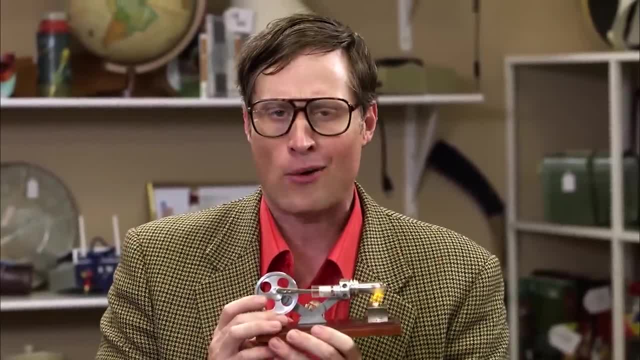 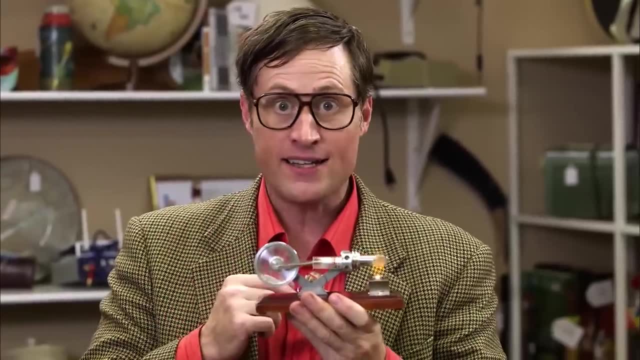 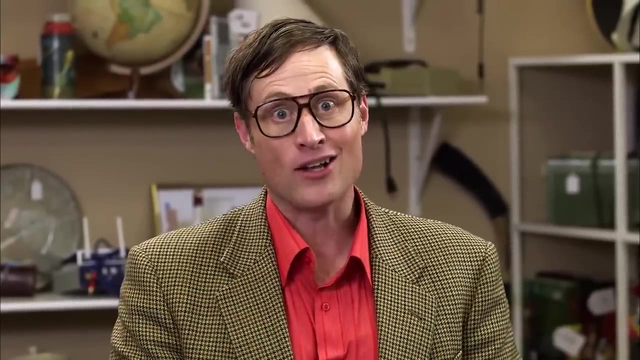 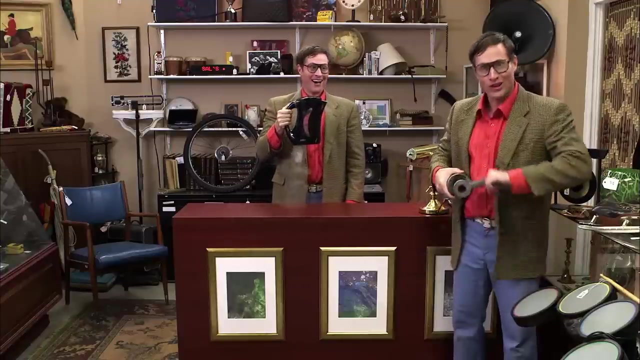 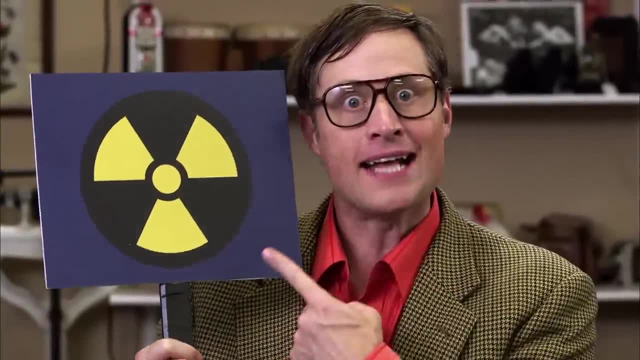 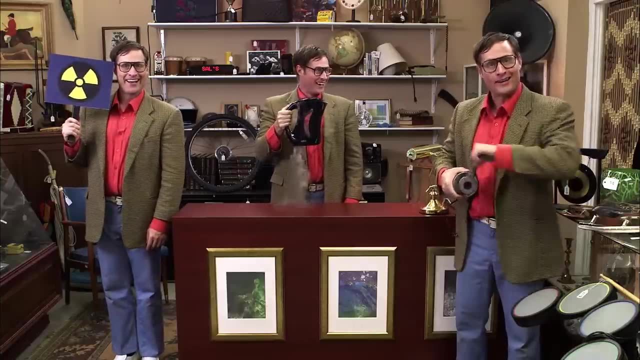 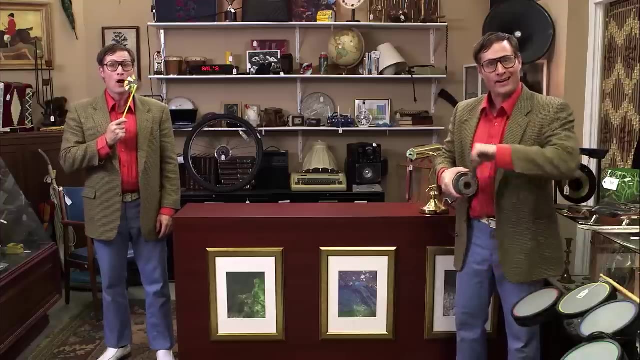 To Boil Water. Nope, it creates heat which you use to boil water, to make steam, to turn the generator. Wind power- We don't even need heat for that, Just use the wind to spin the fan to turn the generator. 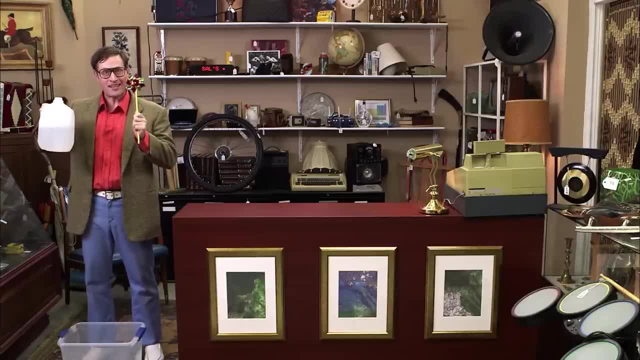 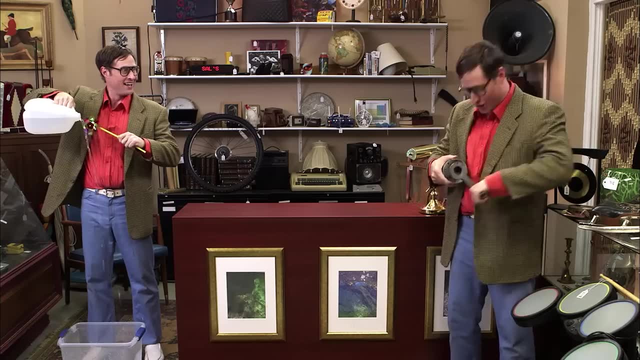 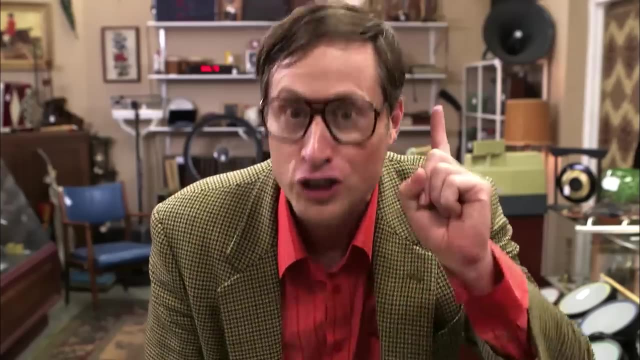 Hydropower Just pour water across something that spins to turn the generator. No matter what, making electricity always comes down to turning the generator. It's always yada, yada, yada, yada. turn the generator, Except for solar. 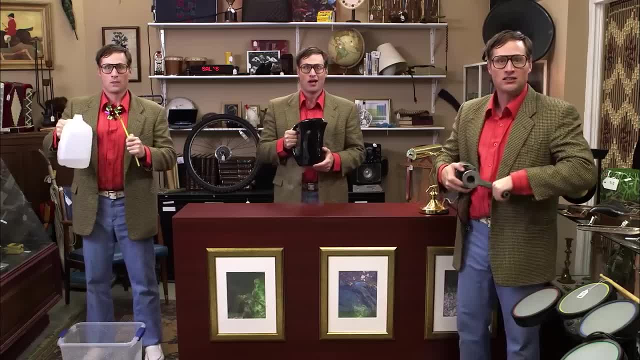 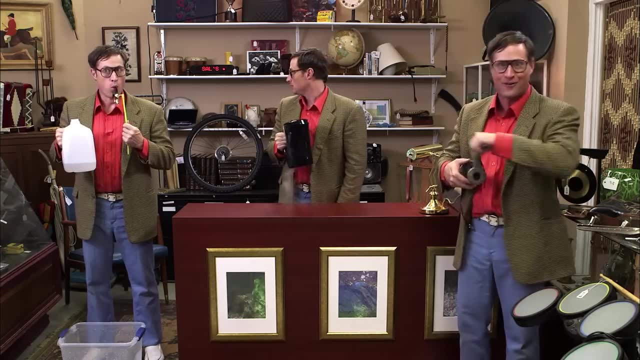 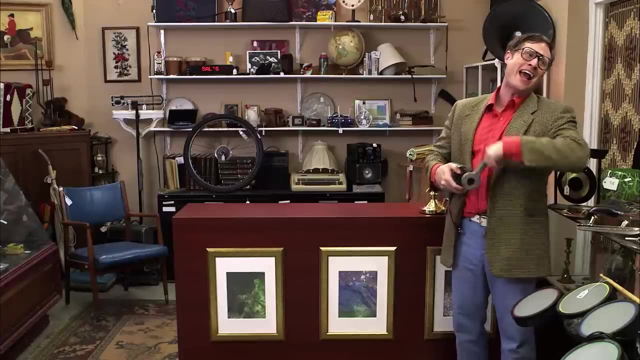 Solar does not work like that, But other than that, it's always yada, yada, yada yada to turn the generator, And now you know your electricity generation. Hey, Ramona, you want to come and give me a hand over here? 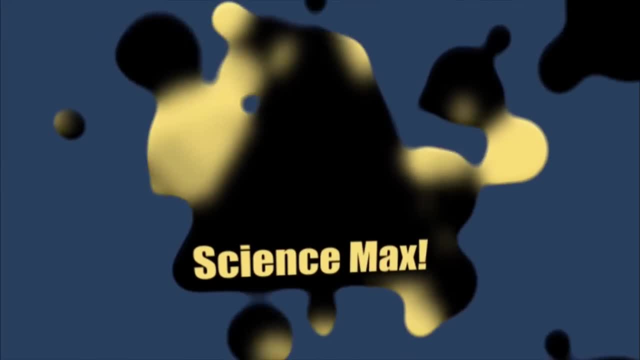 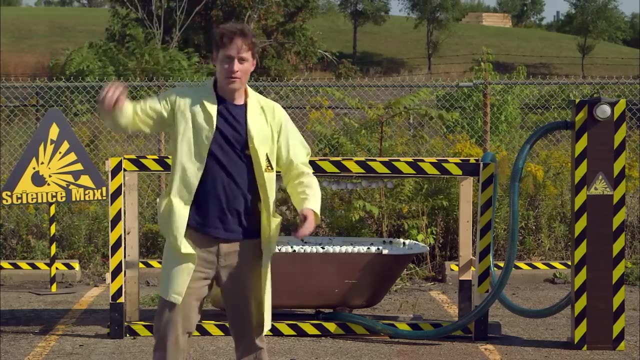 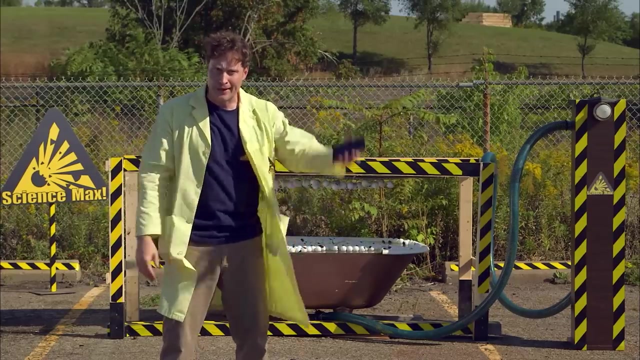 My arm is getting tired. Whew, it is hot out here. Oh, in order to generate electricity, you need to spin a generator. Most forms of electricity generation work like that, but not solar. Solar panels like this one generate electricity from the sun's energy. 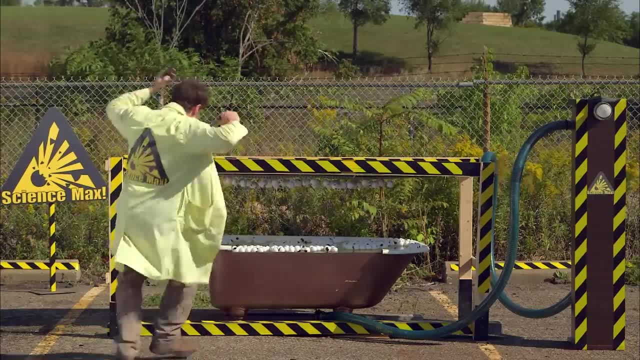 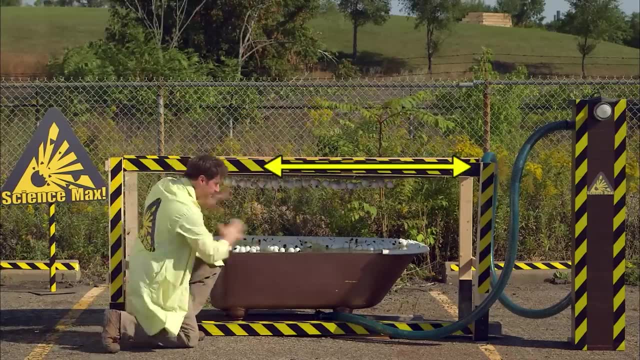 So how do they do it? Well, this is a solar panel. Okay, it's not really a solar panel, I just sort of put this together, but it works the same way. There are two plates. There are two plates. There are two plates. 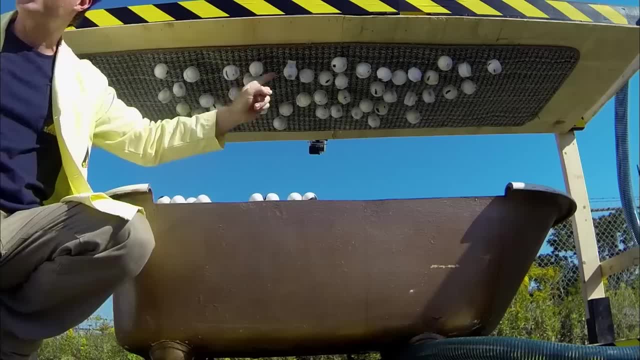 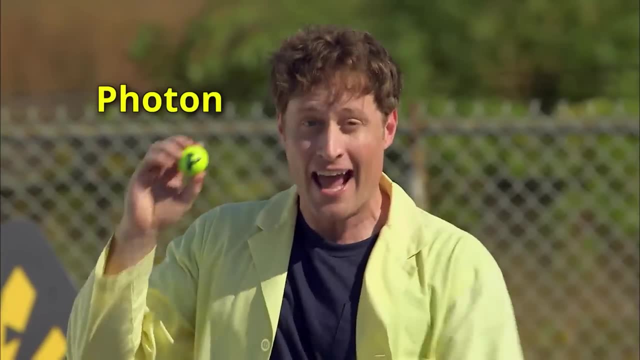 And on these plates are electrons. I've got golf ball electrons up here, ping-pong ball electrons down here, but they're all the same thing. Now, this happy little fellow is a photon energy from the sun in handy-dandy particle form. 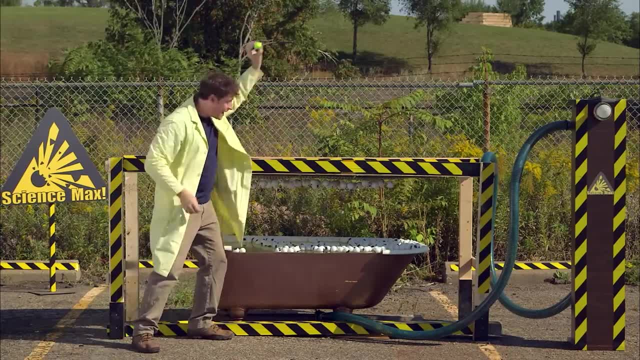 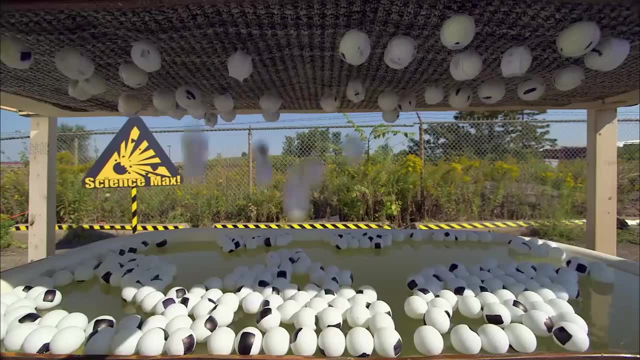 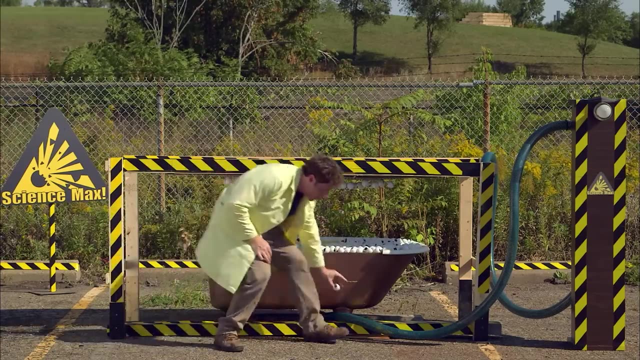 What happens is photons come from the sun and hit the top plate and knock some electrons from one side to the other like this, And that knocks over some electrons. Now these atoms, these extra electrons, travel up a wire in the form of electricity. 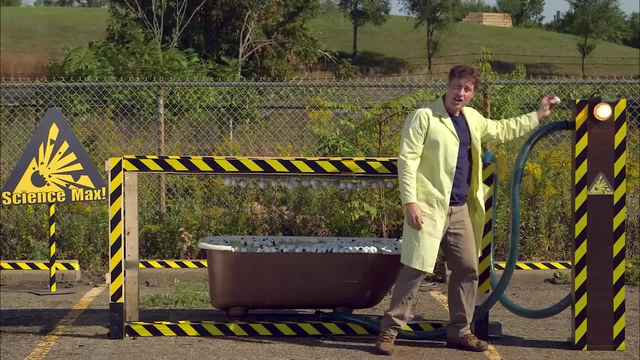 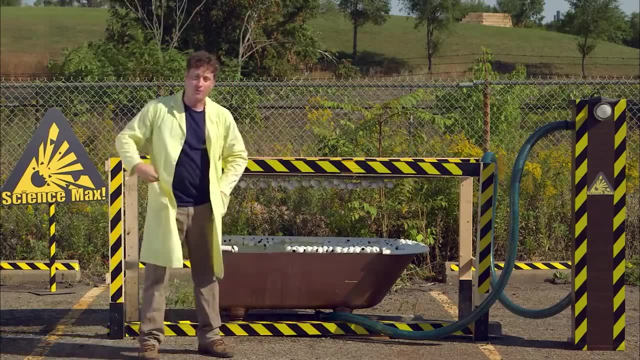 and we can use them to do work for us. Then they change to the other charge, go back and we start the process all over again. That is how solar panels work, But remember, it only works when there's sun and photons. 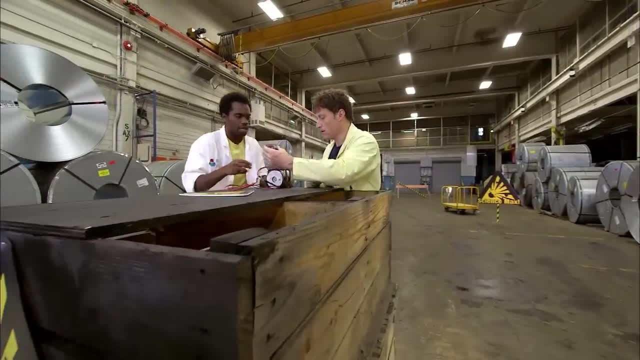 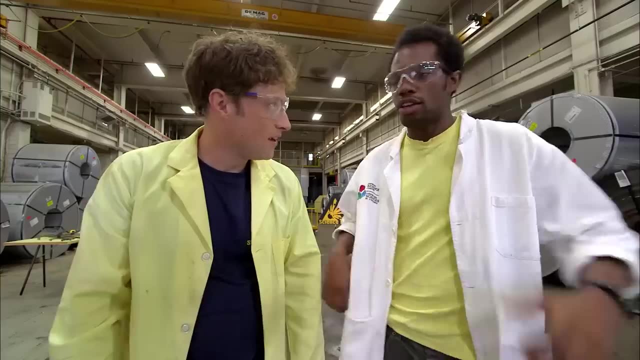 Anthony and I are trying to generate electricity using human power. Spinning the generator didn't work too well, but we found if we used some gears like those on a bike, it worked better. You know, what we need is like: 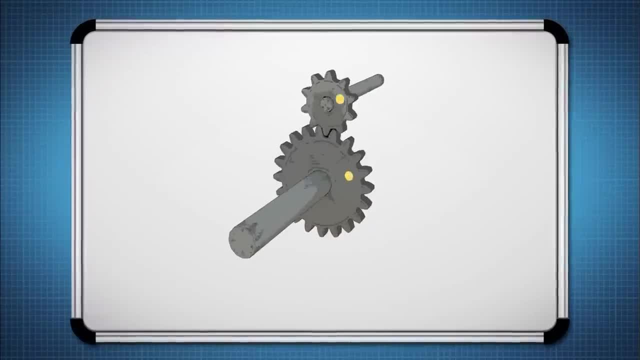 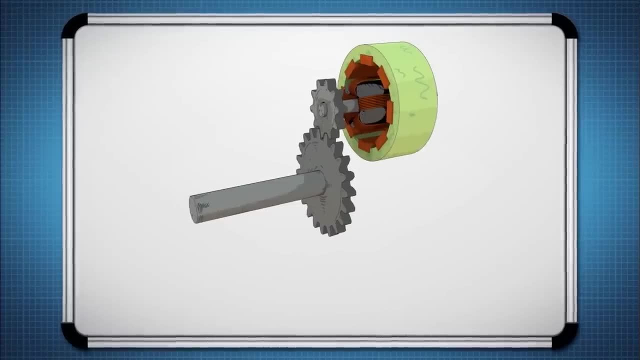 one really hard pull like all of a sudden Using gears is a great way to get work done. The good news is there are generators with gears already in them. That means if we can turn the spindle once, the gears inside will spin the coil a lot of times. 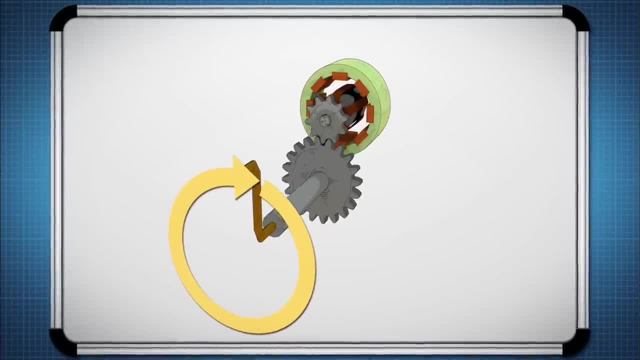 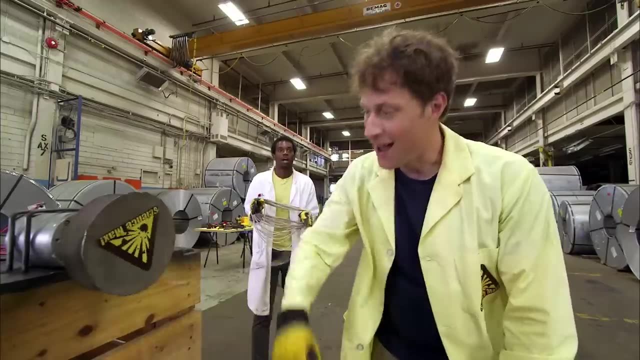 The only downside: Turning the spindle gets harder the higher it goes. So we have to fire the gear. Anthony and I attach a spindle and then we wind up the rope, which takes a while. Okay, so the plan is. it's on a big spool now. 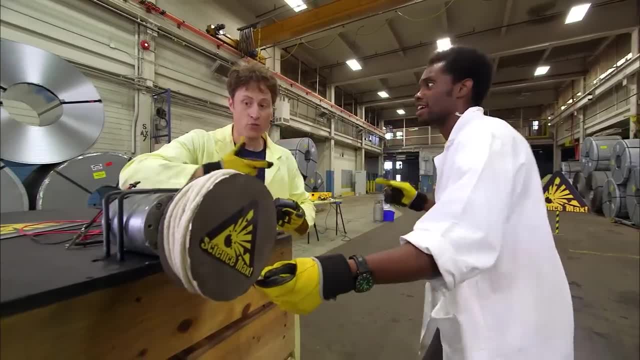 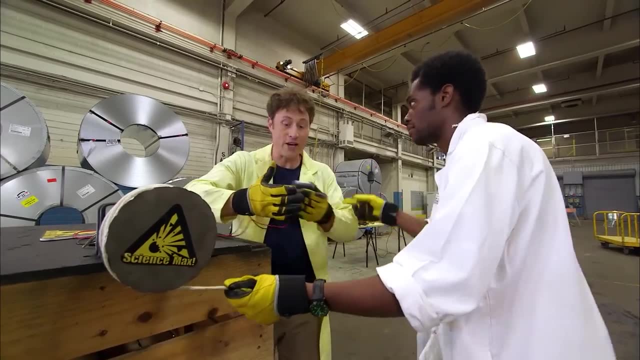 Yeah, And you just run as fast as you can, Got it, And we'll hopefully get as many revolutions as we can, depending on how fast your top speed is. Okay, Sounds good. Sounds good. I can be pretty quick. Okay, good, All right. 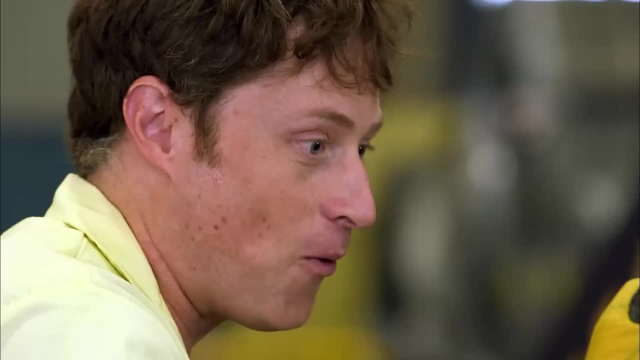 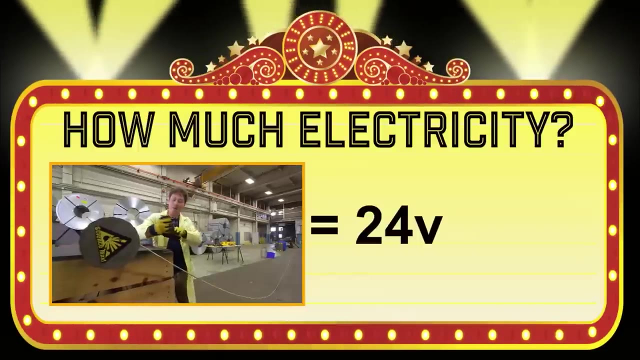 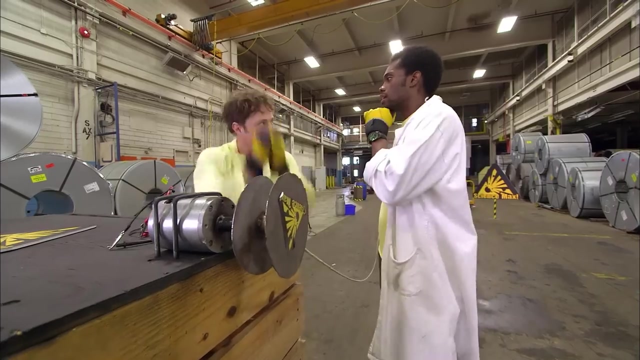 Ready On your mark? Uh-huh, Get set. Uh-huh. How much electricity did they create? 24 volts, Actually, not bad. That's enough to power their own personal scooter. Not too shabby boys, We need like a hard pull all at once. 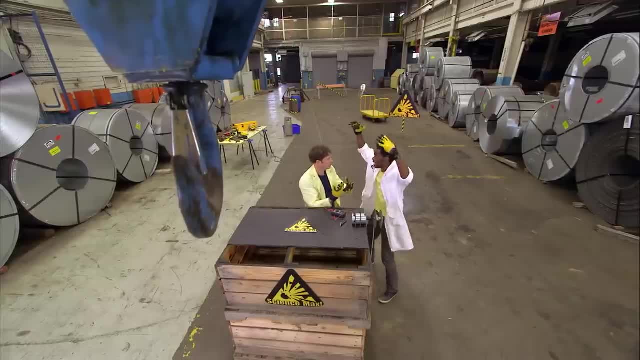 Yeah, From something like really big. What if we could get like really high? Okay, Like up there, Could we attach the generator up there. You could jump down from there And I would hang on the rope. 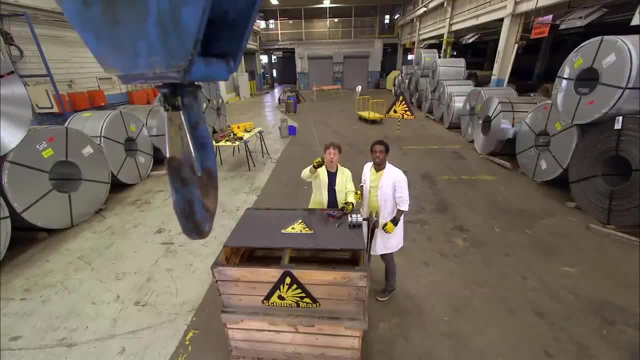 Yeah, Yeah, that's good, but I don't want to jump from up there. Oh, what if we put a pulley up there? That would work, And then the rope goes through the pulley and then back down and then I jump from somewhere much safer. 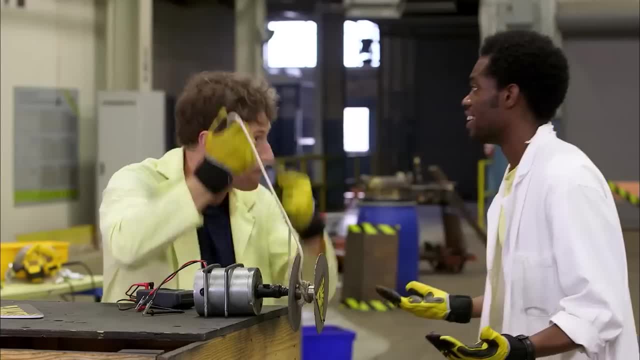 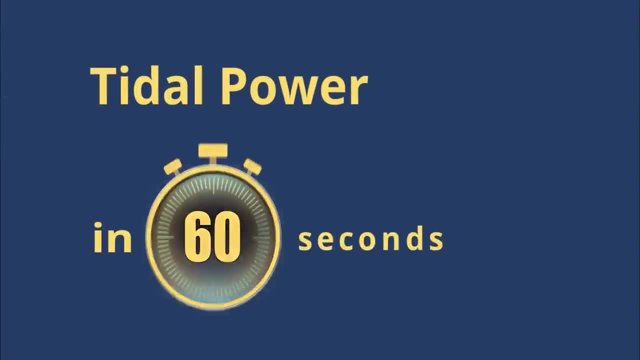 like just on top of here onto a crash mat or something. That sounds great, And that's my full body weight on the rope. That sounds great. All right, high-fives, Yeah, Tidal Power in 60 Seconds. By now you know that in order to create electricity. 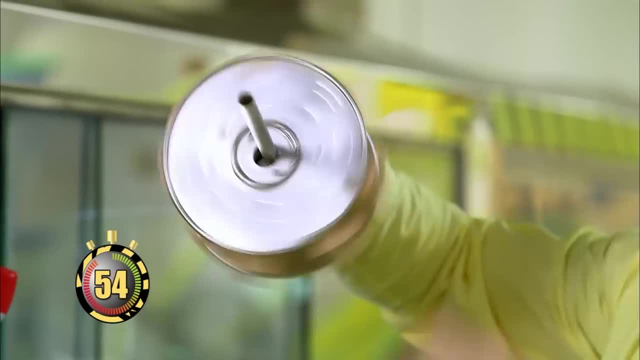 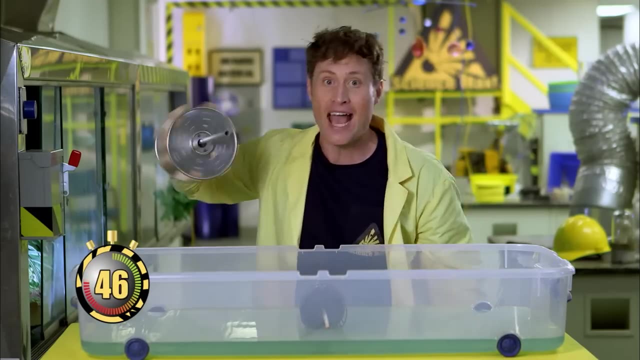 you need to spin a generator. Scientists and engineers are always coming up with lots of new ways to use natural forces of the Earth to spin a generator. To spin a generator and create electricity- One of those natural forces. One of those natural forces is the power of the tides. 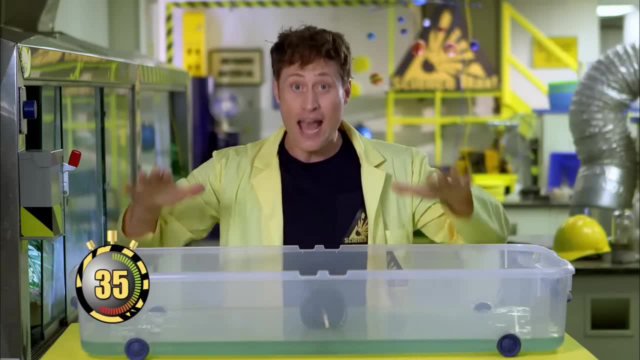 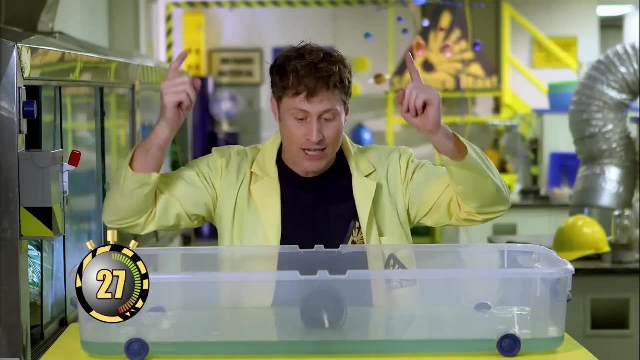 You see, the water in the oceans doesn't stay still. Every few hours the water or the tide goes out And then a few hours later it comes back in. So if you attach a paddle wheel in the water and attach that to a generator, 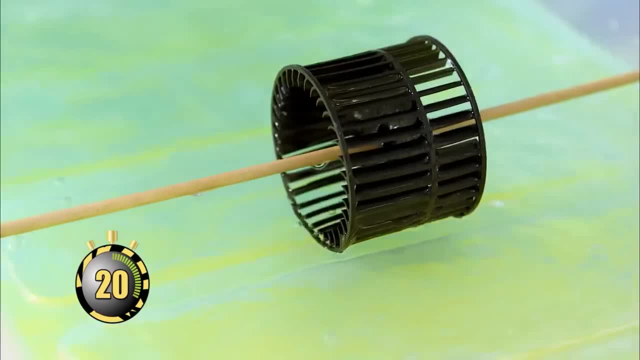 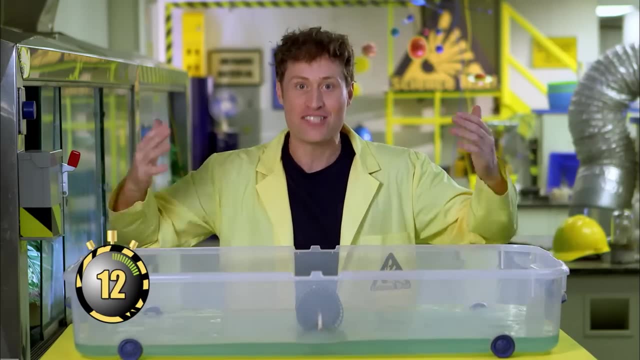 when the tide goes out, it creates electricity. When the tide comes back in, it creates electricity. That is how you create electricity: using the power of the tides. It's water power. In fact, hydroelectricity is also using water power. 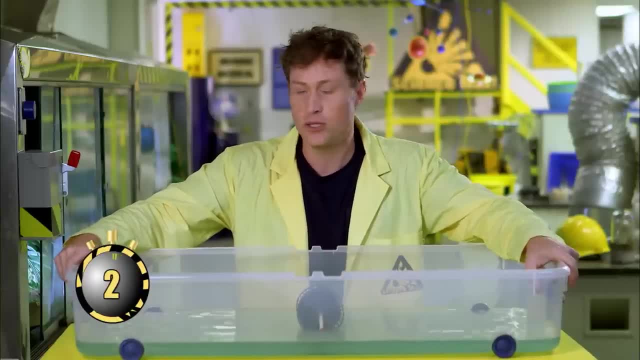 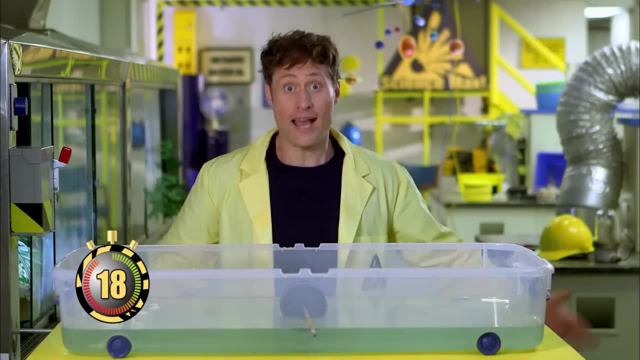 Do we have time to talk about hydroelectricity? We don't have time, We don't. Okay, come back, Come back. Hydroelectric Power in 20 Seconds. 20 seconds, Uh okay. Hydroelectricity comes from water. 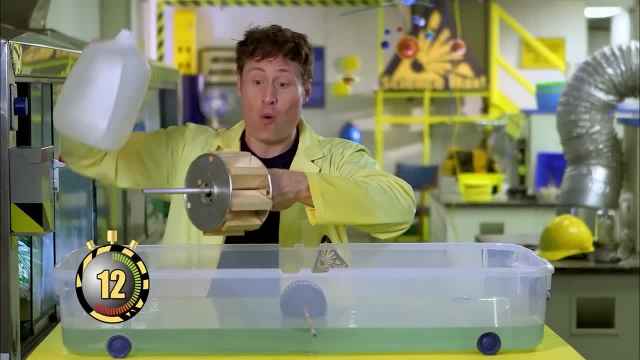 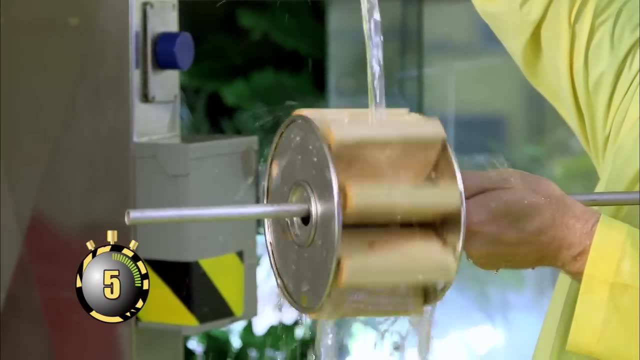 Hydro means water, So all you have to do is find a place where water pours down from a height And you can put a generator in there and, ta-da, you're creating electricity with the power of hydro. Ha-ha-ha-ha. 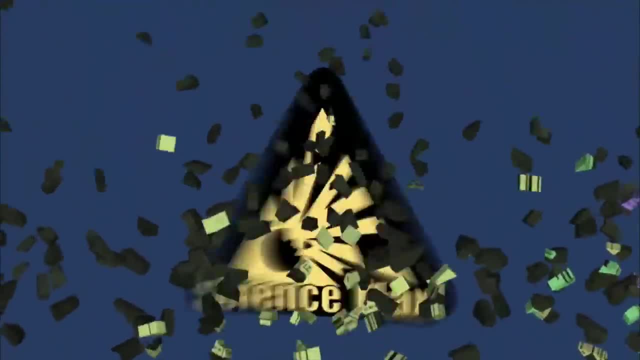 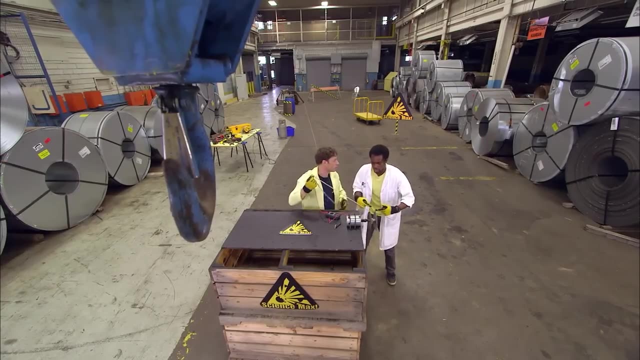 Ha-ha-ha, I did it. Anthony and I have pulled and pedaled and now we're going to hang onto the rope and use our whole body weight to spin the generator as fast as possible. Okay, Okay, Crash mat. 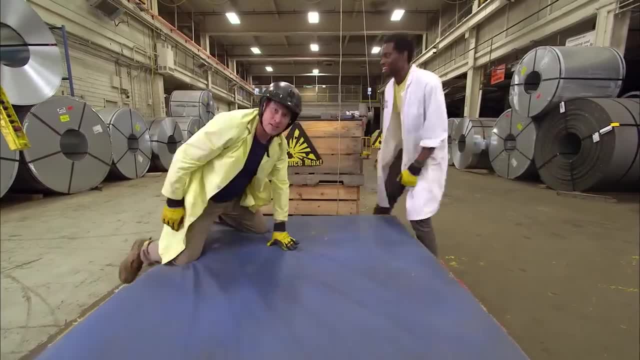 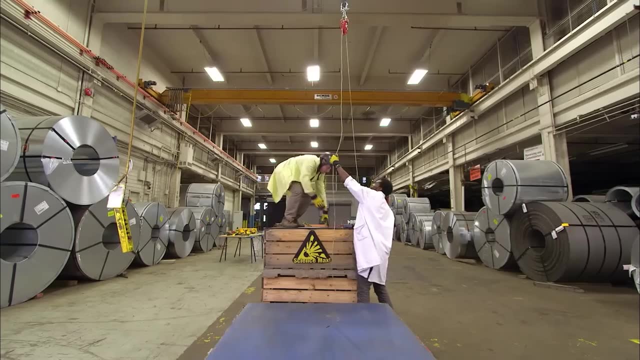 Uh-huh, Let me test it out. Looks good. Yep, it's good for crashing, So I go up here. Uh-huh, Okay, I go up here. Climb on up, We'll get you the rope. Got your helmet for safety. 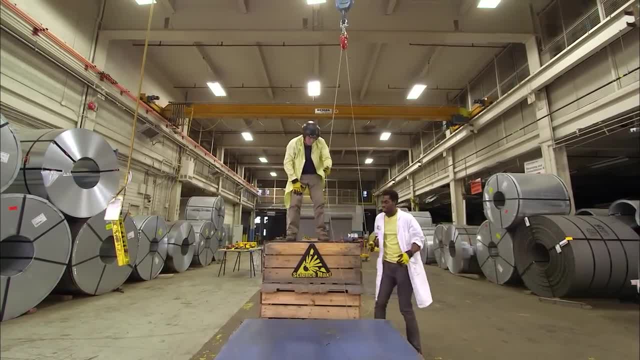 Helmet for safety, Crash mat for safety. So we have the rope and it goes up through that pulley and then back down to our generator, Right with a spindle on it, And as I fall the spindle will turn Exactly. 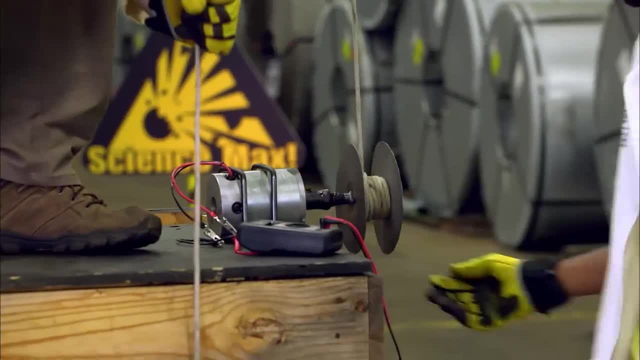 And hopefully the speed of me falling and holding it and yanking it down as hard as I can will be the biggest spike of electricity yet. That's right, We're going to have to do it. We're going to have to do it. 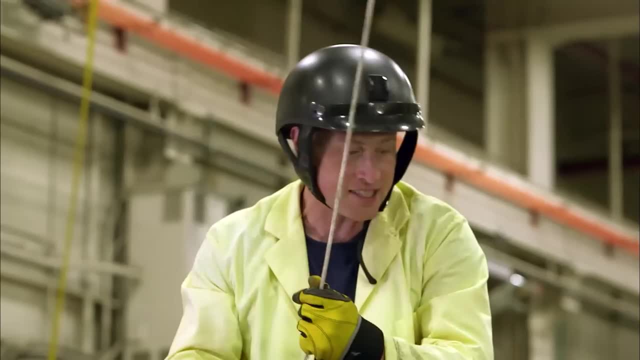 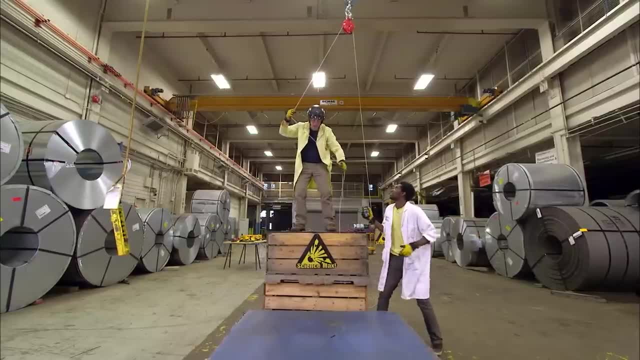 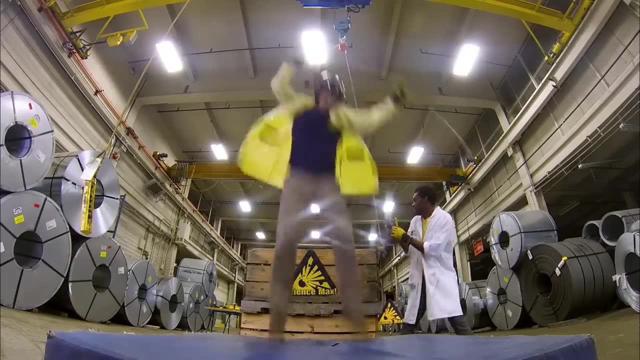 on our multimeter here. Okay, Okay, Ready, You ready, Yeah, Here we go. Three, two, one. I jump down and my whole body weight pulls on the line. Oh, that was awesome. That was like our biggest spike ever. 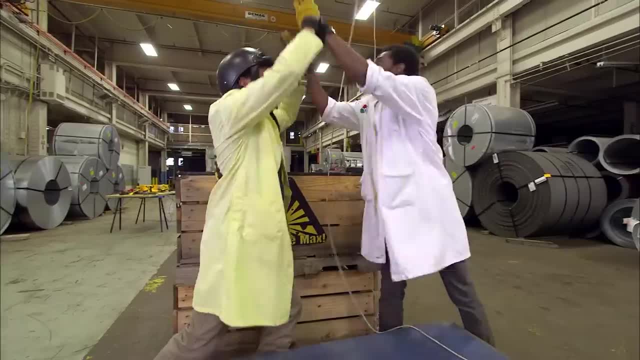 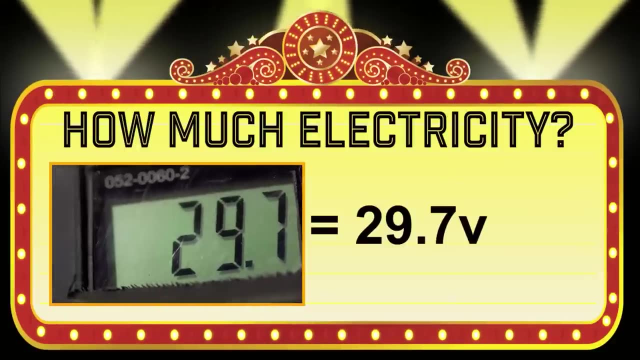 That was amazing. All right, High five, Yeah, Biggest spike ever. Is it enough to power my house? Nope, How much electricity did Phil generate? Almost 30 volts. How much does he need to power his house? Well, 120 volts. 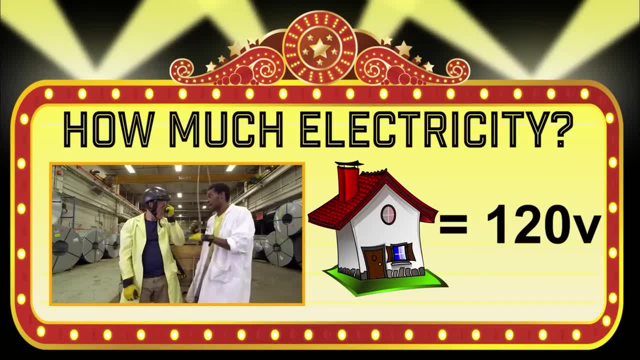 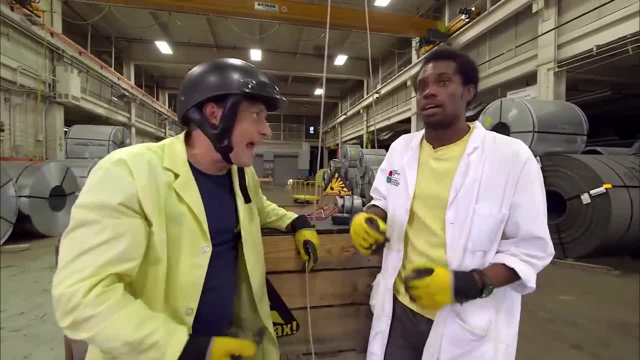 He's still off by quite a bit. Well, we've learned something: nuclear, wind, hydro, solar, natural gas, coal power- It's all great ways to generate electricity, Yeah, And human power not so much. Not as good. 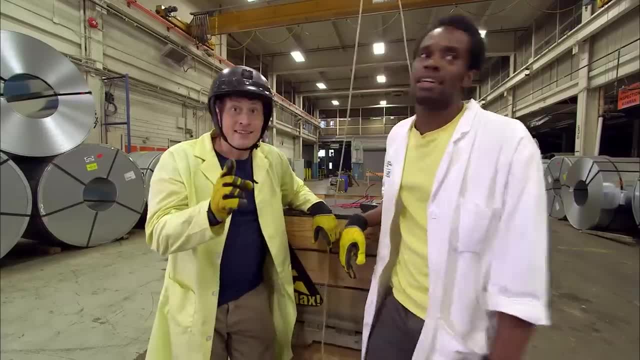 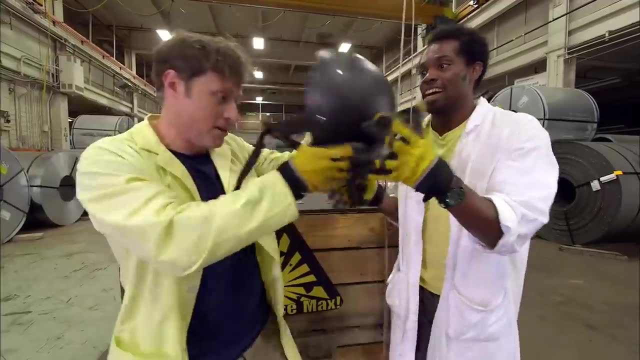 But human power is more fun. Yeah, way more fun. Yeah, So your turn. Yes, Okay, okay, You take the helmet and I'll take the multimeter. Okay, And then we'll go and we'll do it again. 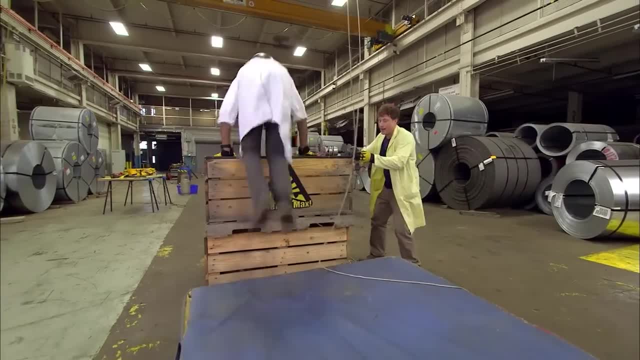 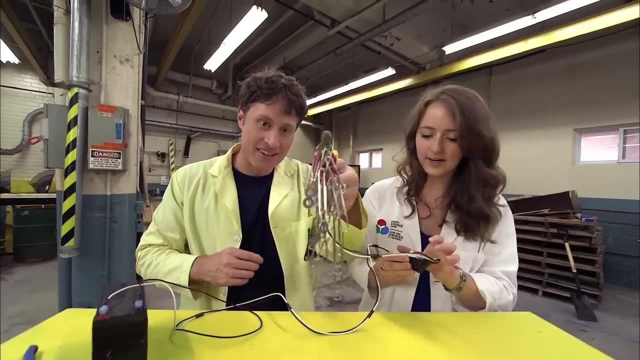 Okay, Okay, Wait, I gotta wind it up. Science Max, Electromagnets are magnets. you can turn on or off when you want. We build our own electromagnet and see just how powerful we can make it. It held 100 kilograms. 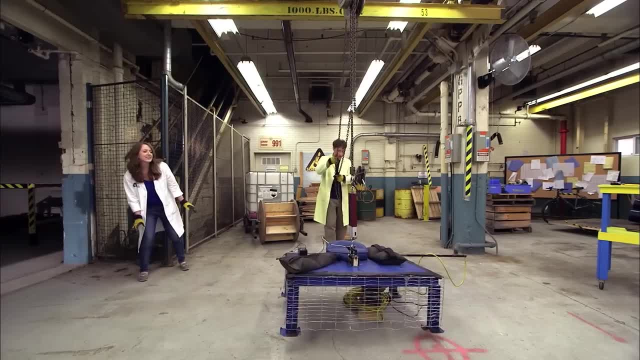 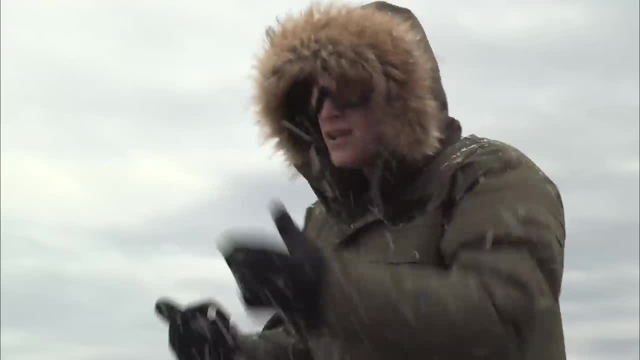 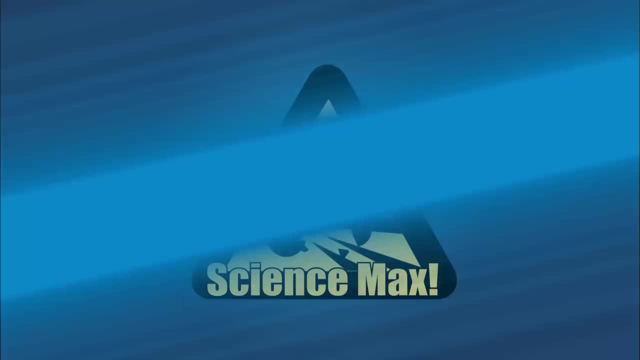 Plus ferrofluid wizards, and I tried to get to the North Pole using a compass. Now that I'm here, I realize it's really difficult. All on this episode of Science: Max Experiments at Large Greetings- Science Maximites. 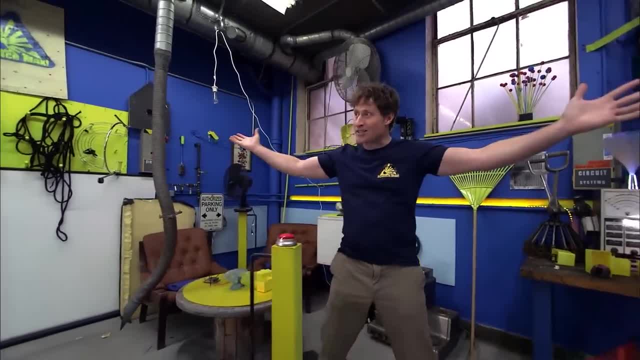 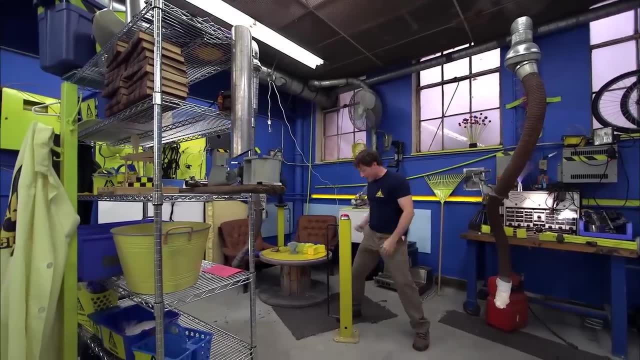 My name is Phil and welcome to Science Max Experiments at Large. At this very moment, half the lab is being held together with the power of electromagnets- Magnet one turning off. Electromagnets are a really cool and powerful way to interact. 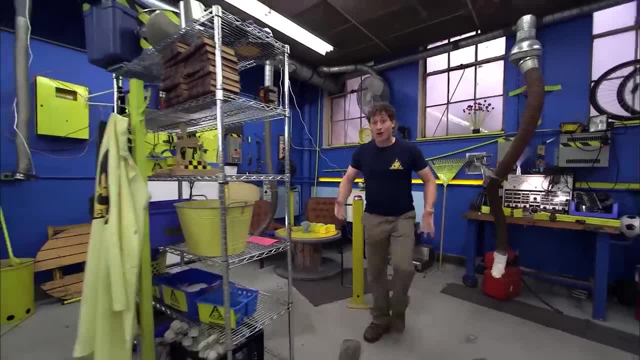 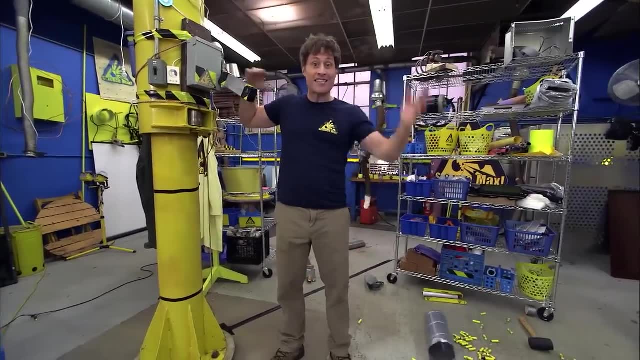 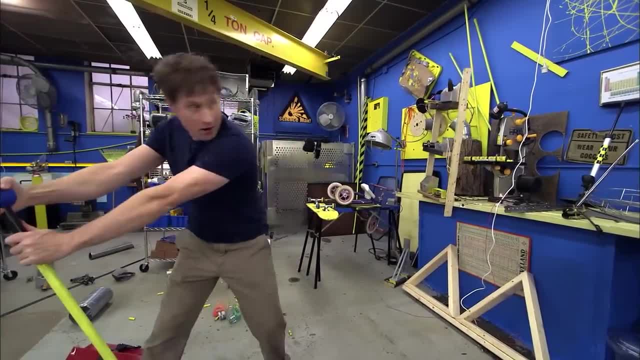 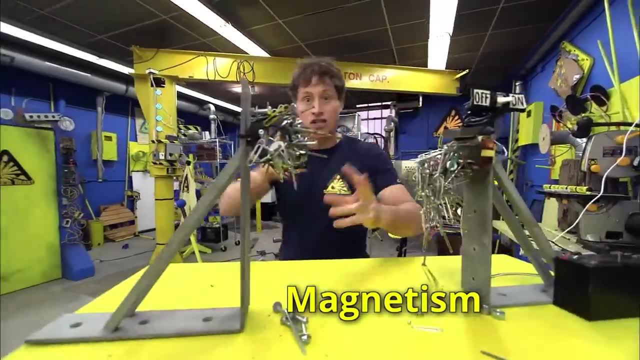 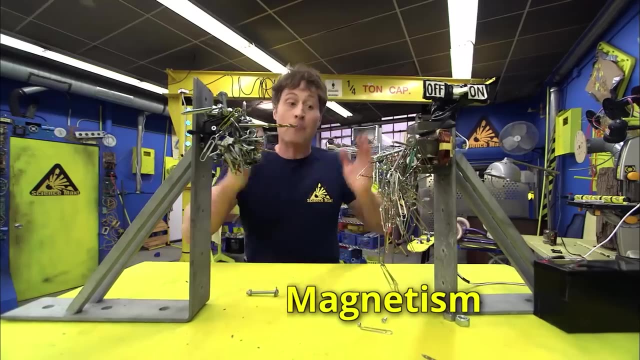 Let's get started. Let's make them work or not work. Magnetism is an invisible force that has to do with the magnetic fields created by magnets. that lets them attract things that are metal or each other. But electromagnetism is a little different. 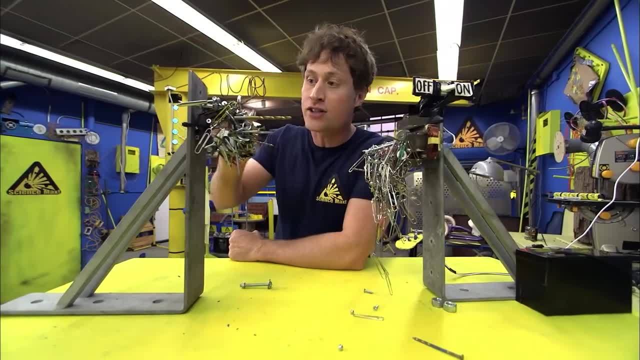 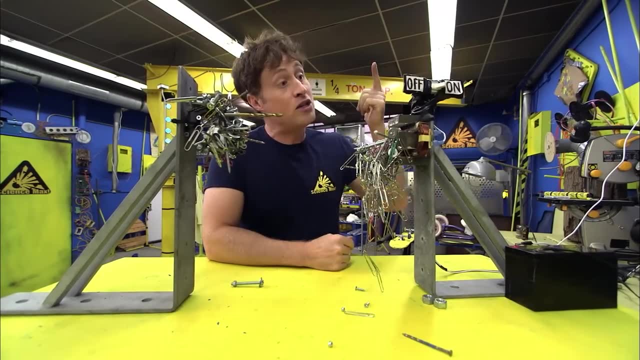 You see, magnets are magnets all the time. It's because of what they're made out of. Electromagnets are only a magnet when you have an electric current going through them, which means you can turn them on or off. Today, 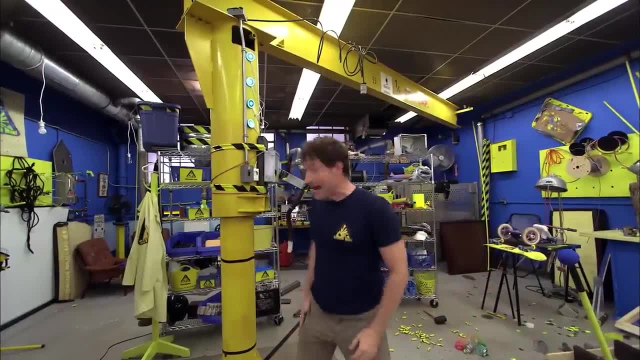 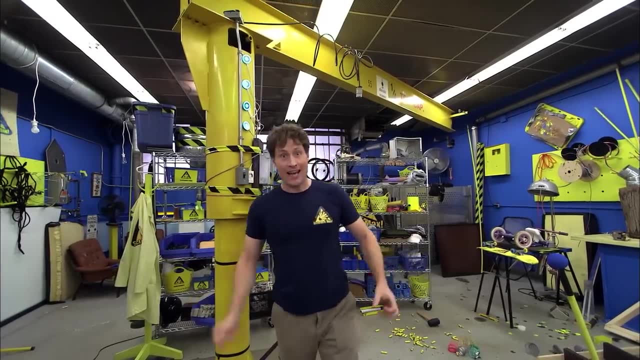 we're going to be building an electromagnet. Oh, that was, that was the wrong switch. Anyway, like I was saying, today we're going to be building an electromagnet. You need a bunch of copper wire, a very large nail or something metal. 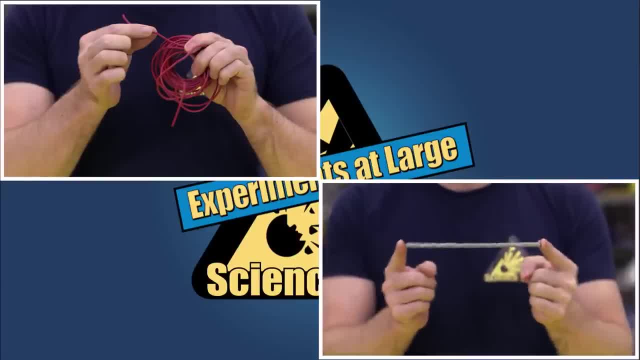 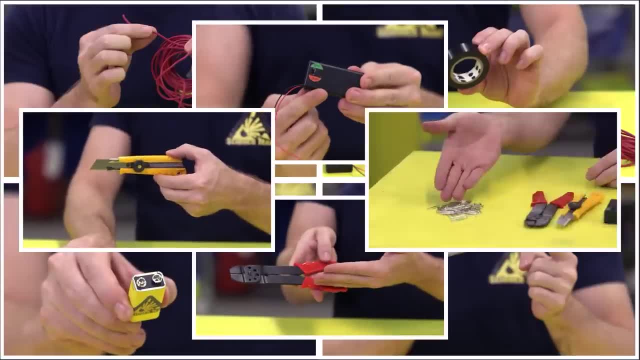 to become your electromagnet electrical tape, a battery, an on-off switch, wire strippers or a craft knife and the help of an adult and, finally, something to magnetize, like these paper clips, And remember all of the steps. 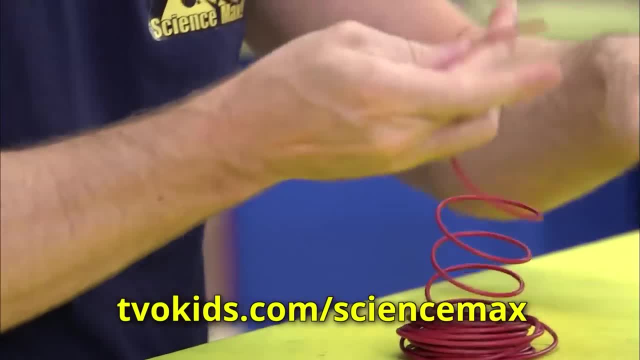 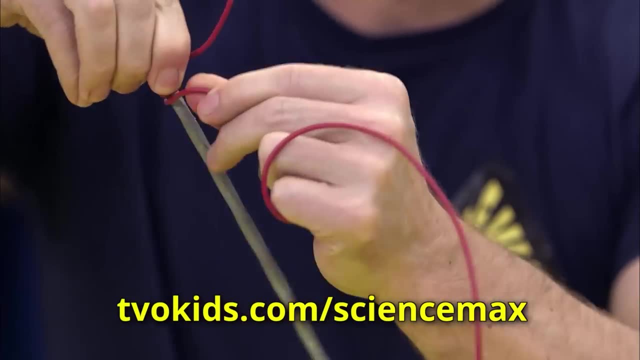 for this experiment are on the website. To begin, take the copper wire and start at the top of the nail. Leave a little bit of wire sticking out, then carefully start to wrap the wire around the nail. Don't go all the way to the end. 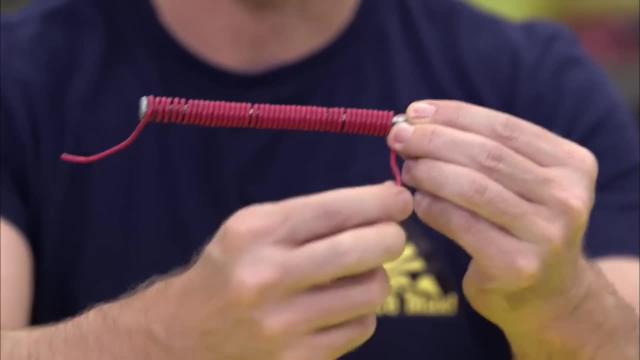 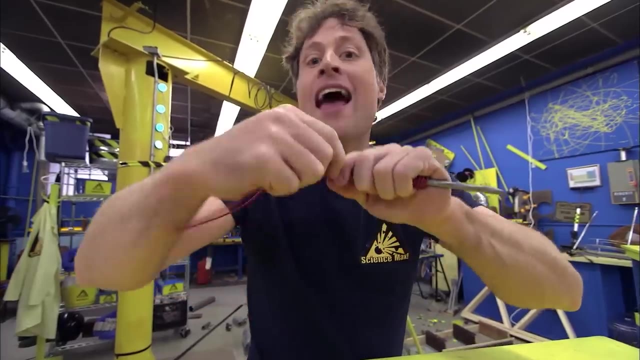 because you need some metal to turn into the magnet. Instead, when you want to start again, run the wire straight back to the top and start wrapping again in the same direction, And keep, wrapping, and wrapping until you get to this. Now I've used 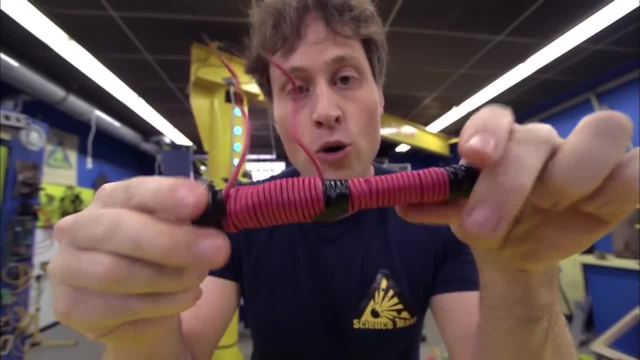 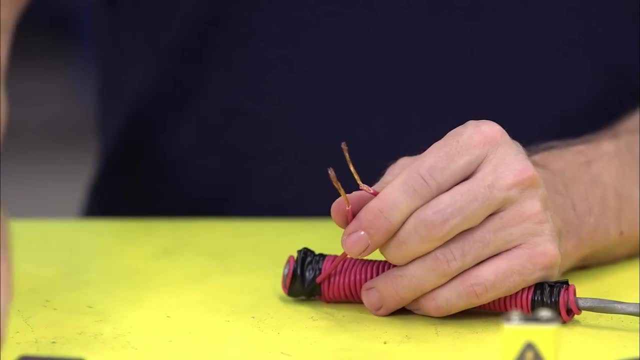 some electrical tape here, here and here to hold it all together. Using your wire strippers or a craft knife and the help of an adult, remove the plastic coating from the ends of the wires. Attach these wires to the wires from the on-off switch. 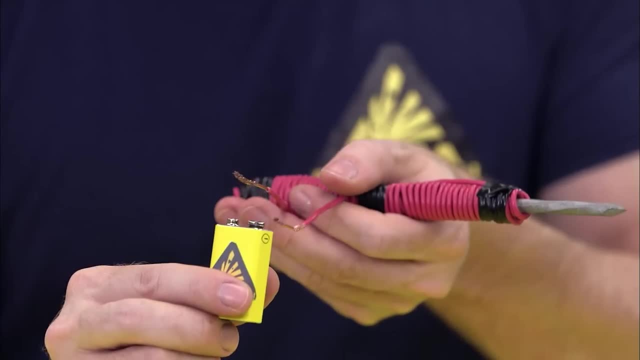 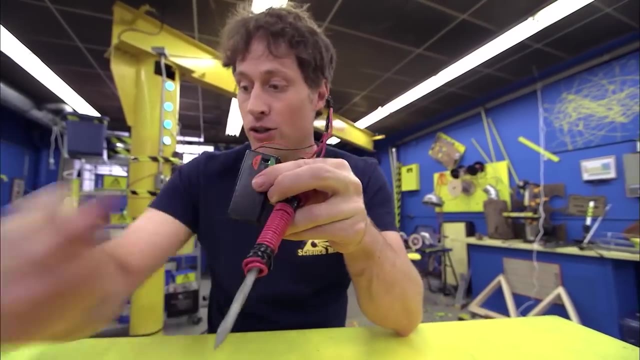 with electrical tape or attach them directly to a battery. if you don't have an on-off switch, And ta-da, you have an electromagnet with your on-off switch. All you need to do is take the things you're going to magnetize. 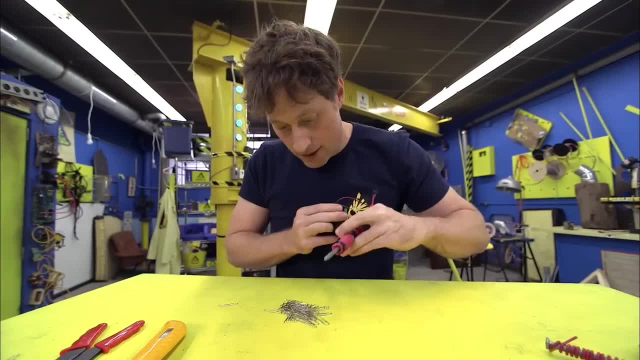 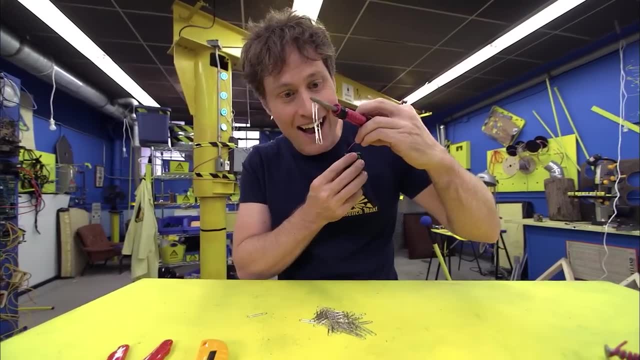 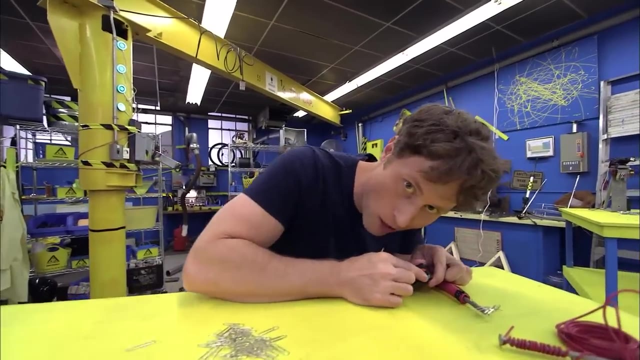 Turn your electromagnet on and suddenly it becomes a magnet. Pretty amazing, Ha, ha ha ha. And then you can magnetize to your heart's content. But when you're done, don't forget you want to turn it off. 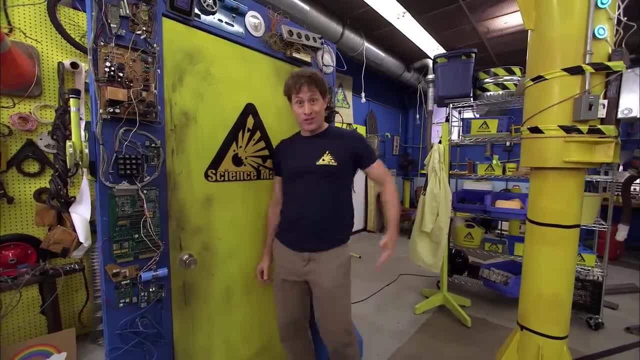 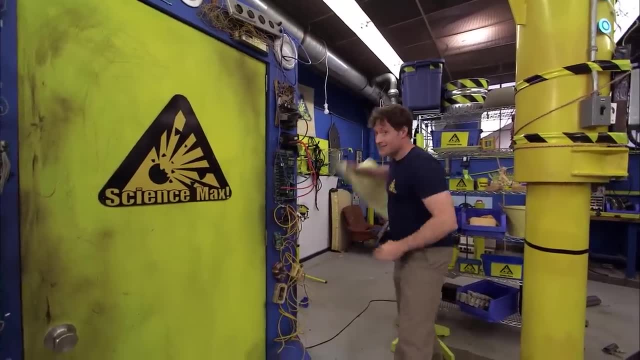 So that's what we're going to do today on Science Max: Experiments At Large. We're going to max out the electromagnet. So where's my lab coat? Oh, there it is. We're going to see how big we can make. 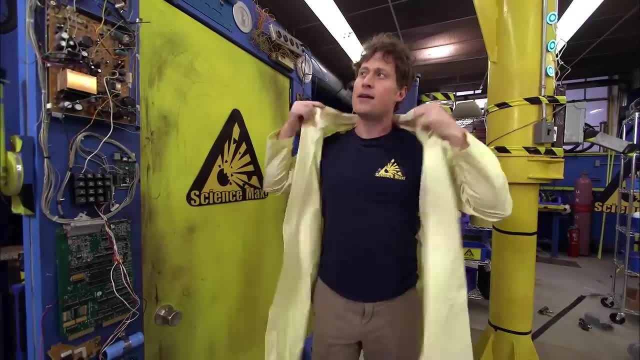 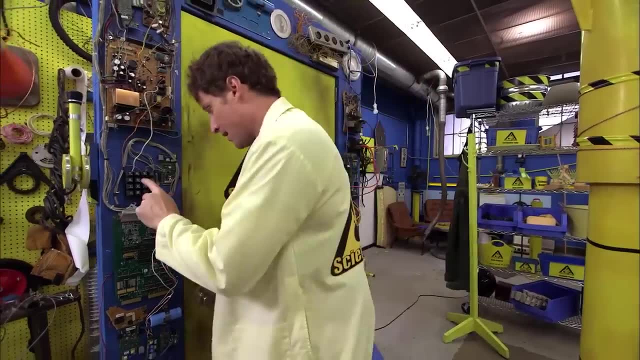 an electromagnet. And when I say we, I mean me and an expert. Let's see, Oh, Heather from the Ontario Science Centre, She knows her way around magnets, So let's see. Uh yeah, I wonder if she's busy. 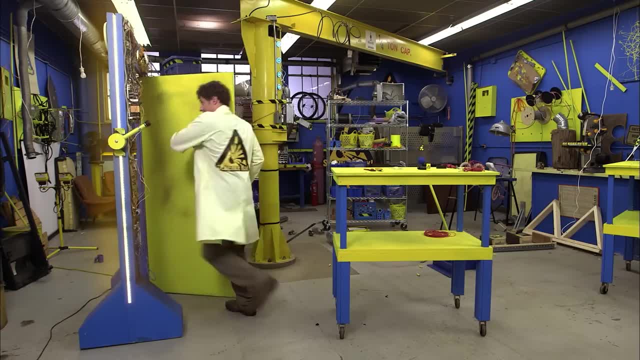 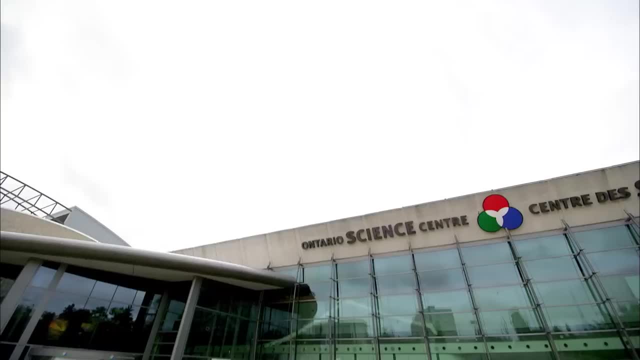 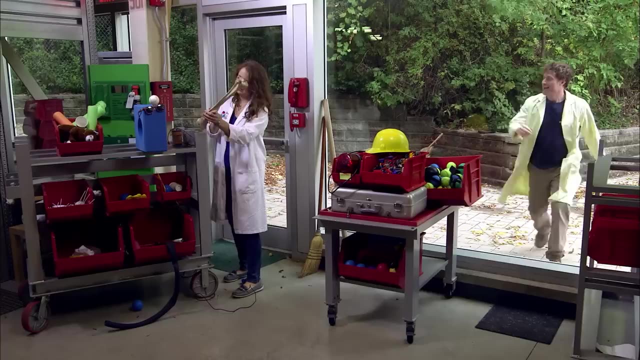 Well, let's find out, And after we're done, I'll need to come back and clean up the giant mess I made in the lab. Let's go. Hey, Hi, Heather, How are you doing? Good, Good to see you, sir. 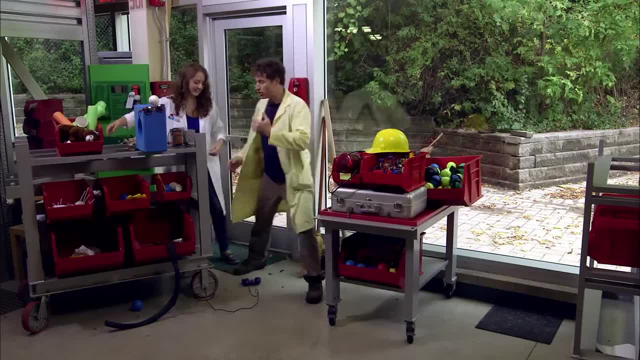 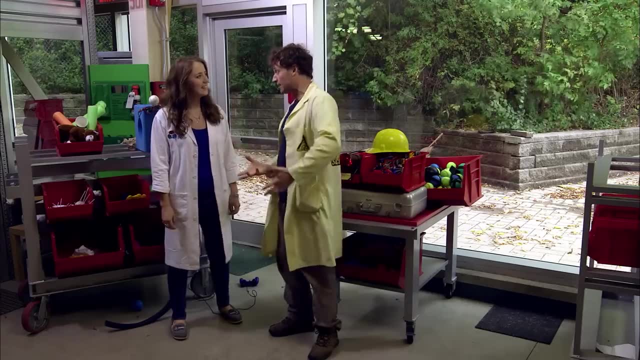 I was just wondering if you could help me with something. Are you busy? No, I've got time. I've got time. Okay, great, Because I'm going to make a giant electromagnet experiment and I need your help. That sounds like. 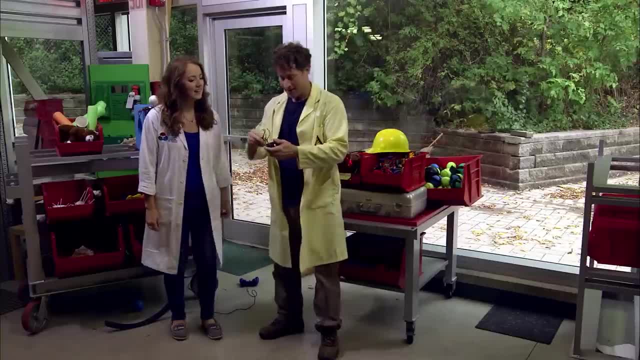 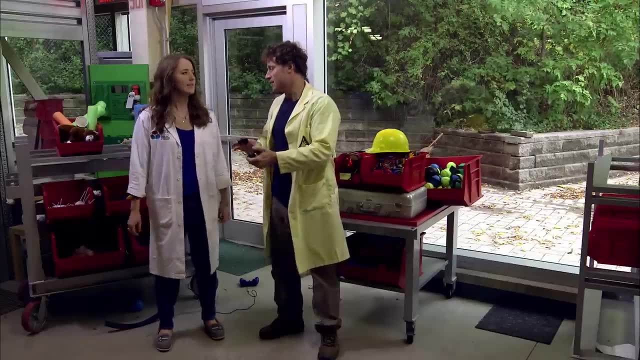 a lot of fun. Okay, great, Let's go back to Science Max headquarters. Oh, via the portal, Yeah, by the portal. Oh, Okay, You sure I know you're hesitant, so I want to reassure you. nothing will go wrong. 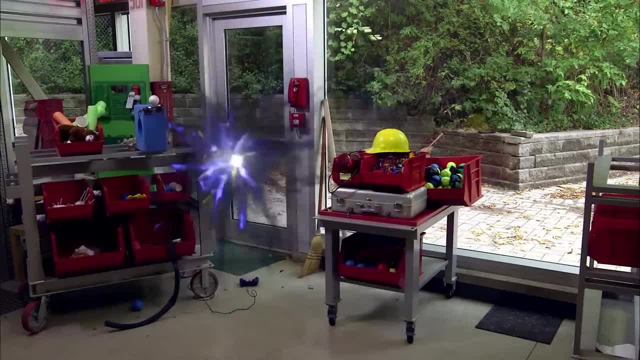 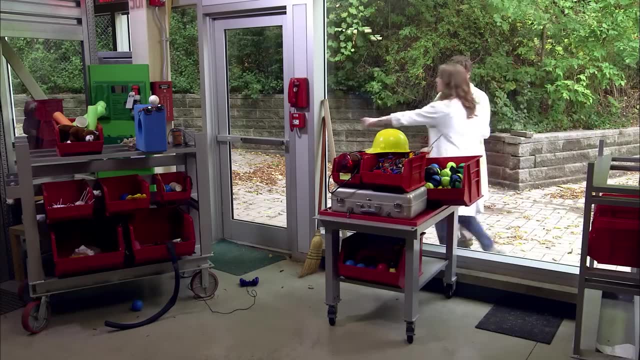 Great, Okay, Okay. Oh hey, We're here, We're outside, It's okay, It's okay, Don't worry about it. No, no, No, I think definitely It's going to be fun, It's going to be fun. 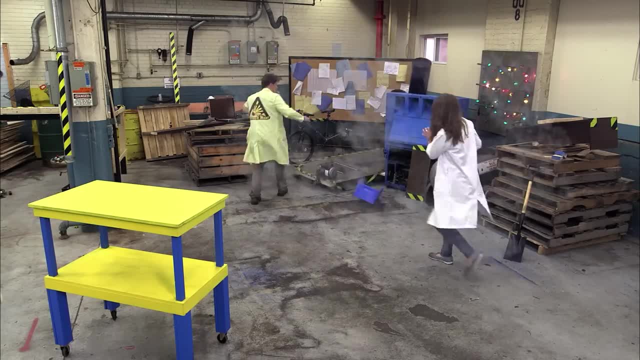 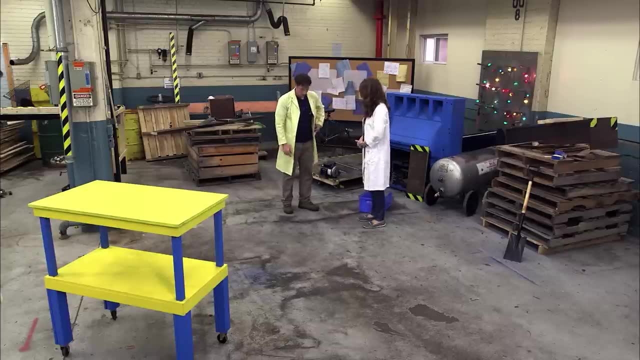 You all right? Yeah, I was supposed to come in over there, but I came in over here, Uh, Oh well. So today, Heather, I want to max out the element that we need to clean up the giant mess in the lab. 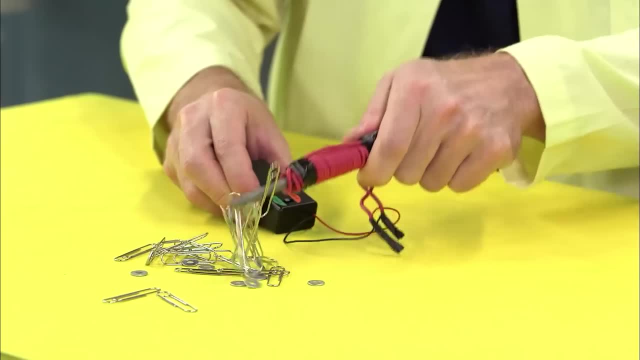 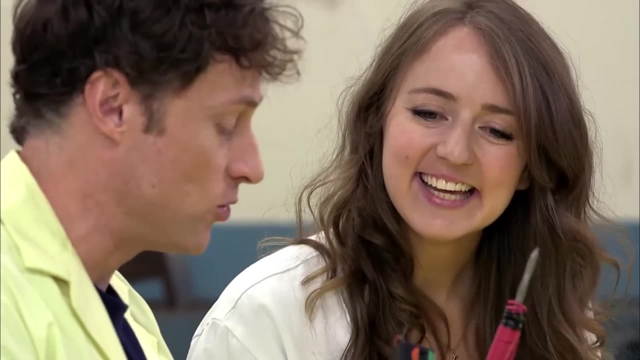 Okay, The electromagnet. Turn it on and it's a magnet, Pretty good. And turn it off and it stops being a magnet. I want to make this into a much bigger, maxed-out version. All right, So what are some? 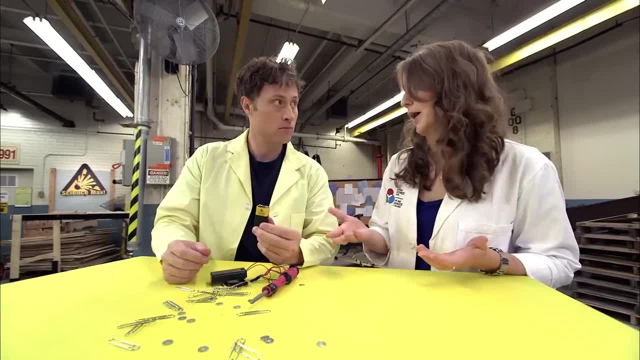 of the things we can do to do that. Well, actually, if you have a larger battery, one that has a higher voltage, we can try that for sure. Okay, That will help. So there are batteries that are 12 volts. 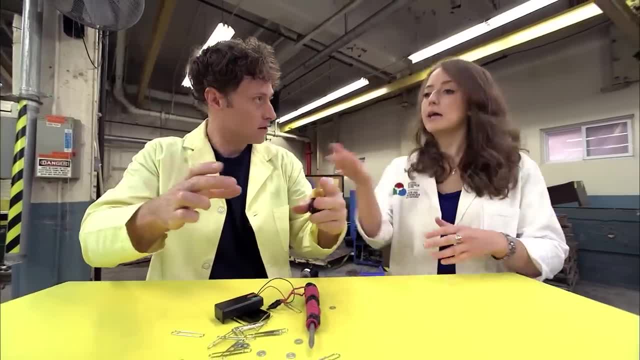 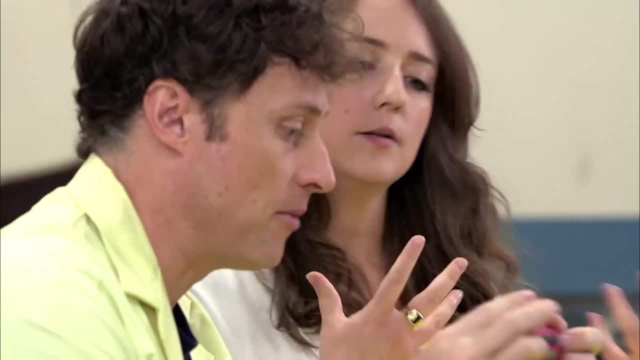 Yes, We could try one of those. I think those are like bigger, right, Yeah, yeah, bigger, more powerful, absolutely. Now, that's one thing we can do. We can also increase the number of wraps of our coil here. 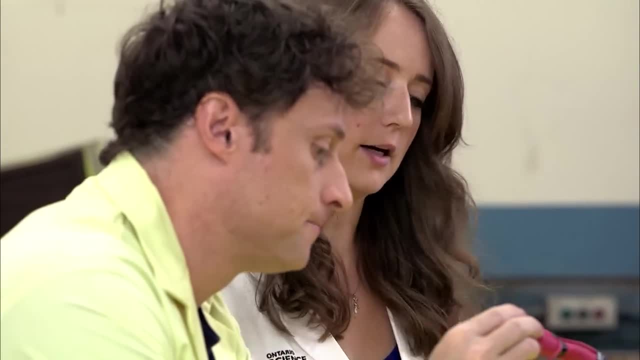 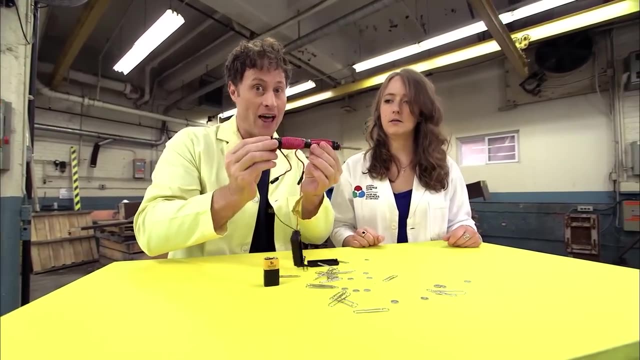 So how many times we wrap that wire? Yes, We'll increase that magnetic field, making our magnet stronger. And, of course, the nail, which is important, because that's the thing that eventually becomes the magnet right Right on. yes, 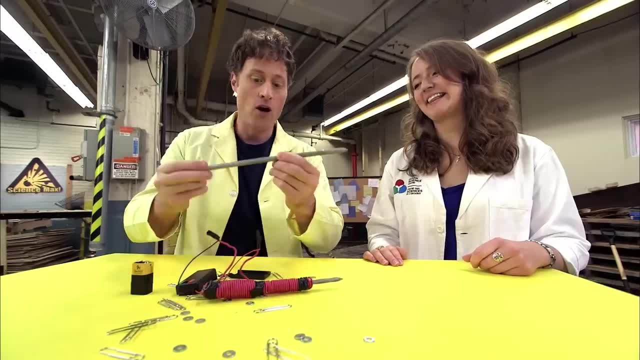 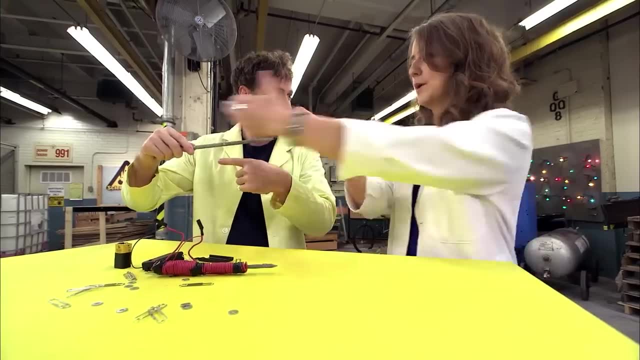 So what I thought we would do is we would start with a bigger nail. What Right So? larger battery, Yes, More voltage and a lot more wraps of the wire Right on. Okay, so we'll get to work Great. 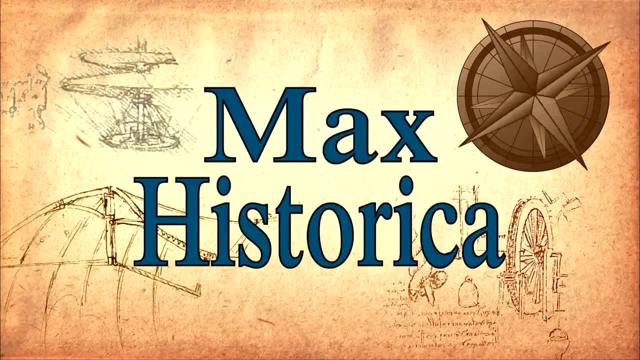 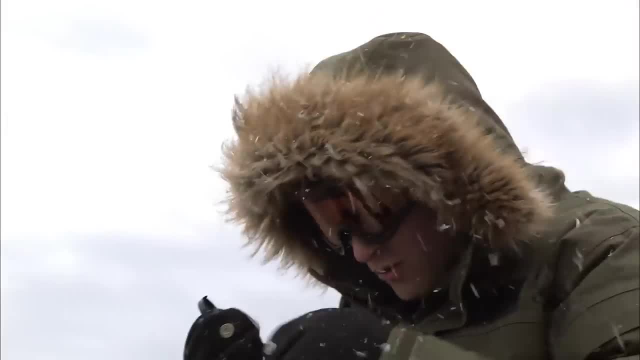 Max Historica. If you've ever seen a compass, you know that the needle points north. That's because a compass needle is a magnet and it points towards the Earth's magnetic North Pole, And I'm using this compass to try to get to the North Pole. 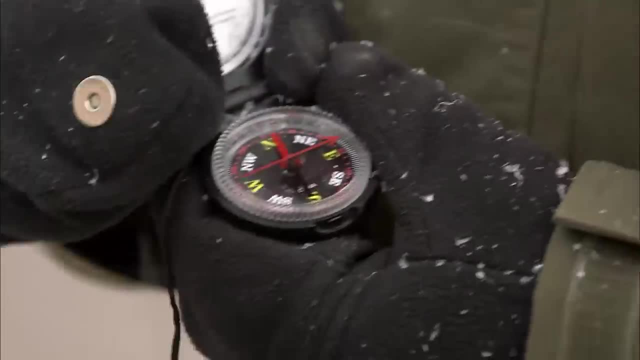 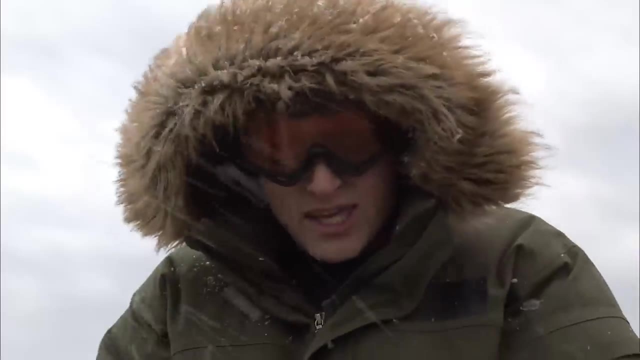 But it isn't easy. In fact, scientists knew there was such a thing as the North Pole, and so they decided to use this compass to try to get to the North Pole. But it isn't easy. In fact, scientists knew there was. 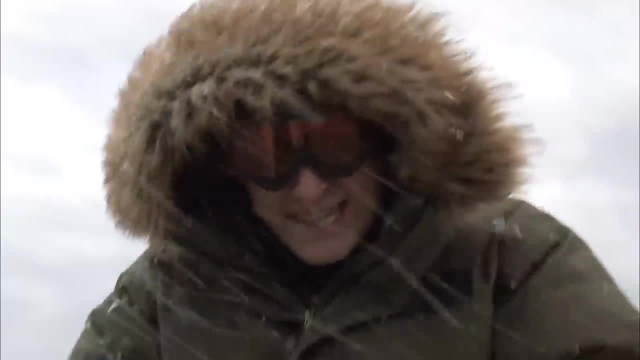 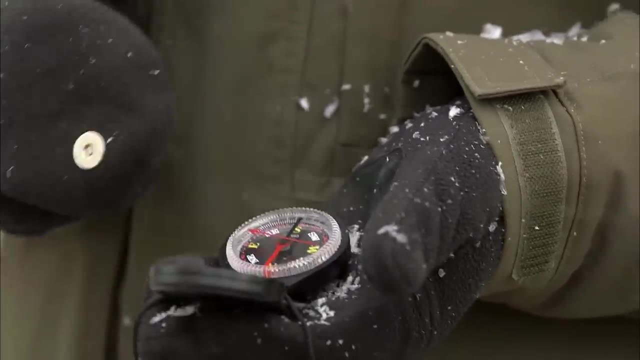 such a thing as the North Pole as far back as the 16th century, But no one was able to actually get there on foot until 1927.. You'd think it wouldn't be that hard, right? I mean the needle points. 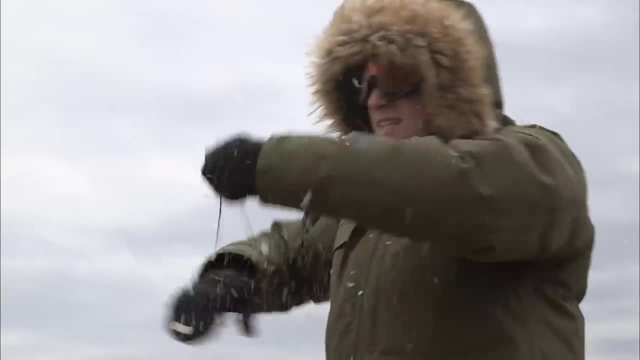 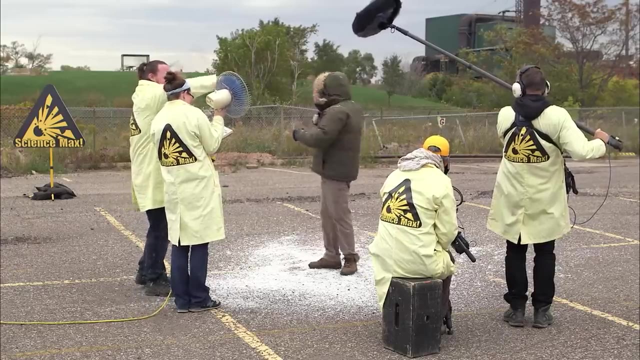 you straight there, Just follow the needle right. But now that I'm here I realize it's really difficult. I mean, the wind is incredible and the snow is intense and it's so cold. my hands are My hands, Yeah, So okay. 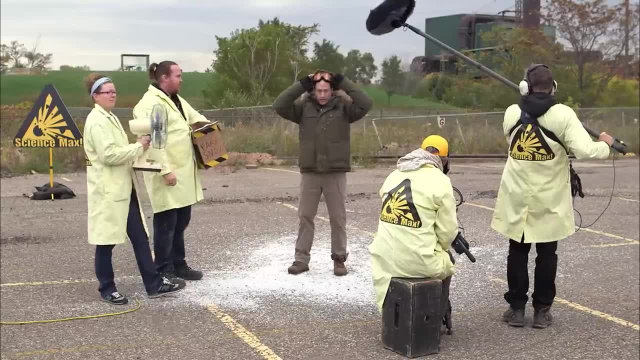 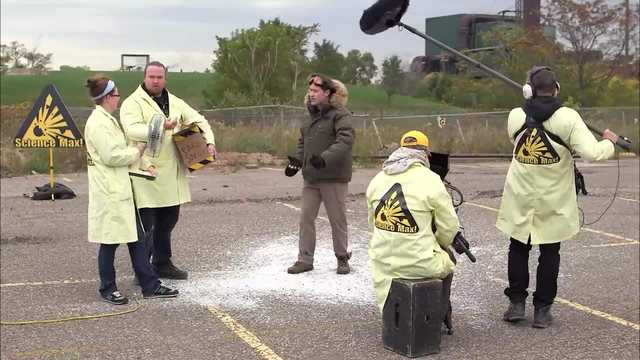 we're not really at the North Pole, We were just sort of recreating that. But still I salute the brave explorers who tried to make it there in the name of science. and I got a sense of it because the wind from the fan. 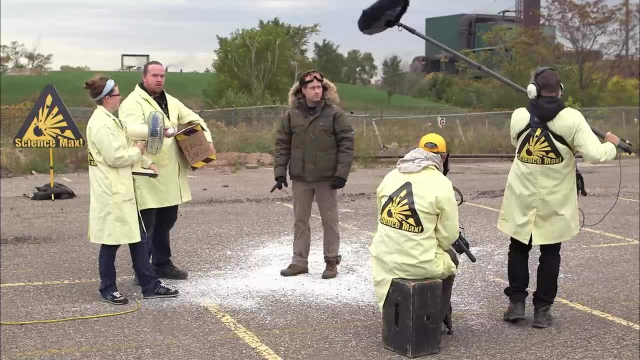 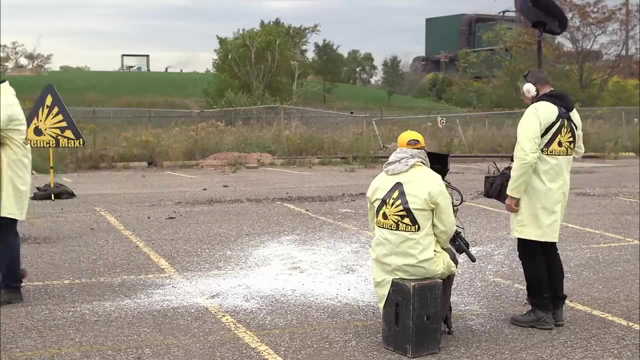 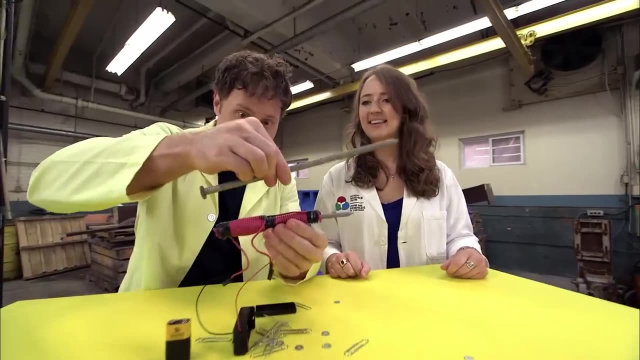 and the fake snow was. Okay, everybody, let's pack it up. I mean, that was pretty good. I just didn't know about that other camera. So back to our main experiment, where Heather and I are building a larger electromagnet. 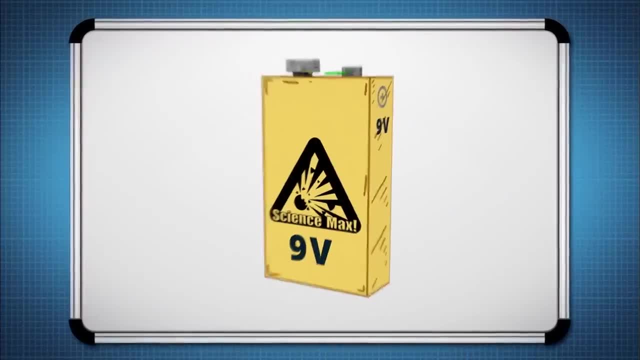 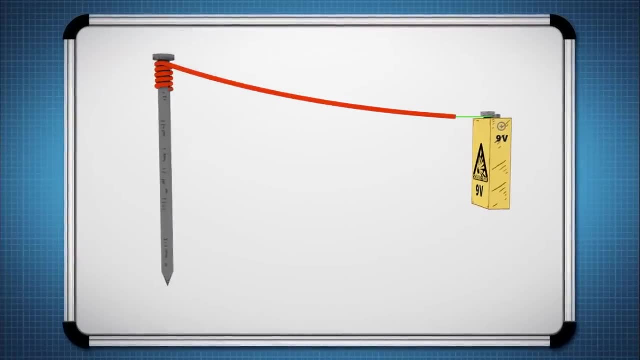 An electromagnet works like this: When an electric current is traveling through a wire, it creates a magnetic field. If you wrap that wire around something ferromagnetic, that's something made out of a metal that is attracted to magnets, like an iron nail. 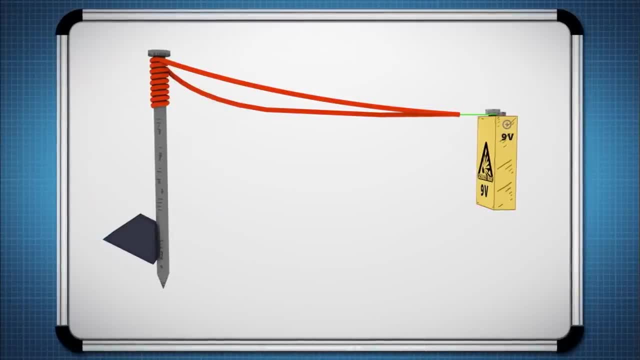 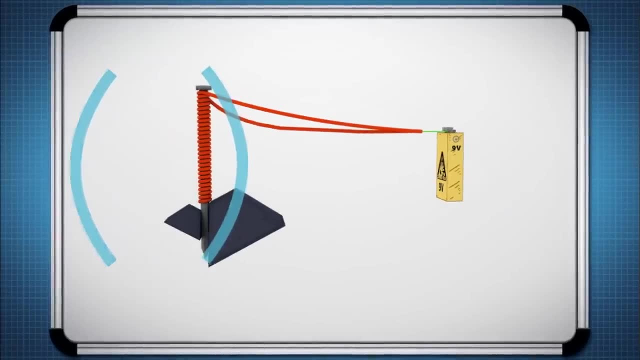 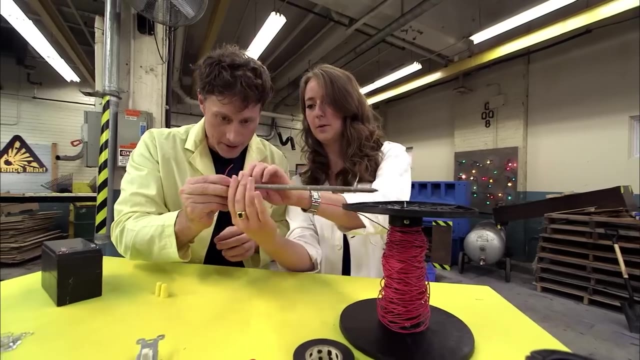 then it becomes a magnet. You can make a magnet stronger by wrapping more wire, which gives more distance for the current to travel, and you can also increase the strength of the current Heather. and I start with a coil of 30 meters of wire and start wrapping. 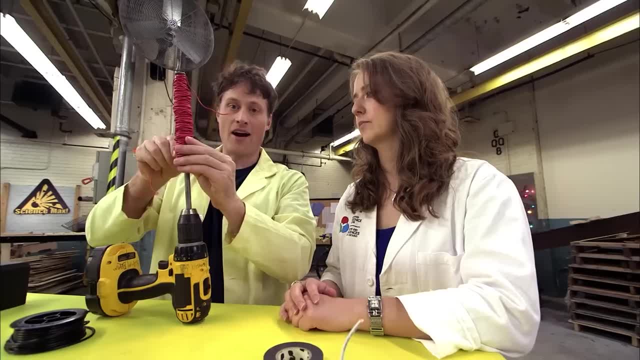 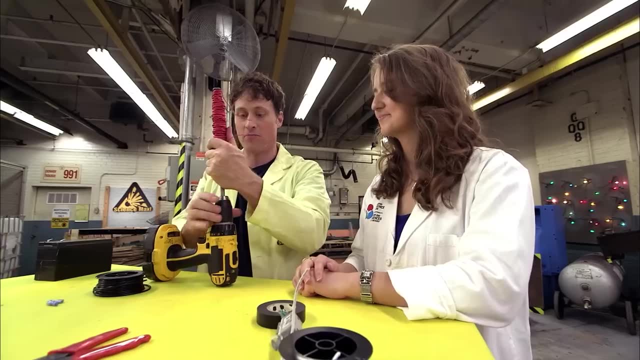 and wrapping, and wrapping There. the wire is now all done. And remember, if you're doing this at home, do not use a drill unless you have an adult to help you out, because drills can be very dangerous. This one goes at a very slow speed. 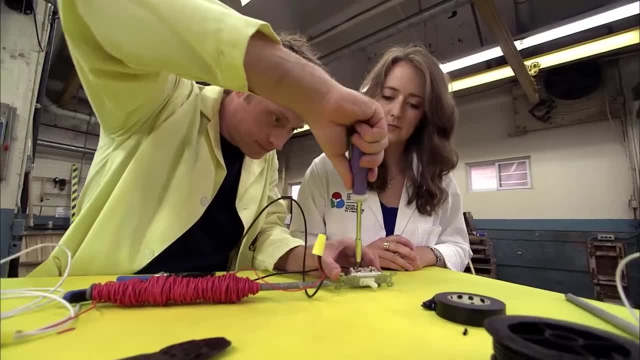 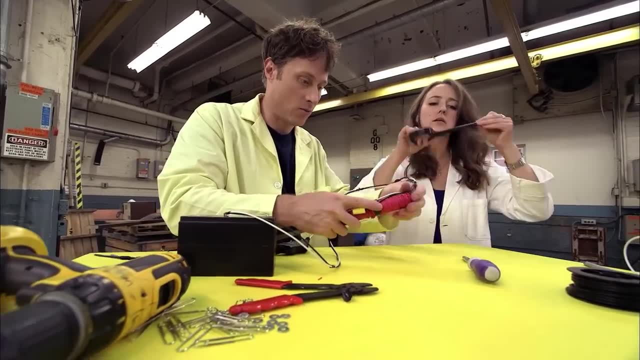 so it was okay. but yes, definitely an adult to help you out. Now let's try another on-off switch and make some leads that connect to a 12-volt battery. So more wraps of wire and more current means: the electromagnet. 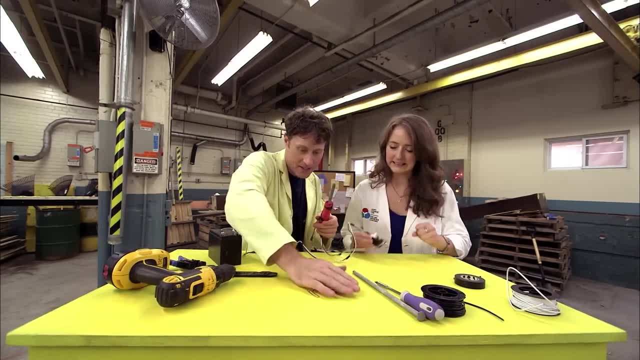 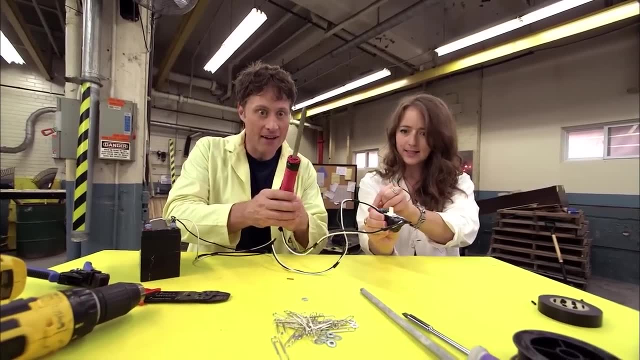 should be stronger. Okay, so we're going to try this electromagnet and we're going to pick up this stuff right here. Great, Are you ready? Yeah, Three, two, one go. Is it on? Yeah, yeah. 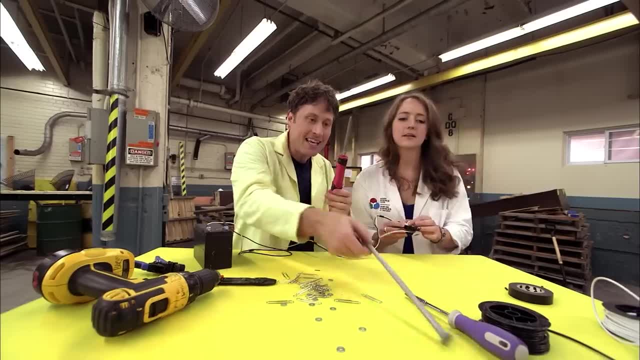 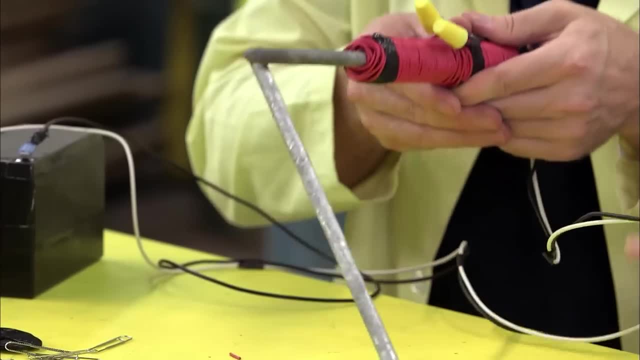 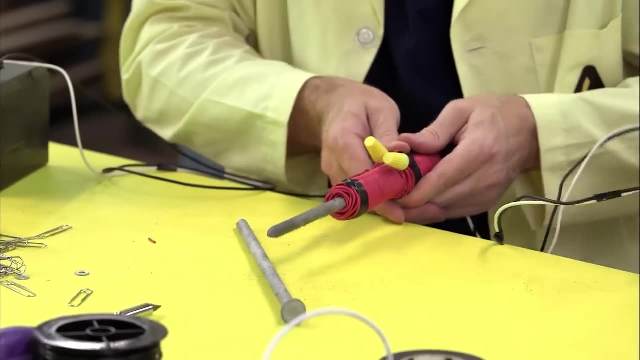 Wow, it really does. huh, Let's see if this nail can pick up this nail. All right, Ready, Ready Go. Uh, uh, oh, Okay, how about this side? Oh no, Uh, no, Hmm. 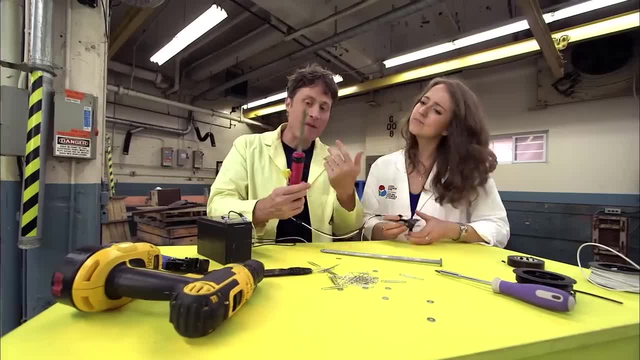 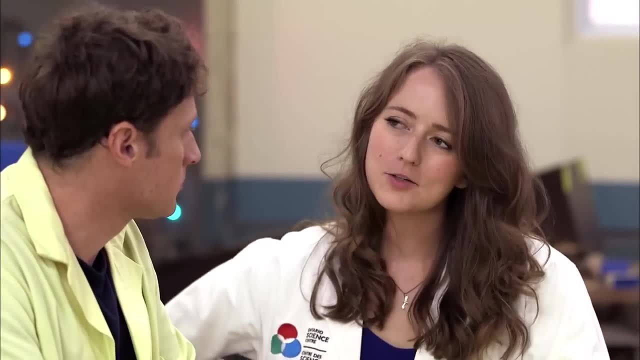 I don't think we're strong enough. It's not strong enough. I think that we need to max this out even more, Even more Right, Um? so I'm thinking there are a lot of appliances that use electromagnets, but it already has. 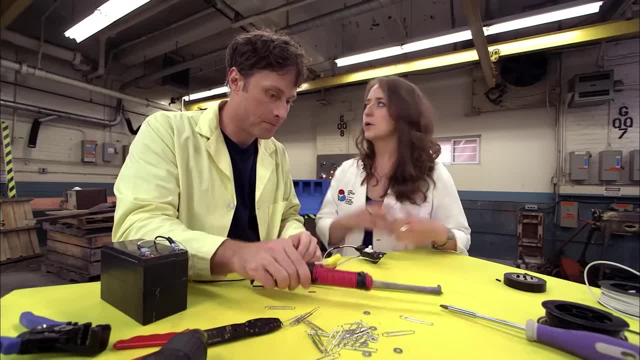 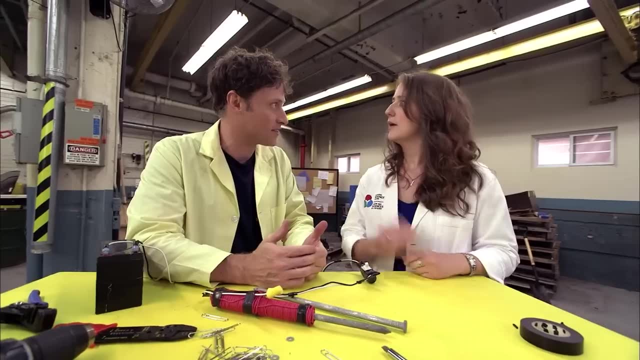 tightly wound coils and high voltage. so we're in a lab here. Maybe do you have old appliances around? I have. I have parts, bins with a whole bunch of stuff. Maybe we could find some electromagnets in those. Let's do it. 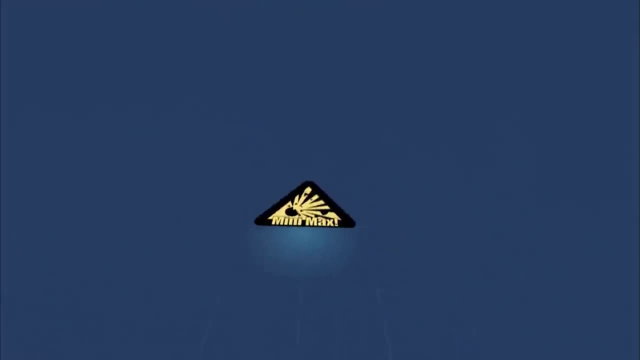 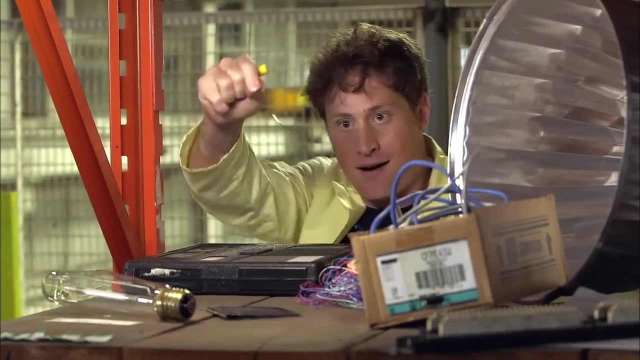 Okay, great, Yeah, Let's go. Mini Max, All right, Pliers, battery, copper wire. Now, if you've already done the electromagnet experiment, here's another experiment that uses all the same magnets, plus these Ha. 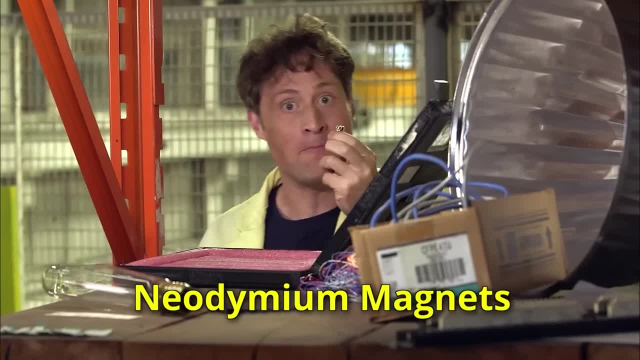 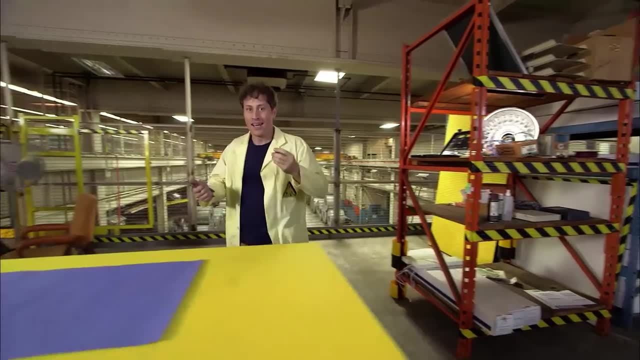 Neodymium magnets, some of the strongest magnets you can get. So here's what you need: A battery, some neodymium magnets the same diameter as your battery, copper wire and some pliers. So here's what you do. 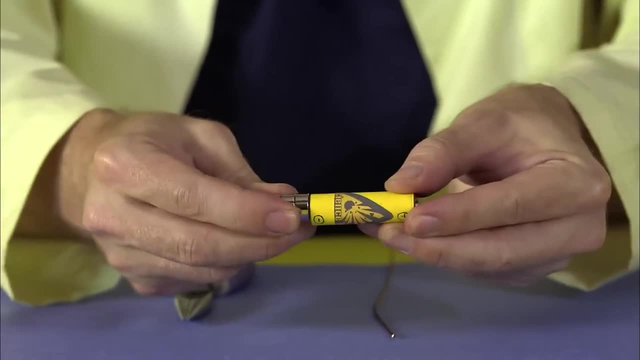 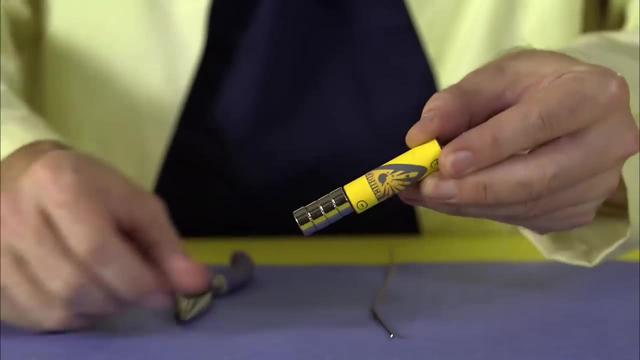 First thing is you put the batteries and the magnets together like that. Then what you want to do is bend the wire so it's tight enough to hold the magnet in place. Now what you want to do is you want to bend the wire. 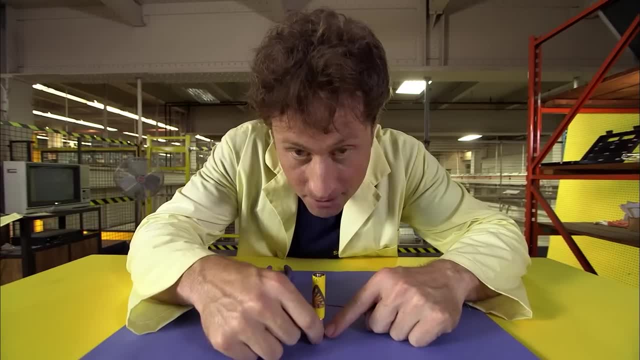 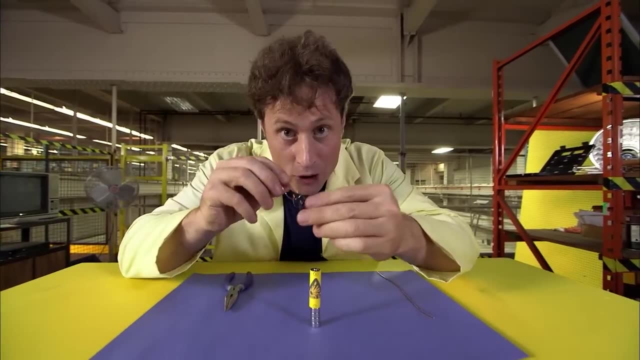 so it's touching the top of the battery and goes around the battery and then touches the magnets at the bottom. Here's what that might look like. I say might because you can do any shape you want. I've made a coil here and if you put it- 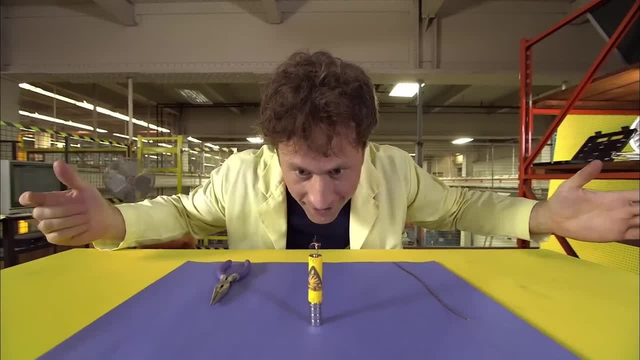 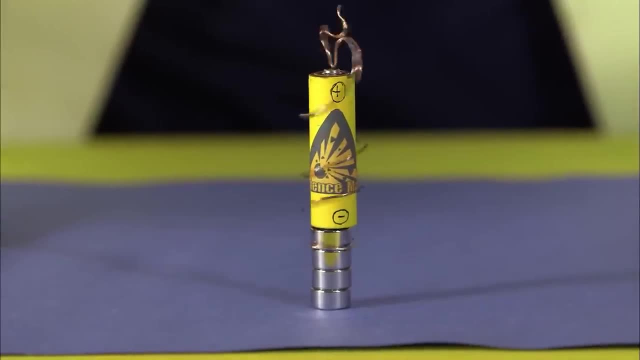 over the battery. you'll see it only touches the very top of the battery and the magnets at the bottom And if I let it go, it spins. It's a homopolar motor. What happens is the battery sends an electric current and that turns it. 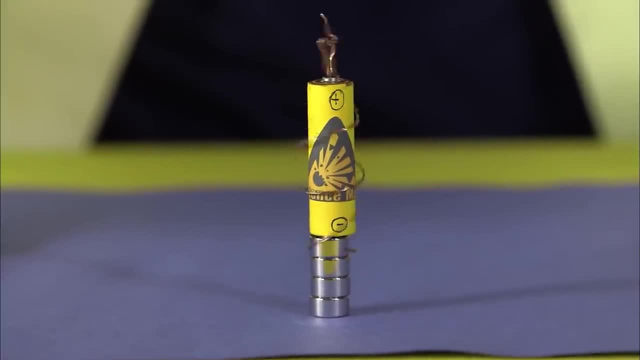 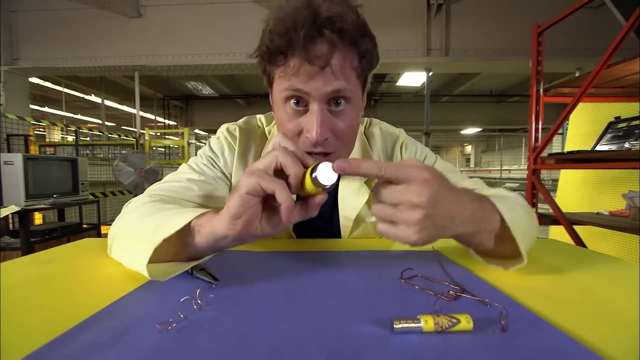 into an electromagnet which is attracted to the magnets at the bottom and it spins. So now let's max it out. Ha-ha, A D-cell battery which is larger, and, of course, larger neodymium magnets. 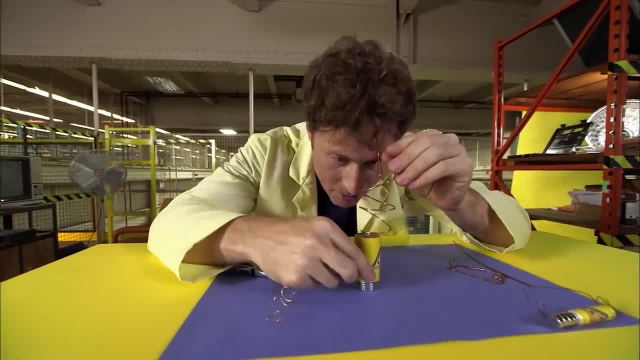 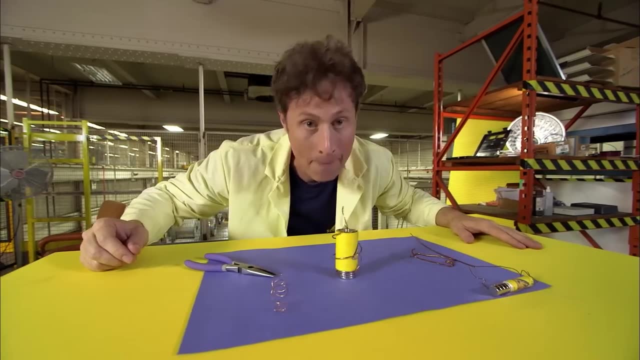 And you do the same thing. Make a coil that only touches the battery at the top and at the magnet and, Ha-ha, It spins Max out. homopolar motor. But don't worry, This is not the biggest size we're going to do. 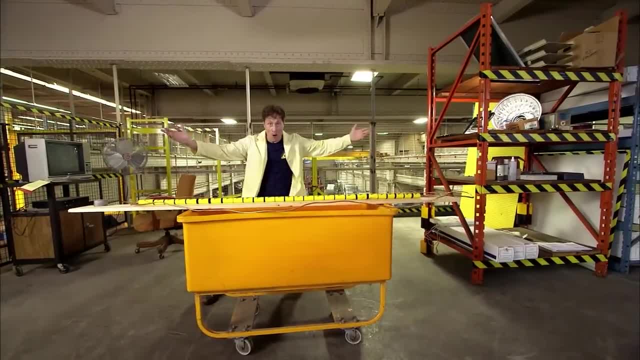 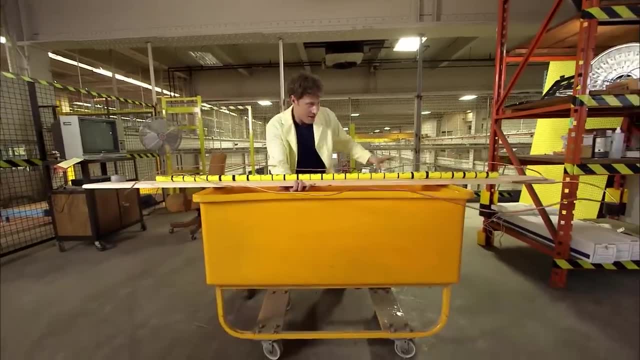 Ha-ha-ha-ha-ha Maxed out homopolar motor. I have 27 D-cell batteries, a giant copper tube and a neodymium magnet. So I'm just going to, And then we get. 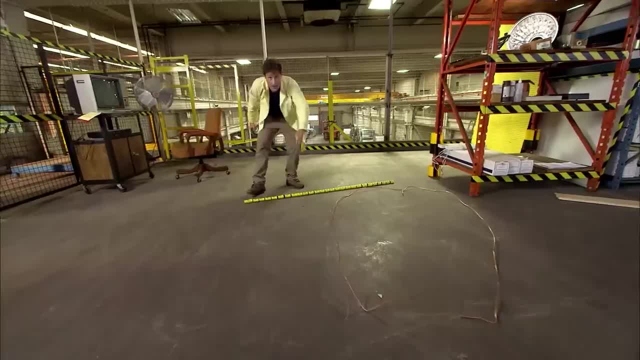 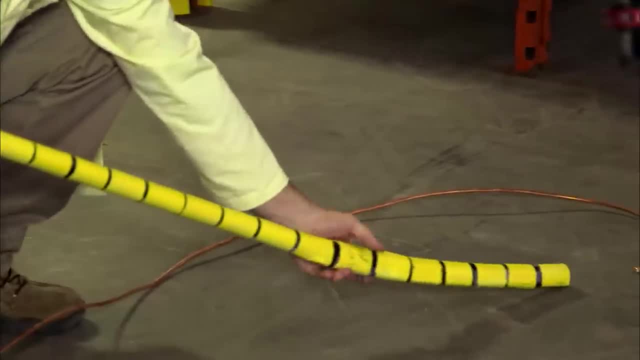 Get rid of that. Put this down, Okay, so the first thing I do is attach the neodymium magnet to the batteries, And I've got all the batteries taped together here, so they'll sort of stand up like like this: Huh. 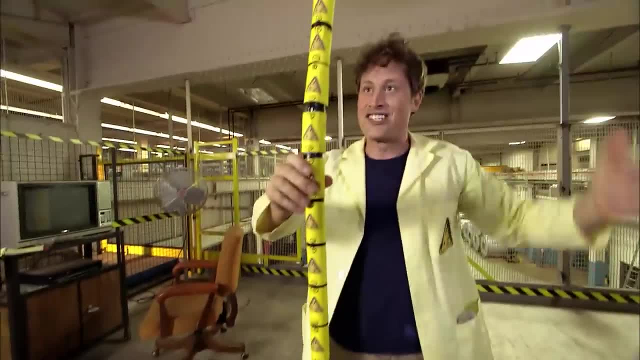 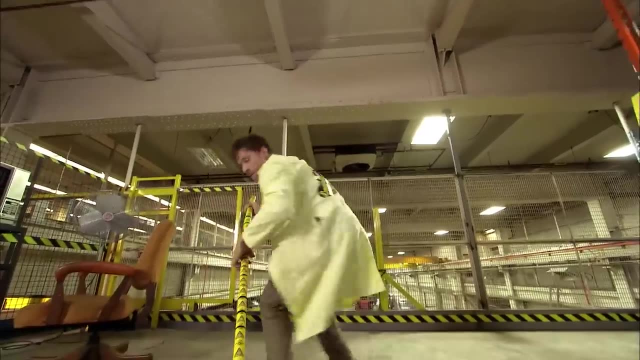 Ha-ha, Ha-ha-ha-ha-ha- Giant stack of D-cell batteries. Okay, Now what I do is I take the copper co, I take the copper coil. Um, I need to get, I need to get. 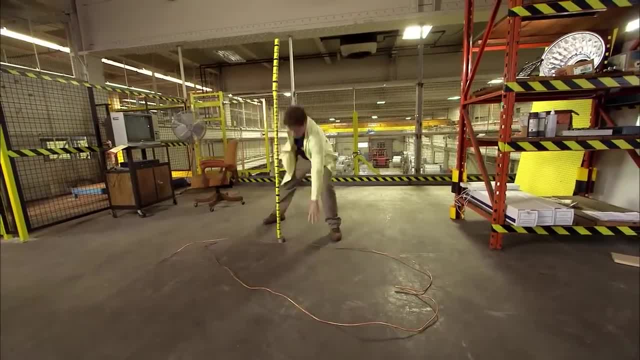 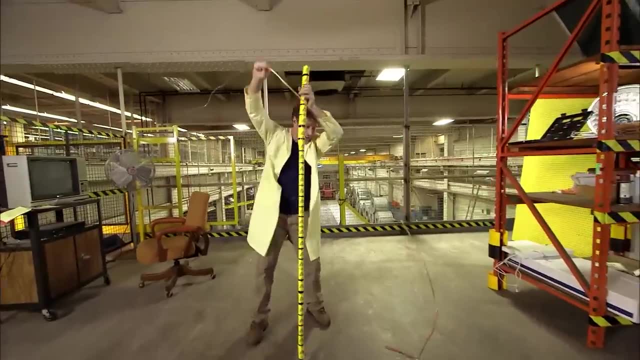 Okay, Hold on, Hold on. I got this. I just need to get the copper coil in. Ha-ha-ha-ha-ha, I did it, Okay, So I take the copper and I put it on top of the. 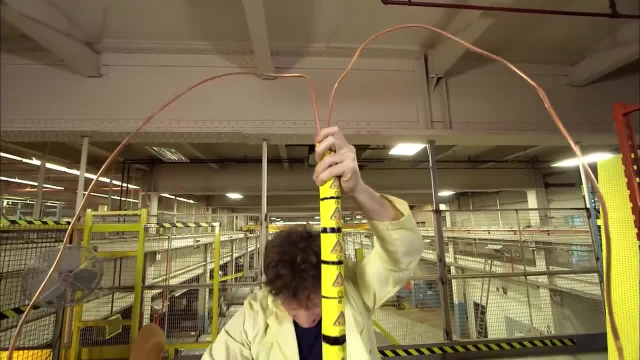 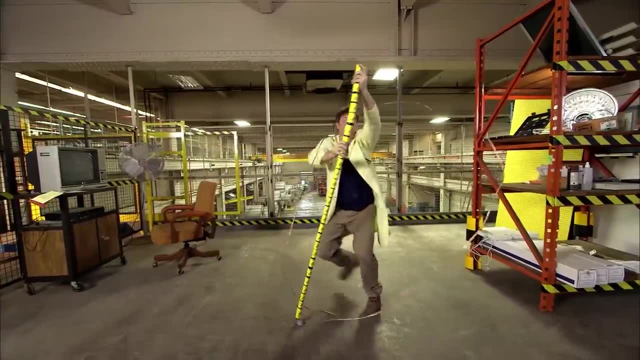 D-cell batteries like this, And then I Let it go. Let it go. Nope, Whoa Homopolar motor. Okay, So that didn't work, But that's okay. I like it when it doesn't work. 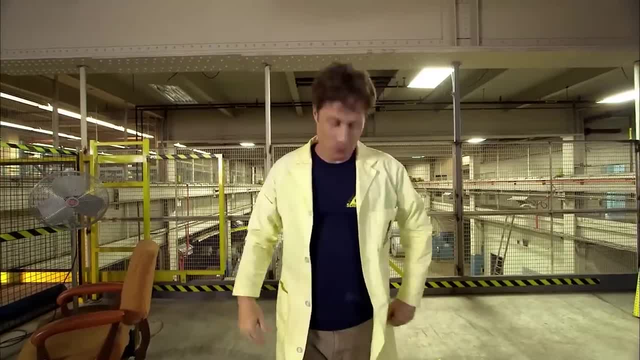 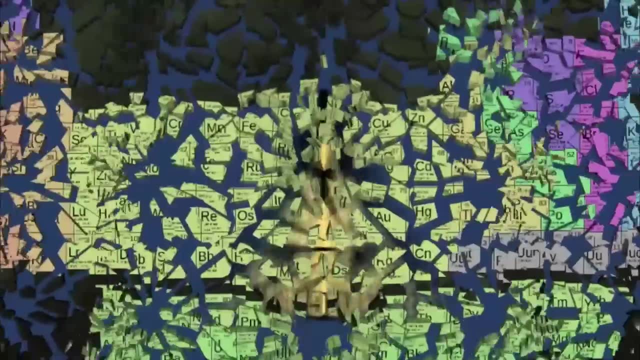 because that's science. It's not science if it works perfectly every time. I mean you got to have some room for improvement. How do you know if the battery is working or not? Heather and I built a larger electromagnet, but it still wasn't. 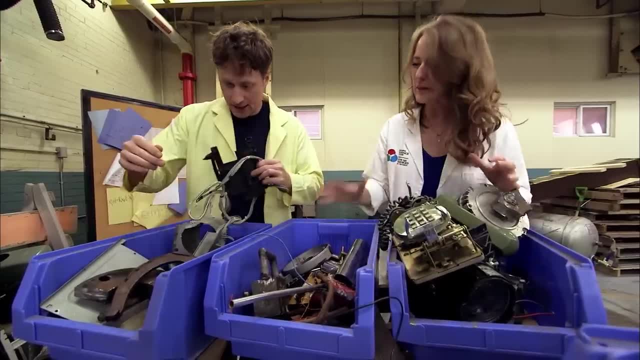 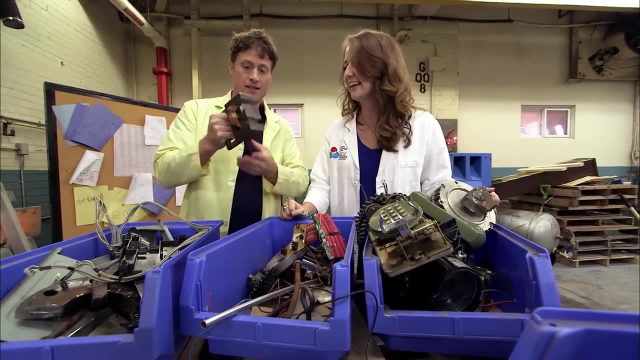 as powerful as we hoped. So now we're searching for parts that came out of an appliance that are pre-built electromagnets. What about this? I think that'll do the trick. Do you think this is? This does look like an electromagnet. 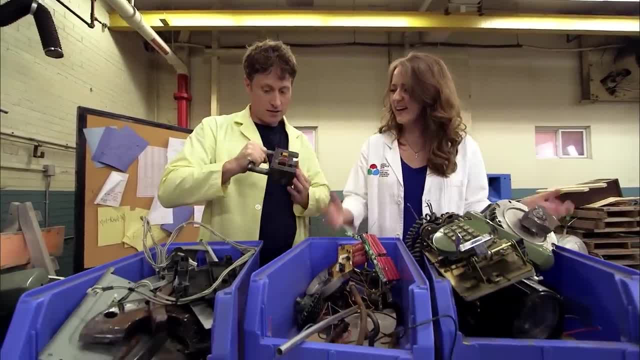 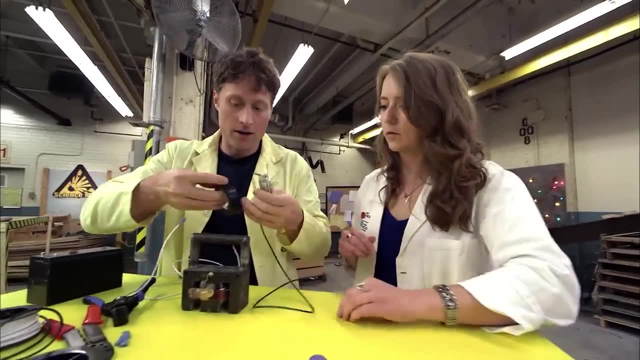 huh, It does. yeah, And there's a whole big bunch of copper wires coiled on that, Coiled around. So you think we can use this? Yeah, let's try it. So it's just a matter of attaching wires. 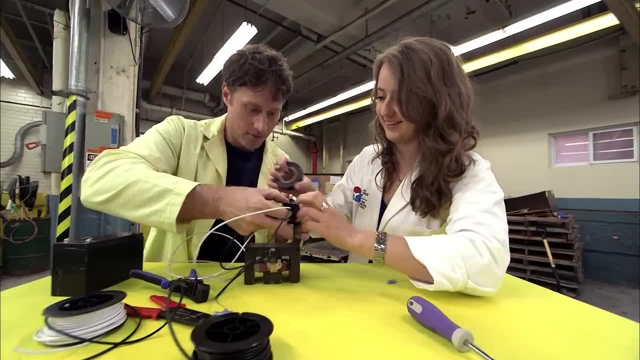 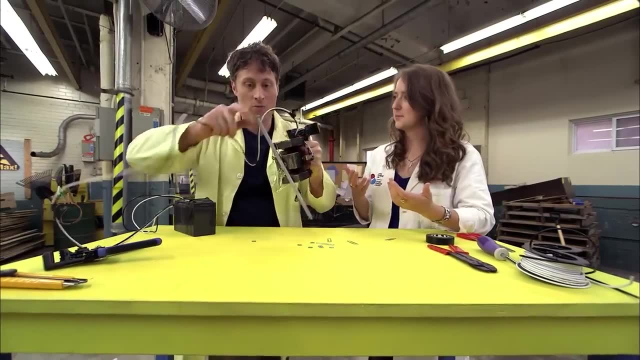 and an on-off switch and attaching all of it to a 12-volt battery. Do you think 12 volts will be enough? Let's find out. I think so. Try that Once we do. it works much better Oh. 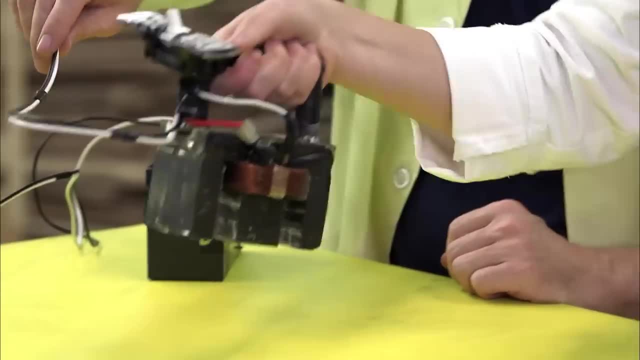 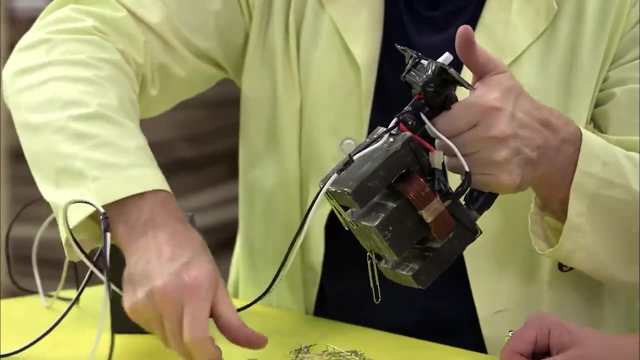 No problem at all, Ready. Yep, Turn it on On. Whoa, Pretty good. Okay, Off Off Neat. In case it was really strong, I have the next step: Horseshoe. Okay, Ready. 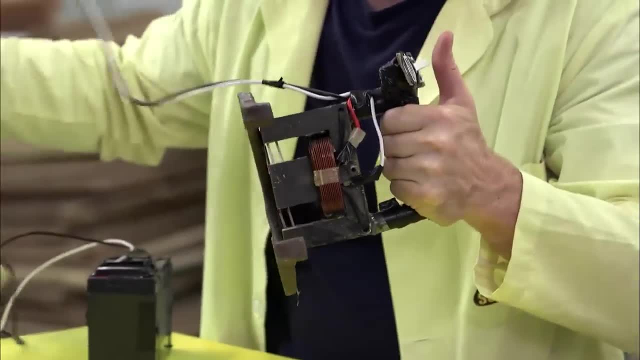 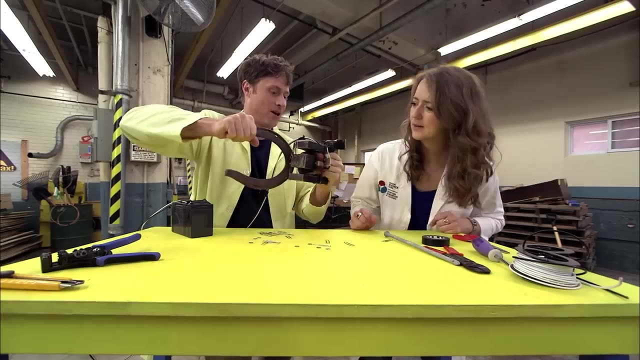 Whoa, That's Fair. I can't pull that off. I, Okay, wait, We'll grab this. Okay, Work together. Yep, Wow, So that's passed all of our tests. Yeah, This is really strong. 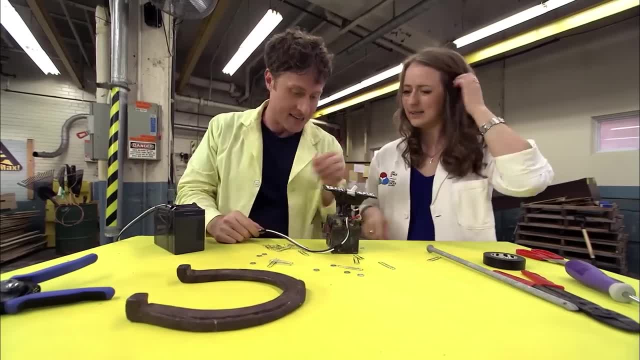 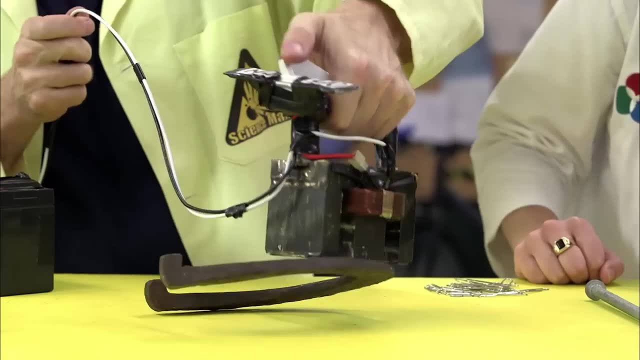 Um, Is there a way to test it further In order to test how strong our magnet is? it's as easy as seeing how much weight it'll lift, So let's test how strong our magnet is. Heather and I find a metal table. 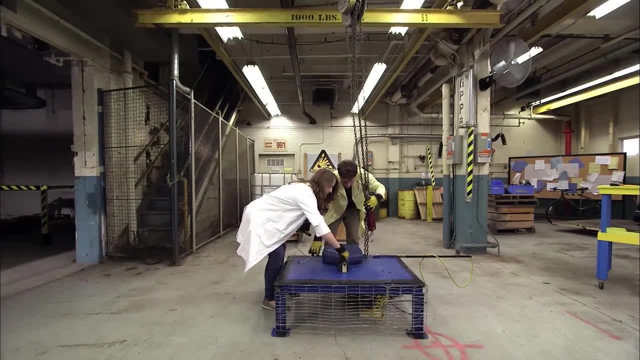 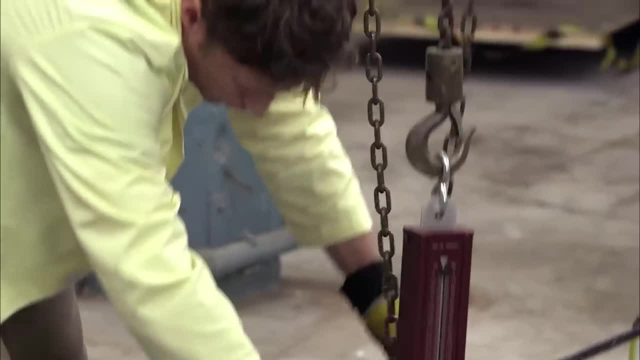 All right, Phil, So I brought the electromagnet. Okay, Just put it right here. Yep, We add some sandbags for more weight and then attach a scale so we can measure how much weight we're lifting. We use a chain hoist. 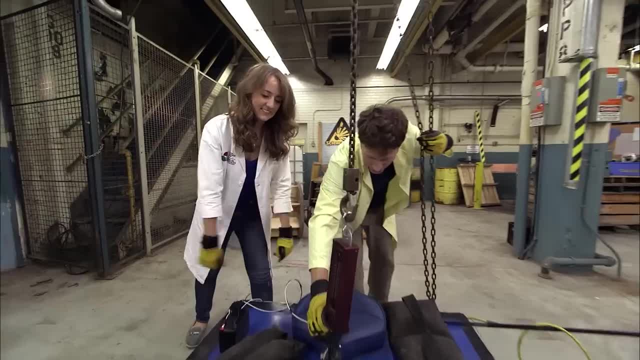 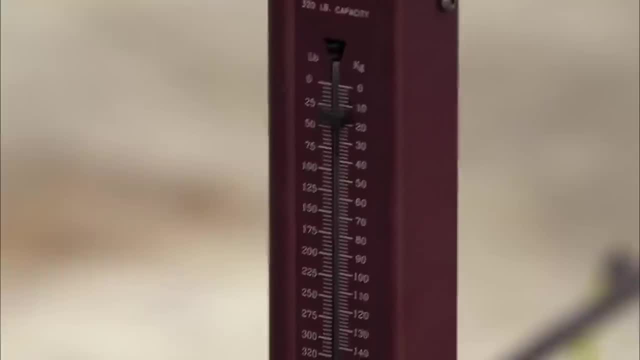 a simple machine made for lifting heavy things. This one can hold up to 454 kilograms. Want to turn it on Ready Yep, Here we go. You can read on the scale how much weight we're lifting. The scale's going up. 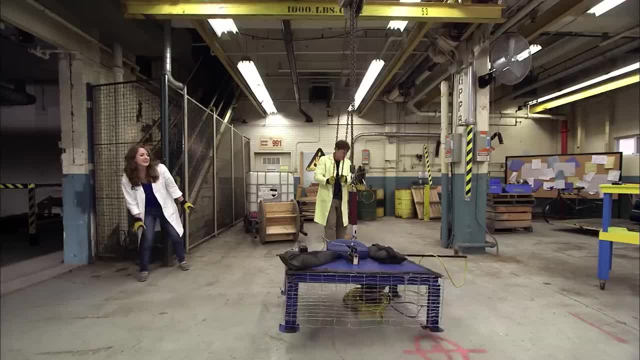 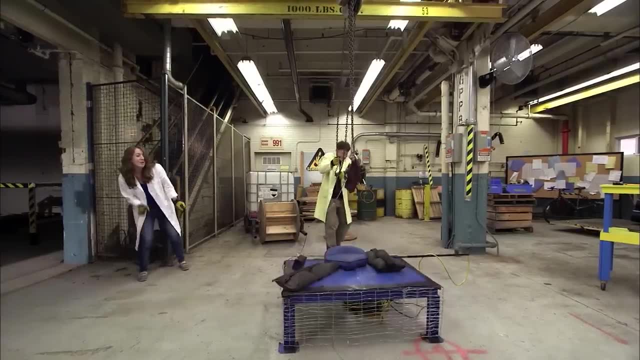 Pounds on this side, Kilograms on this side. We keep lifting until Oh, Oh, Oh, Okay. So how much did it hold? It held 100 kilograms. Oh, That's more than I weigh, which gives me. 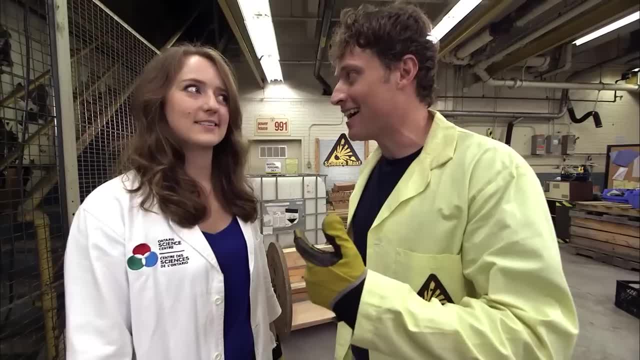 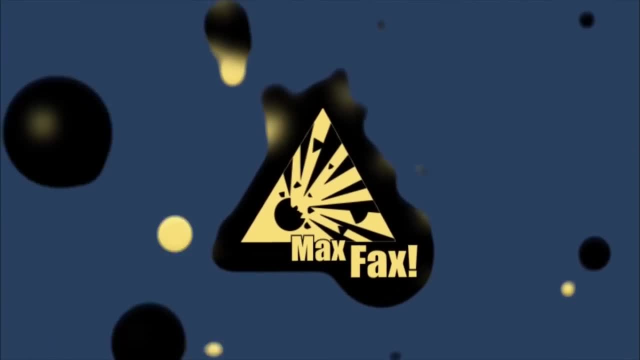 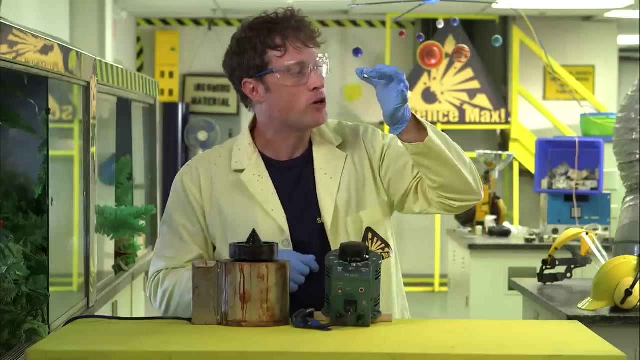 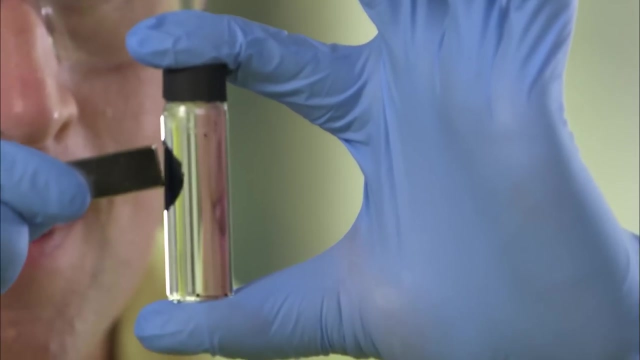 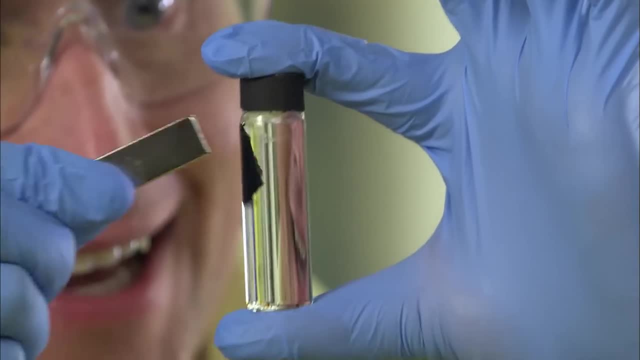 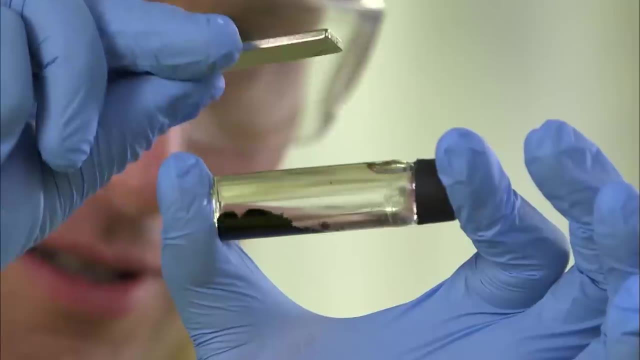 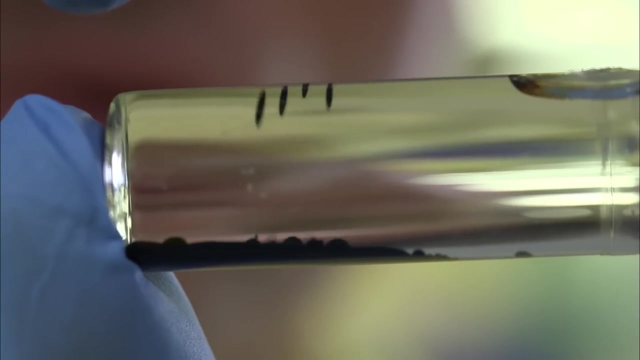 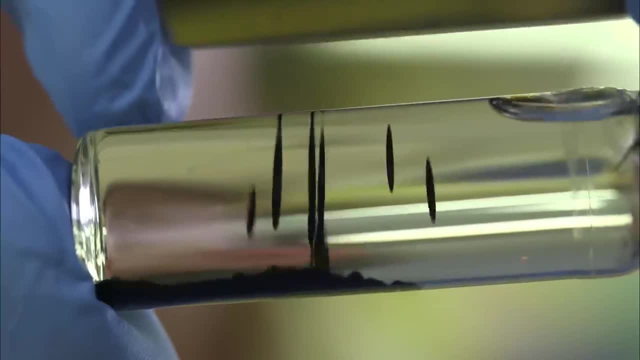 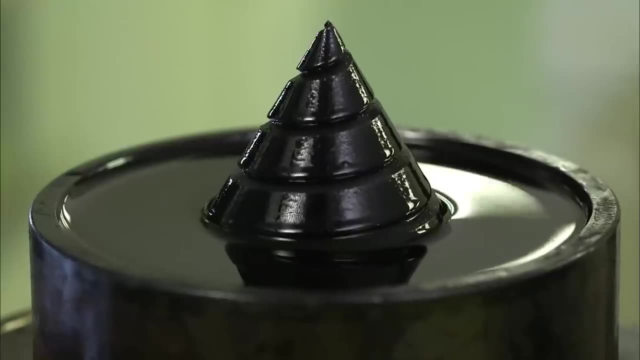 You can see the magnetic field in 3D. It's even more impressive when we max it out. This is ferrofluid outside of a glass jar. Now it's sitting in a pool around this electromagnet And this is a dial which I can use. 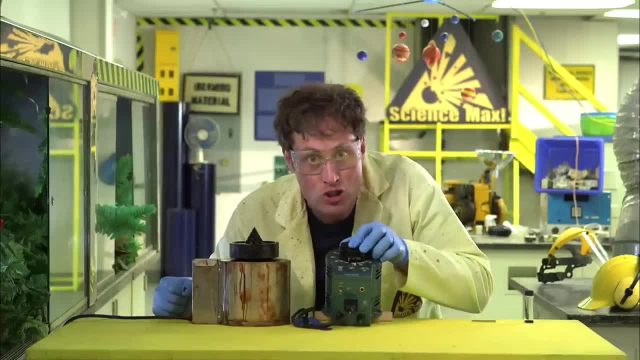 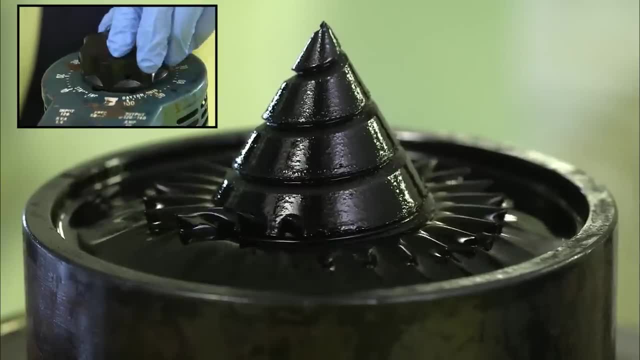 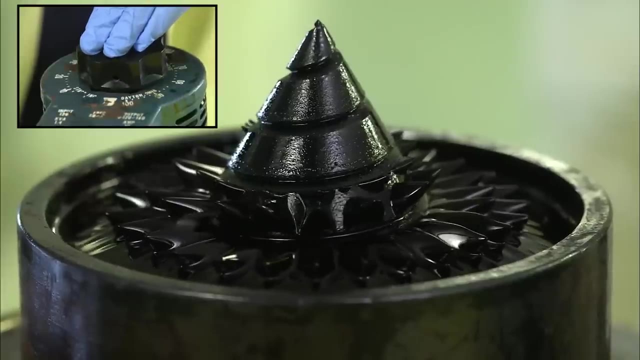 to change the voltage of the electromagnet, making the magnet stronger. Watch this: Changing the current going to the spiral in the middle turns it into a magnet. The more current I put in, the stronger that magnet becomes, allowing the ferrofluid to climb the spiral to the top. 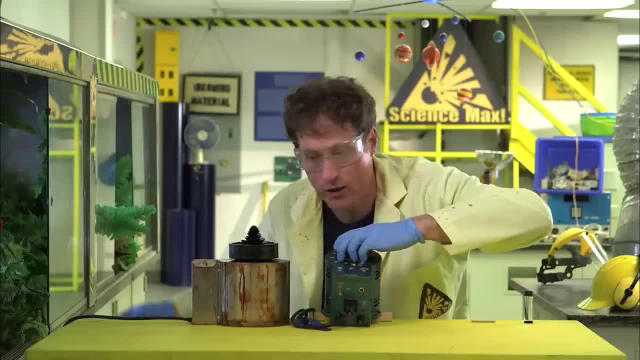 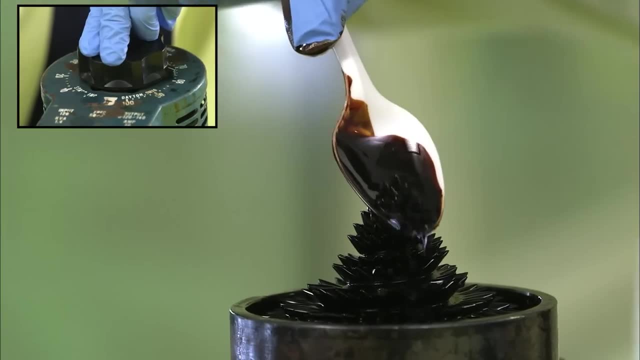 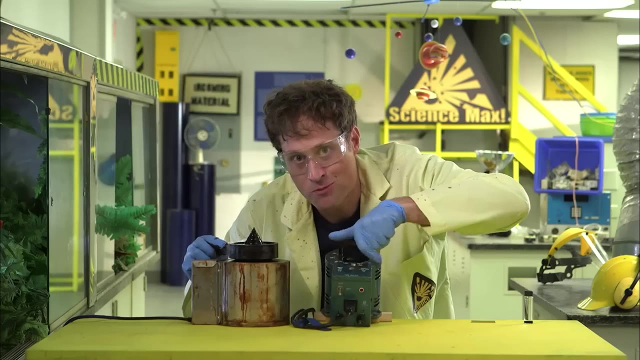 And remember, even though it looks all spiky, it's still a liquid. I will demonstrate with my plastic spoon And watch this. When I turn the magnet off, it stops being spiky. Turn it on, Turn it off. 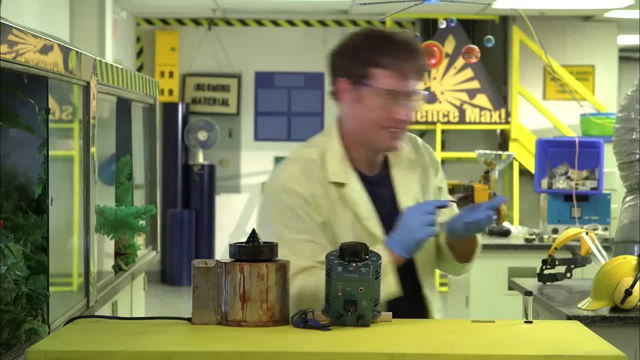 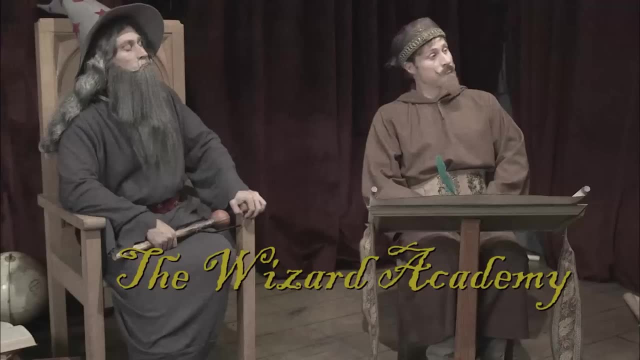 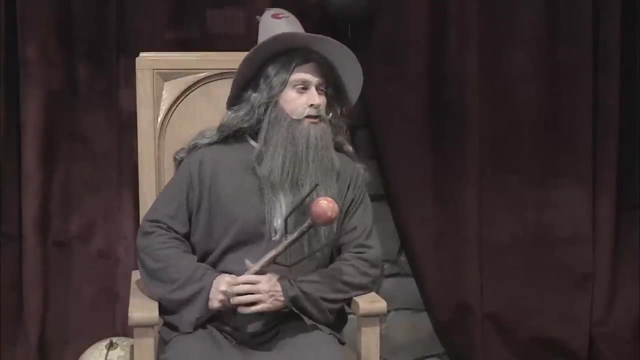 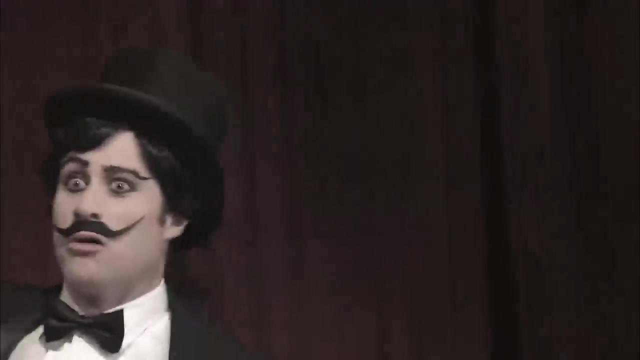 Science, The Wizard Academy. All you have to do is demonstrate true magic and you will be granted entry. Well, fuzzix, who is the next applicant for the Wizard Academy? Overwhelmer, Indeed, it is I Overwhelmer. 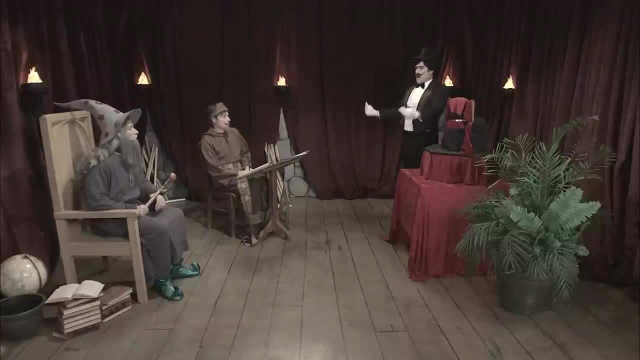 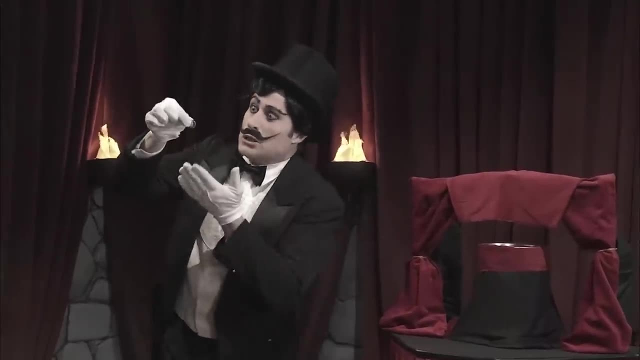 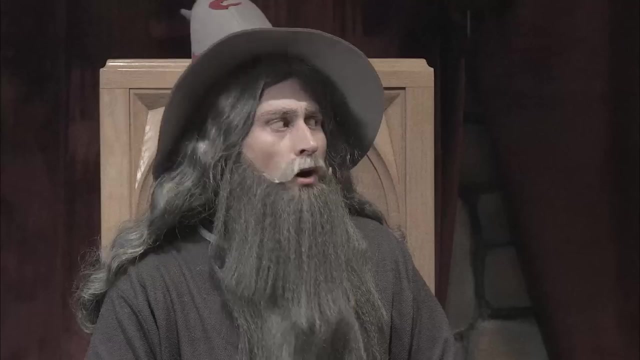 And prepare to be overwhelmed-o. Would you be flabbergastified if I balanced this coin on its end? Not really, no, But would you be impressed if I was to balance this coin on top of this coin? Possibly Prepare to be flustered and stoopified. 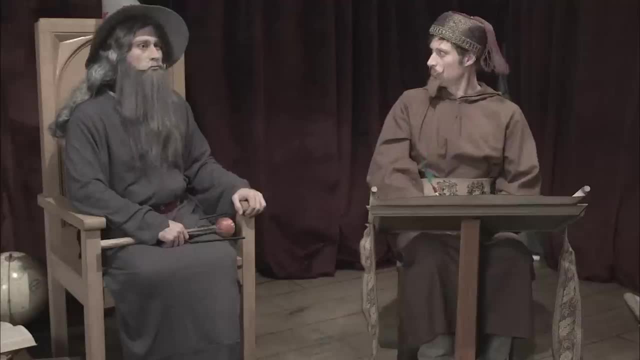 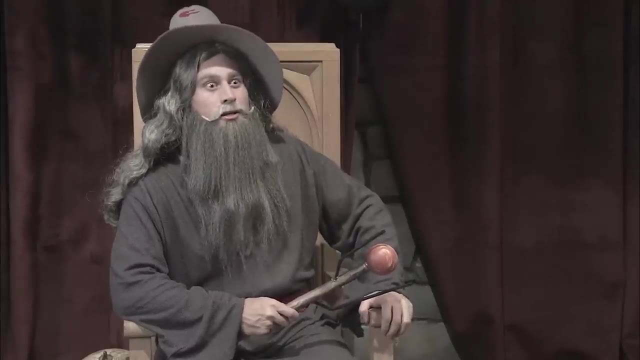 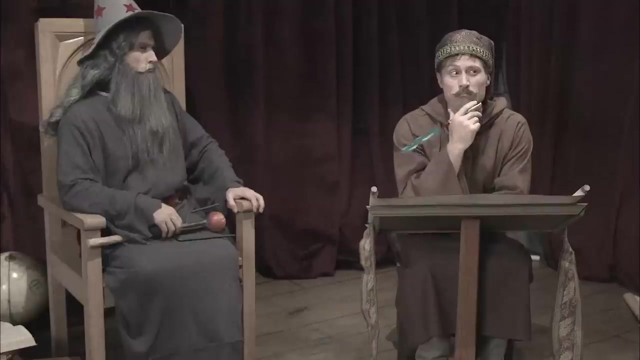 Stoopy, Stoopy, flustered, As I balance three, Three coins on their ends on top of this glass. Well, that certainly would seem like magic. Let us see. Okay, No pressure Overwhelmer, You can do this. 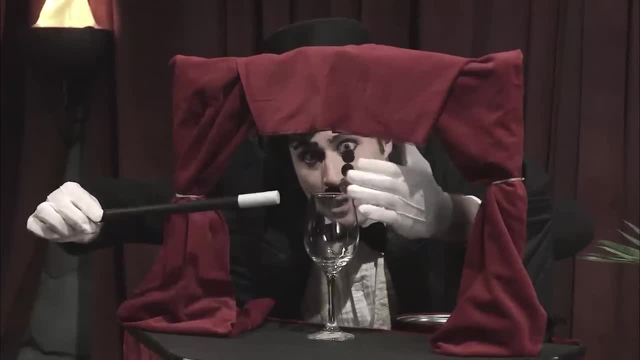 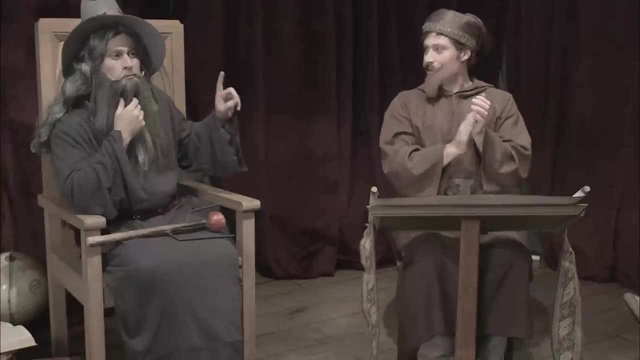 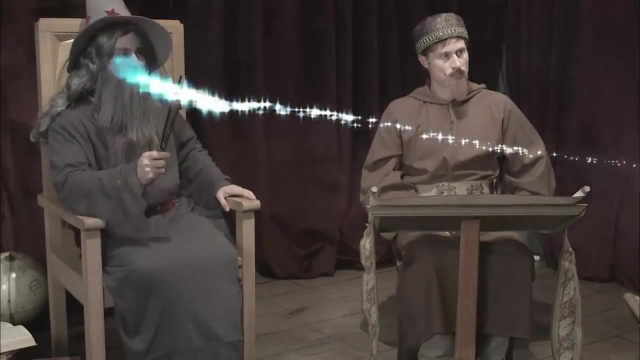 And now I say a magic word. A magic word: Ha, ha, ha ha. And now you must let me into your academy. Wait, What's under the cloth? What? What cloth? This cloth? Nothing. Oh, Is that a magnet? 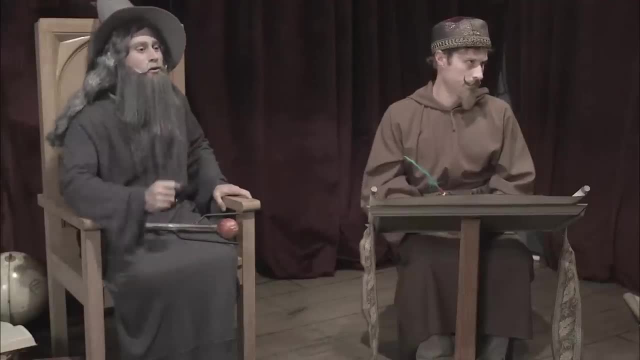 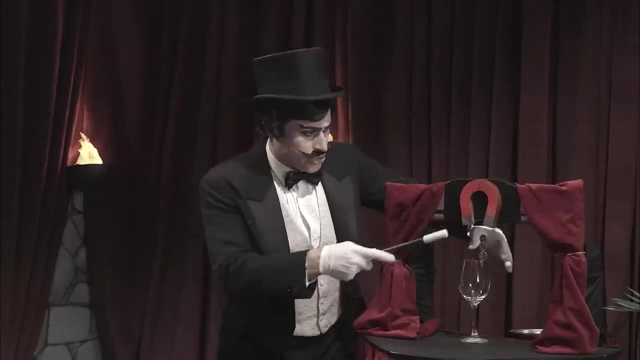 This. No, The pull of the magnet is what's keeping those coins up. The magnet is just strong enough to keep the coins from falling. No, This is set dressing, It's just pull. It was a good trick, But it's science, not magic. 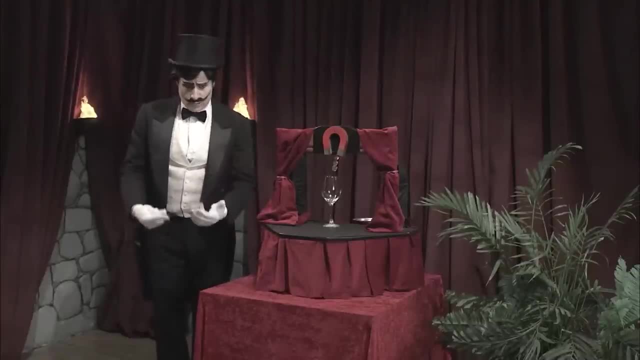 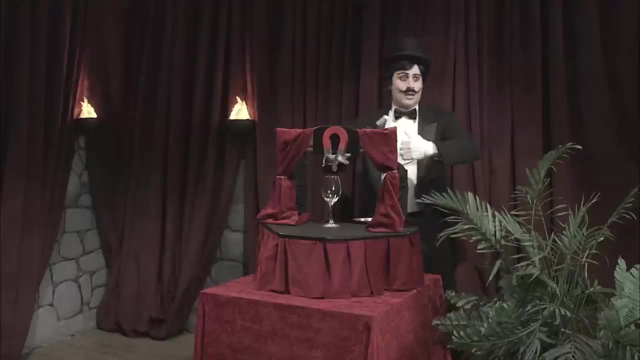 Well, yes, And you will see. You will see, I will see, I will see, I will be back. I, Overwhelmer, will return And I will do such magic that you will need extra socks, Because I will knock them off. 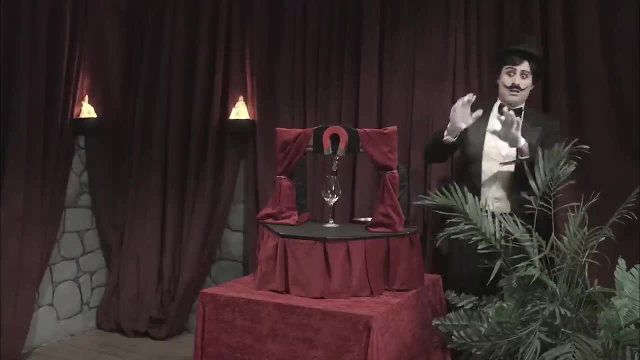 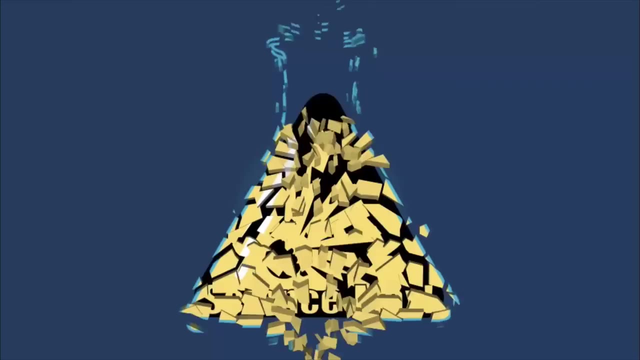 With my magic, you will need at least two pairs of socks, Maybe three pairs of socks. We can still see you. No, you can't. So back to our main experiment. Heather and I have created a very strong electromagnet that can hold a lot of power. 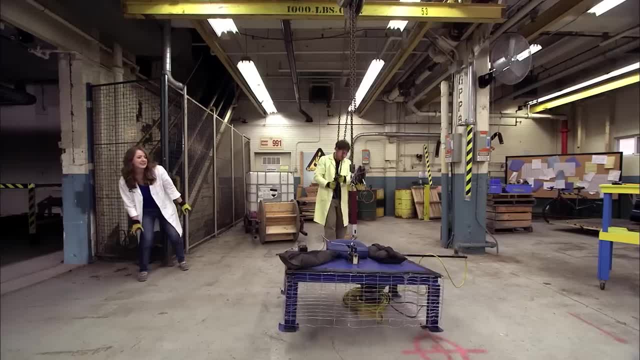 Heather and I have created a very strong electromagnet that can hold a lot of power. Heather and I have created a very strong electromagnet that can hold a lot of power. It held 100 kilograms, Oh, which gave me an idea. All right, you ready? 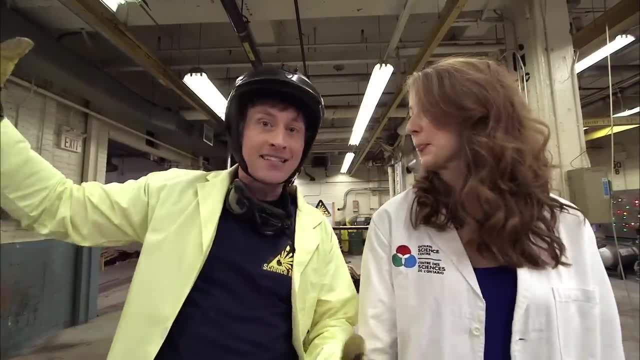 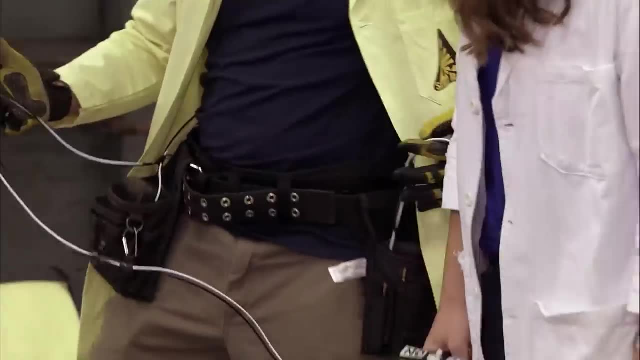 Let's do it. Electromagnets, super maxed out experiment. We've got two electromagnets, one, two, And those are wired to two batteries which are on my belt just like this, so that I can carry them around. 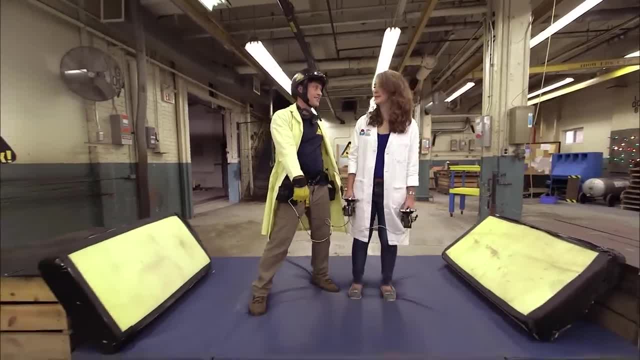 And we've got a crash mat here because we need to keep you safe, because you're going to be using these batteries, Because you're going to be using these batteries, because you're going to be using these batteries and we're going to use electromagnets to get across this massive beam above us. 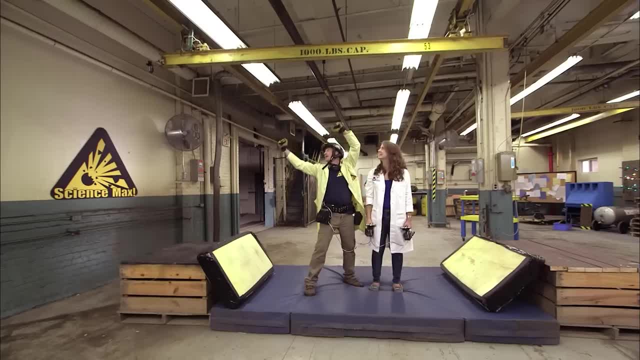 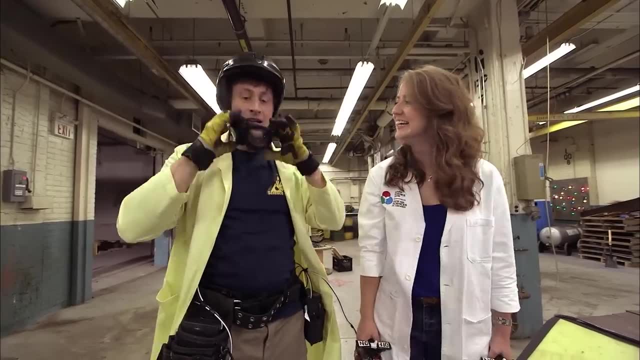 That's right. I'm going to stick to this metal beam and go across with the electromagnets. we hope I have faith. I'm glad you do. I've got a helmet for safety, goggles for safety, gloves for safety. 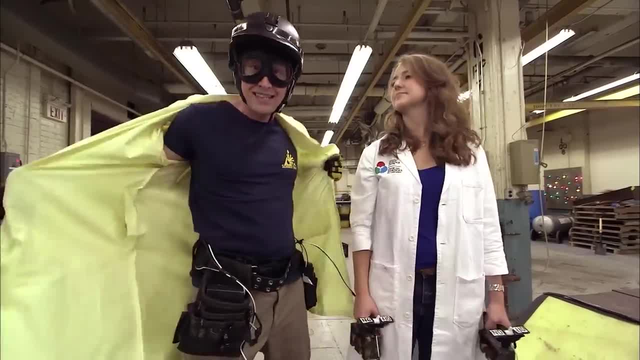 But in this case, sometimes the lab coat is more safe and sometimes it's less safe. This time it will get all caught up. so no lab coat. All right, you ready to go? I'm ready, Let's do it. 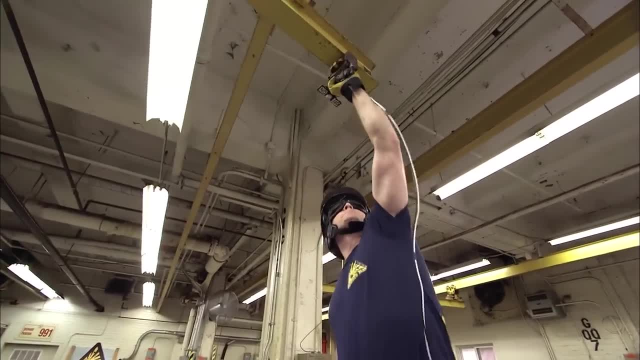 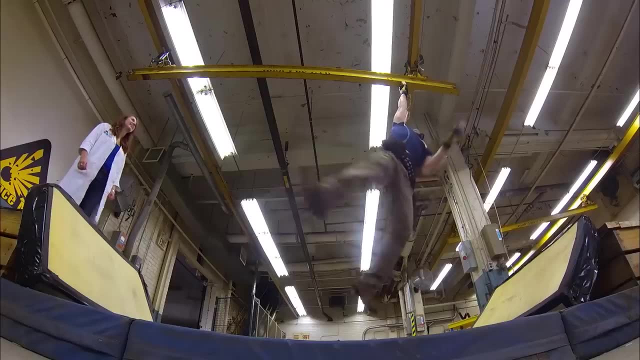 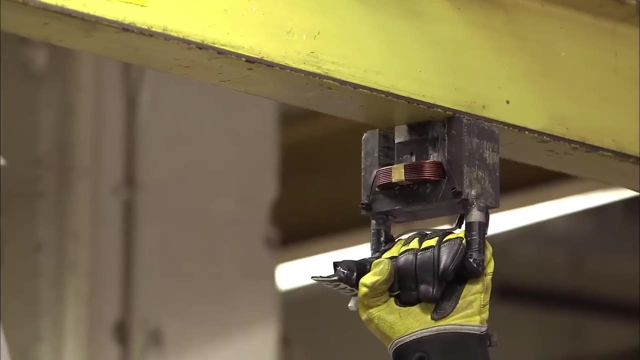 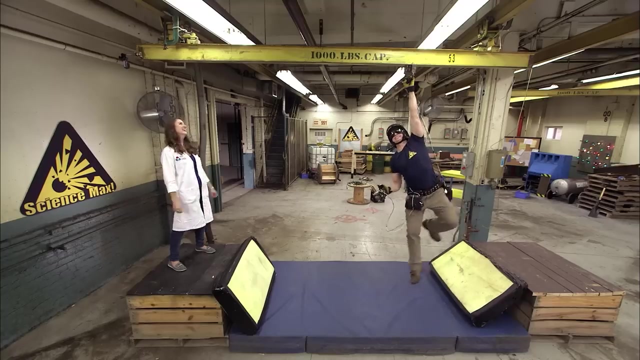 OK, Oh, my goodness What? OK, Because each of our electromagnets can hold more than my whole body weight. I can use them to cross the beam. When they're on, they stick like well magnets, And when I turn them off they stop being magnets. 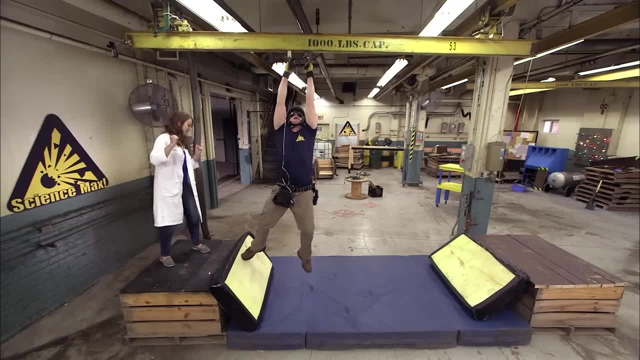 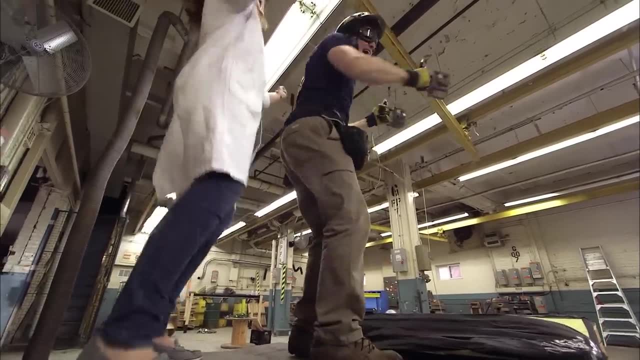 and I can move them along as I go. This is something you should definitely not try at home. Come on, Phil, You're almost there. Ah, Ah, Ah, Ah, Ah. We did it. Yay, Yeah, Woo. 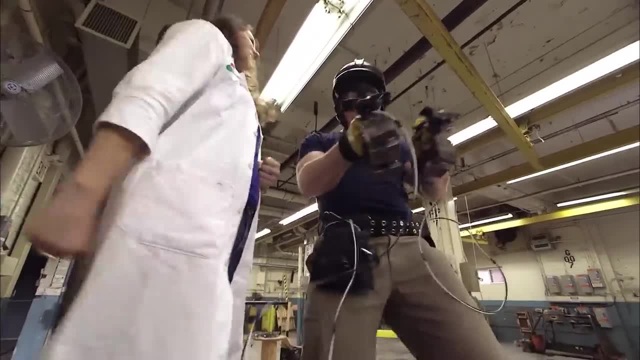 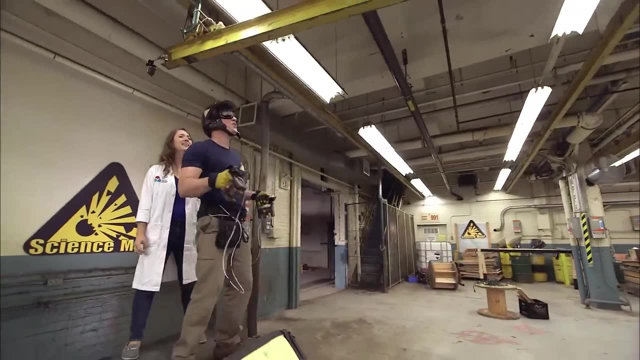 Woo, There you go. Science Max: Experiments at Large Electromagnets. Woo, You want to go. No, You sure I'm positive? OK, I'm going again. Woo-hoo, You're crazy. Science Max. 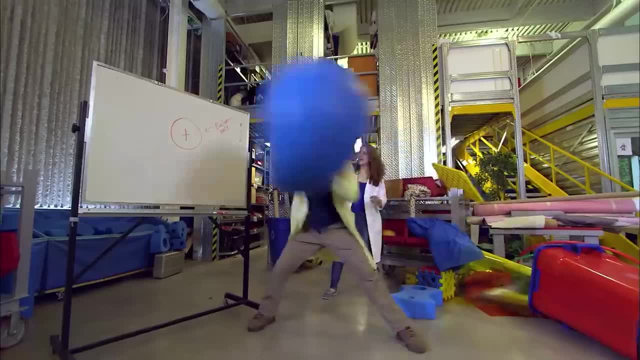 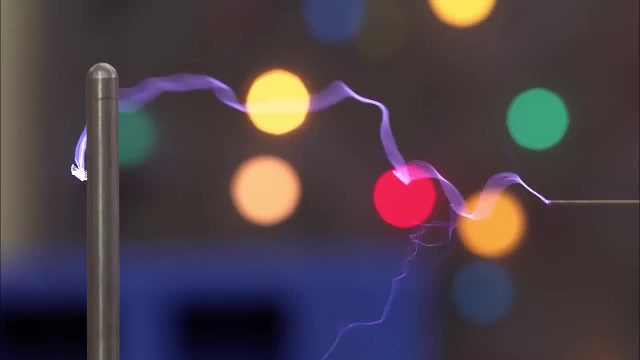 On this episode of Science Max. I'm on a quest to harness the power of light. Its balloon-sticking, hoop-levitating, hair-raising power is all thanks to static electricity. Hold on to your grounding rods, There's electricity in the air. 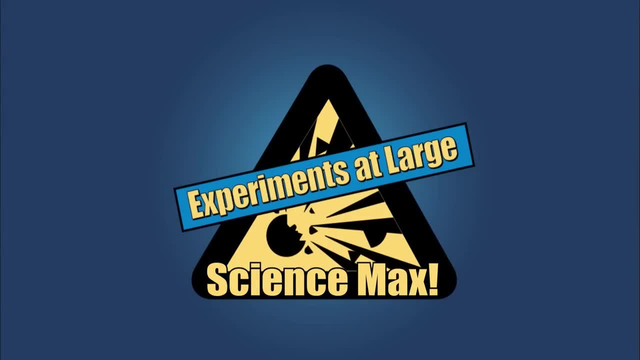 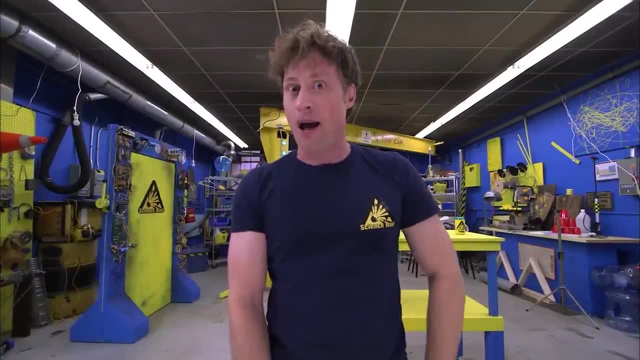 All on this episode of Science Max Experiments at Large. Greetings Science Maximites. Welcome to Science Max Experiments at Large. My name is Phil And today, on Science Max, we're going to be harnessing the awesome power of lightning. 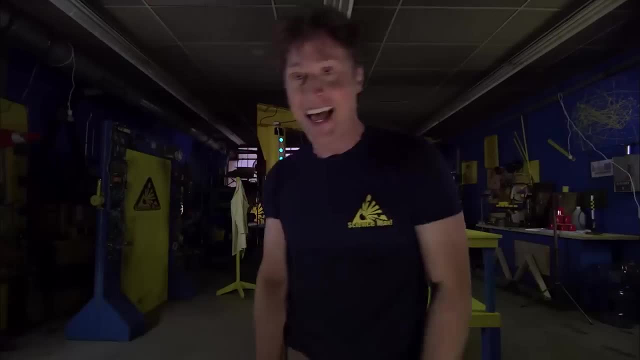 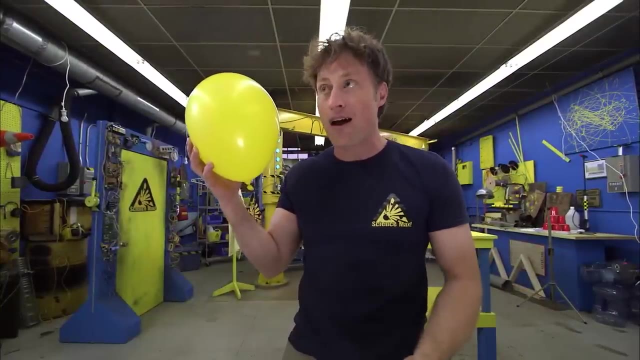 Wah, Ha, Ha, Ha, Ha Ha. How are we harnessing the power of lightning, you ask, With this balloon? I know what you're thinking. You're thinking, Phil. what's similar between a balloon and lightning? 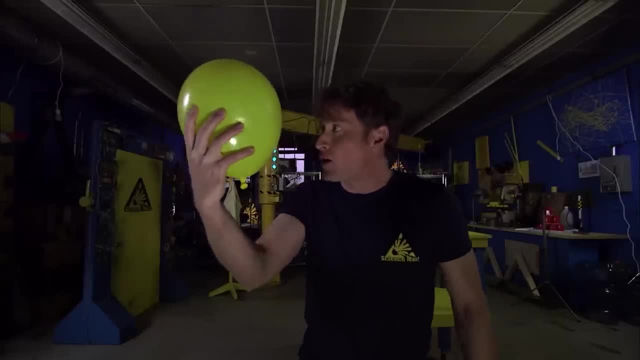 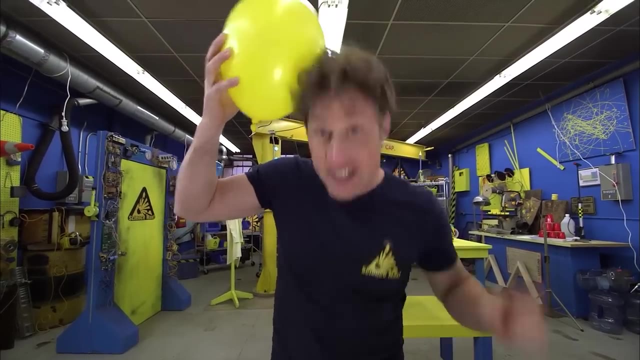 Well, nothing right now. But behold as I use the power of static electricity and rub the balloon on my head, Because basically that's how it starts. You see, when I rub this balloon on my head, it's stealing electrons from me. 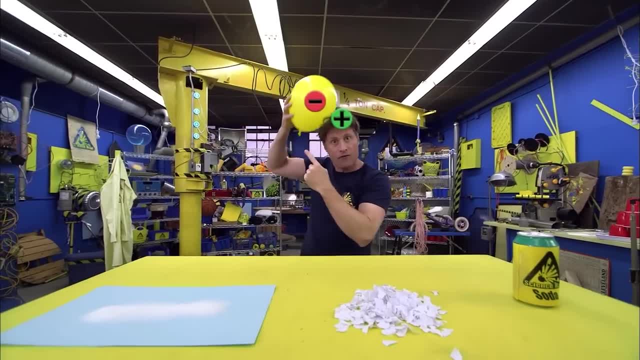 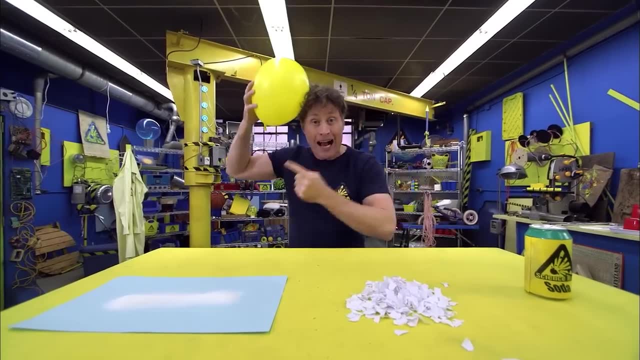 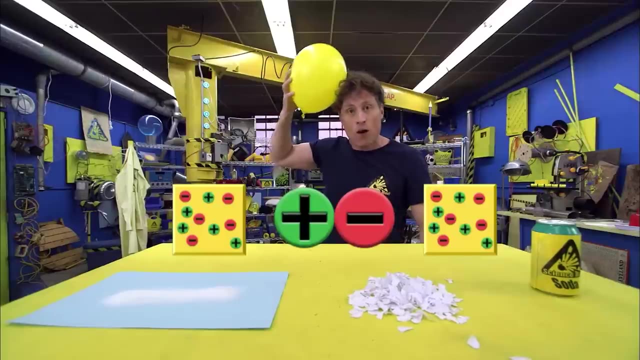 creating a positive charge in my hair And a negative charge in the balloon. And the interesting thing is you know that things with opposite charges attract each other. right, Something that has a positive charge will attract negative things, and vise versa. But anything with a charge will attract anything. 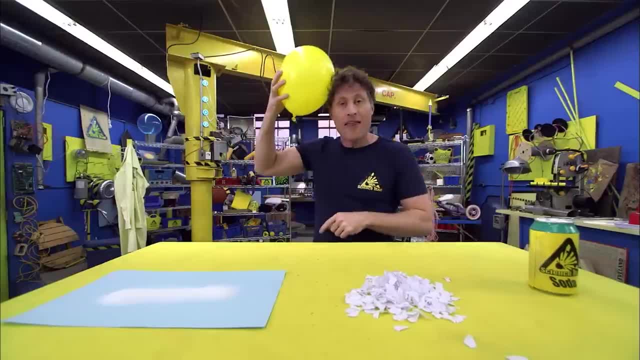 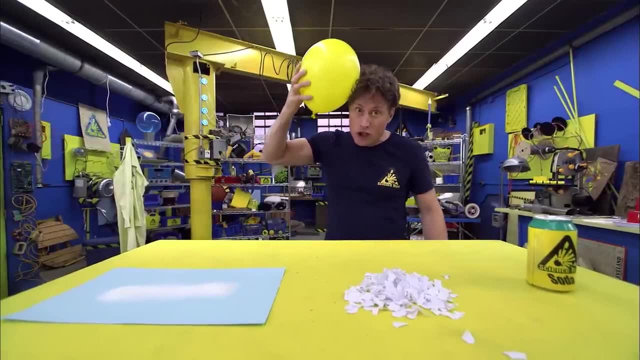 with a neutral charge. See all these things on the table. They all have a neutral charge, which means they've got equal amounts of positive and negative. Right now, this balloon is building up a big negative charge, which means it will be attracted. 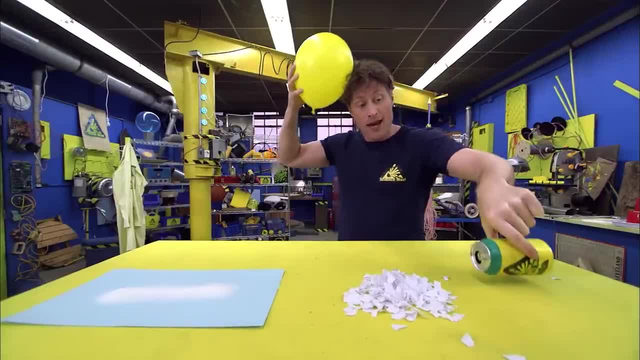 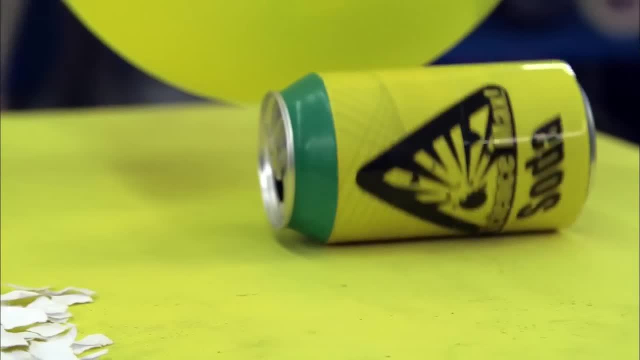 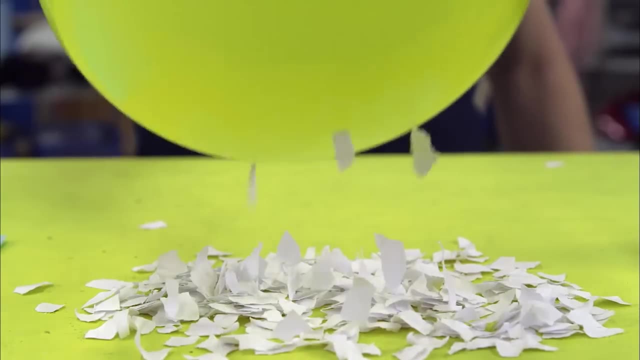 to all of these things. This can of Science, Max Soda. it has a neutral charge. The balloon has a negative charge, which means the can will be attracted to the balloon, And this paper is neutrally charged, which means the paper will be attracted to the balloon. 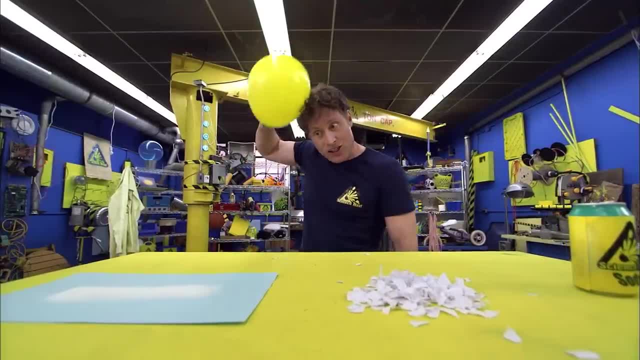 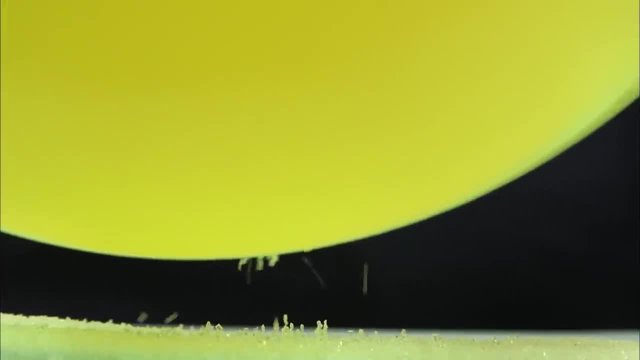 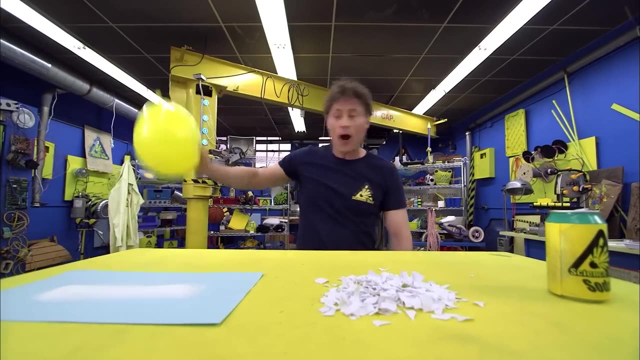 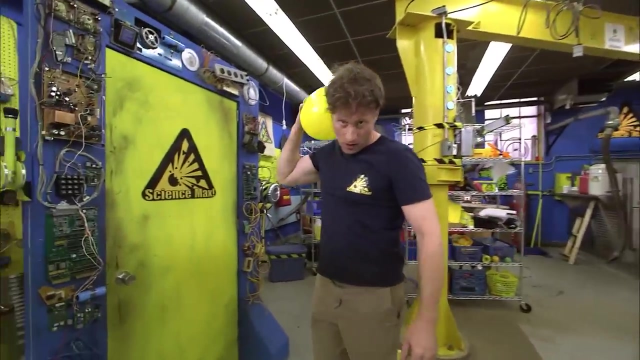 And if you hold the negatively charged balloon next to neutrally charged sugar, ha ha, sugar storm. And you probably wait. I don't want to get sugar in my hair- And you probably know this trick: If you rub a balloon on your head, you can stick it on the wall. 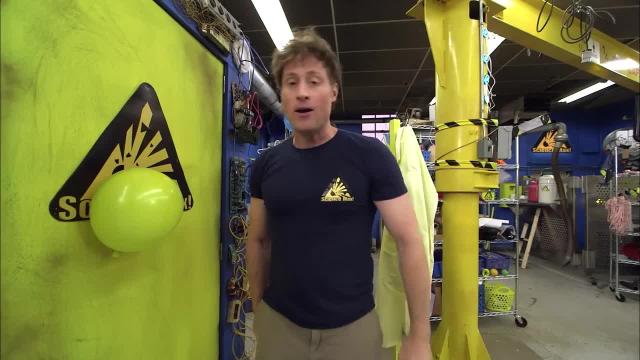 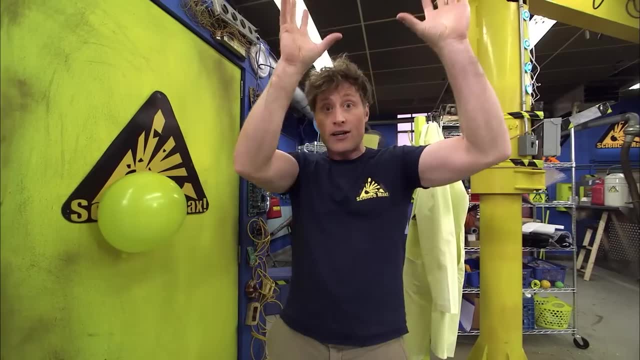 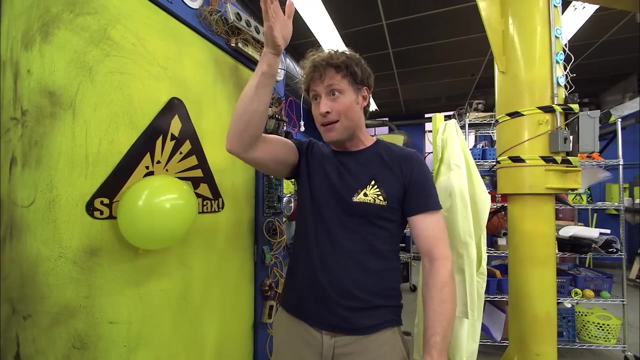 Ha ha. But what does any of this have to do with lightning? Well, the same thing is going on with a lightning bolt. The clouds become negatively charged and that negative charge wants to equalize itself with the ground, which is neutrally charged. and that lightning bolt. 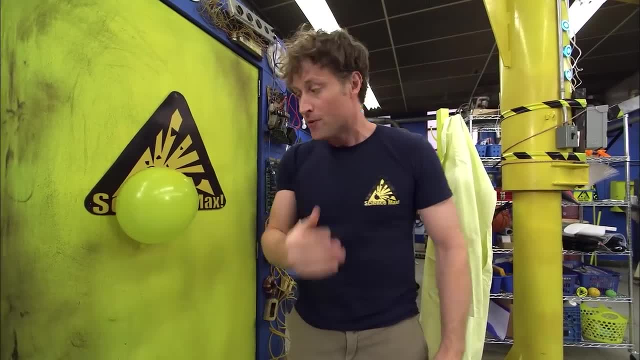 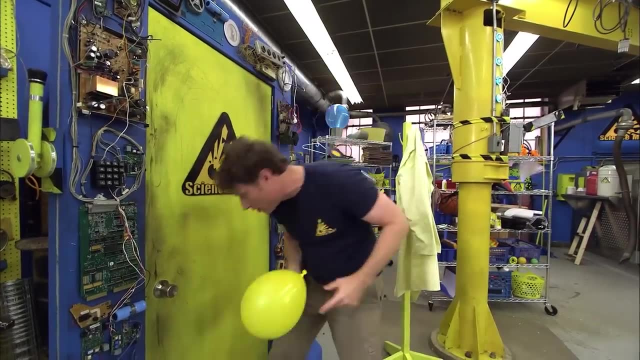 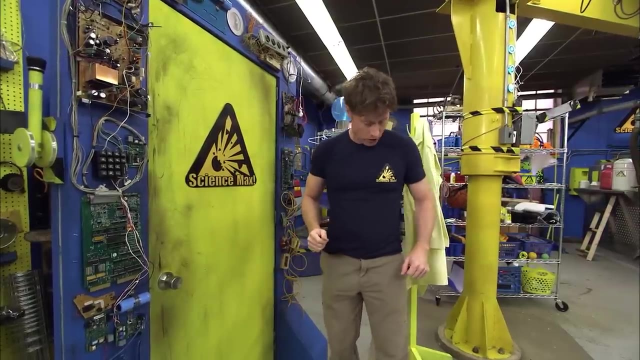 is the electricity jumping from one place to another, And you can see this yourself. If you rub a balloon on your head and you put it next to something metal, like a doorknob, there'll be a spark. But here's another thing you can do if you don't have a balloon. 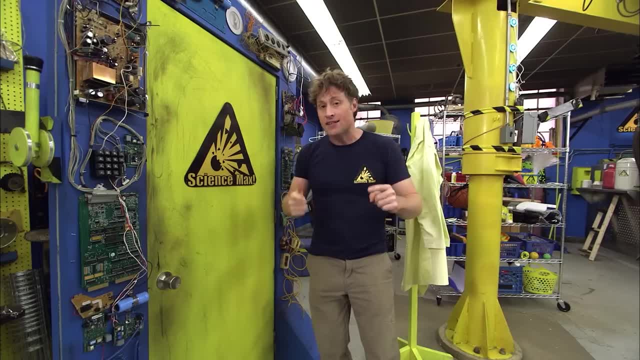 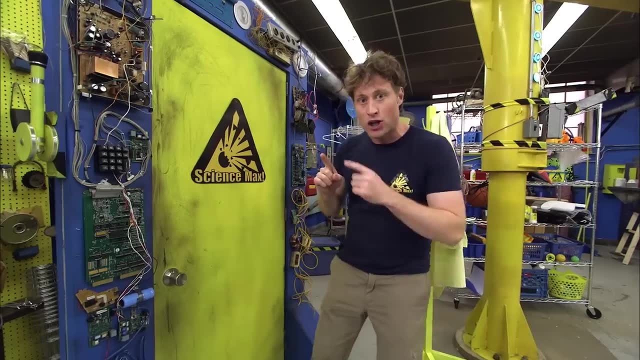 which I guess I don't anymore- Rub your feet. if you're wearing socks on a carpet and then turn out all the lights and touch a doorknob, you might not be able to see a spark jump from your finger to the door. 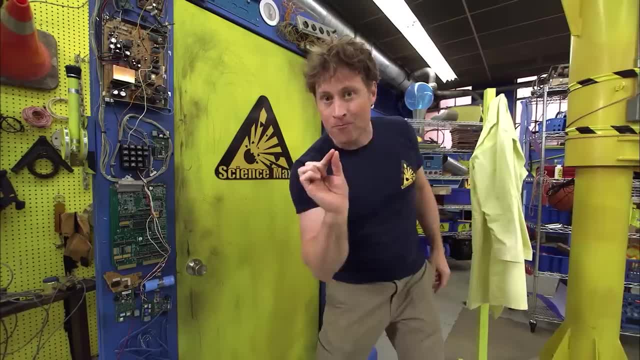 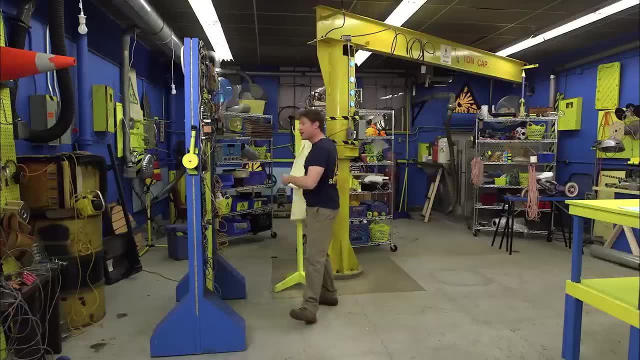 That's lightning in a very, very small form. So that's what we want to do today on Science: Max Experiments at Large, Max out lightning. I think I'm going to go to the Ontario Science Centre and ask Heather her advice. She really knows her stuff. 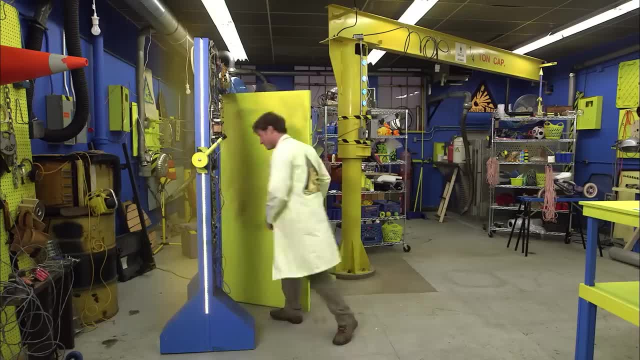 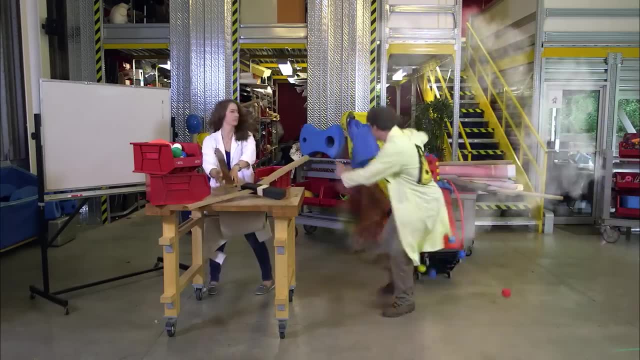 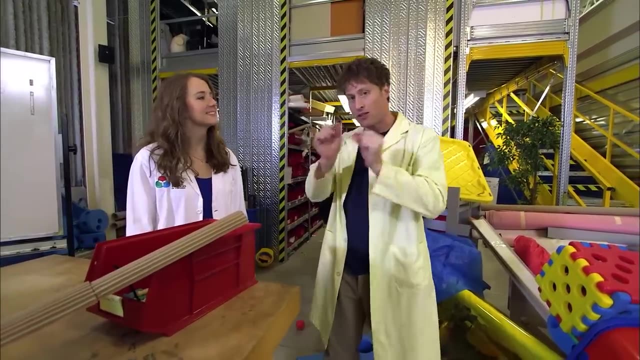 I'm going to go see if she's busy right now. Come on. Well, you got the portal fixed. so Well, it's not exactly fixed. It's still got a couple bugs that I'm ironing out, but I stopped coming in 10 feet above the floor. 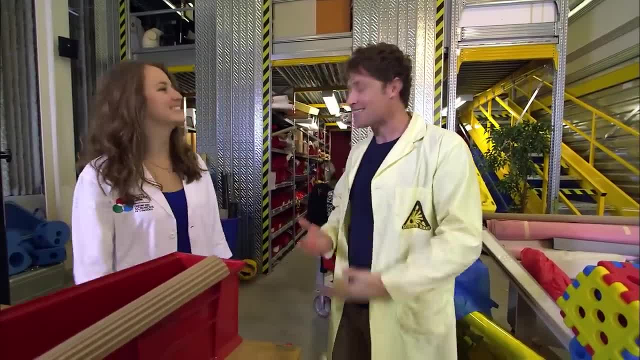 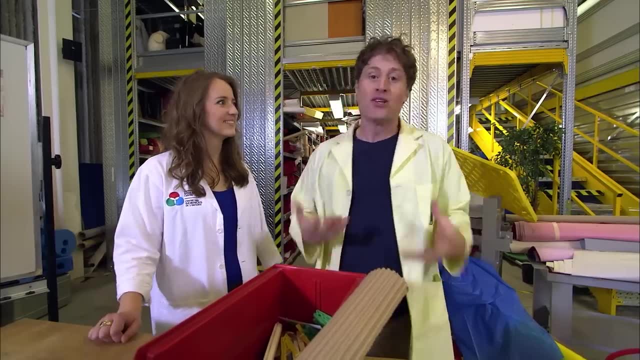 Hey, So that's a step in the right direction. Anyway, Heather, I've come here because I want to ask your advice on something. Yeah, for sure, Awesome. So what I am doing is creating lightning. So this is where I'm at right now. 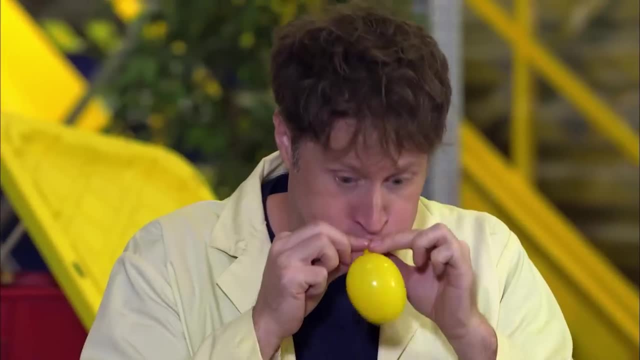 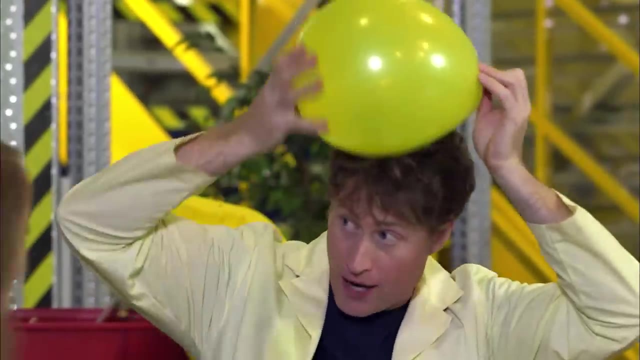 So this is a balloon. I blow up the balloon and then I rub it on my head. and I'm going to blow up the balloon. I rub it on my head and it creates a static charge. right, Right, yeah. 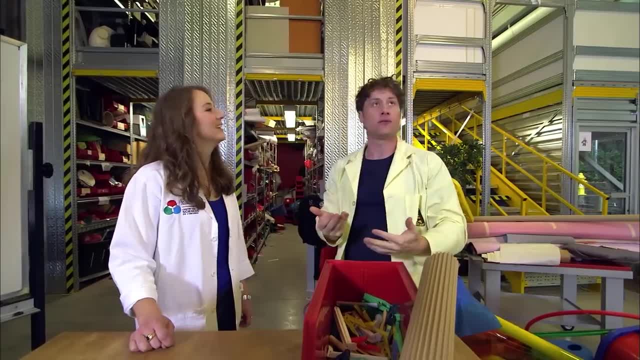 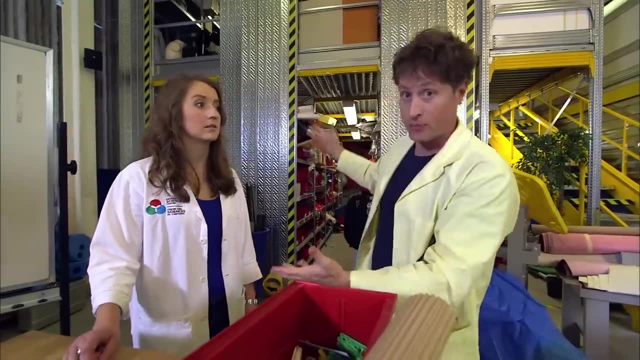 Just like in the lightning bolt between the clouds and the ground And the ground. So I was wondering if I was wondering if you could help me, maybe max that out. and I thought the perfect place to start would be a larger balloon. Ooh, right on. 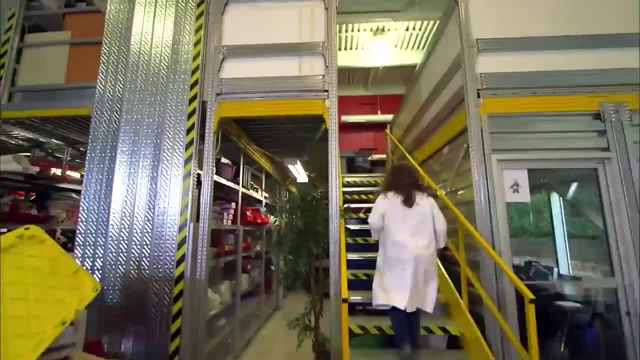 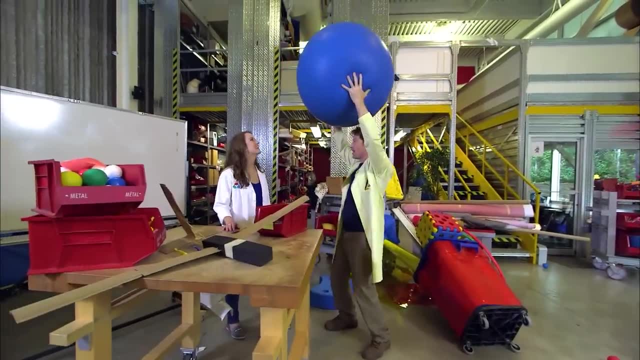 Actually, yeah, I like this. Yeah, I've got a big balloon. Can you just give me a second? Sure, All right, catch. Okay, All right, giant balloon. So what I figured is I'll just start rubbing it on my head. 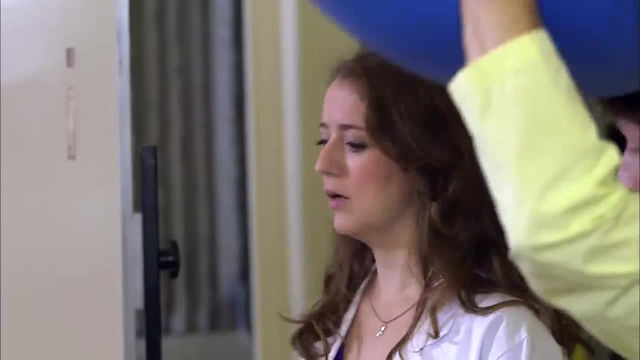 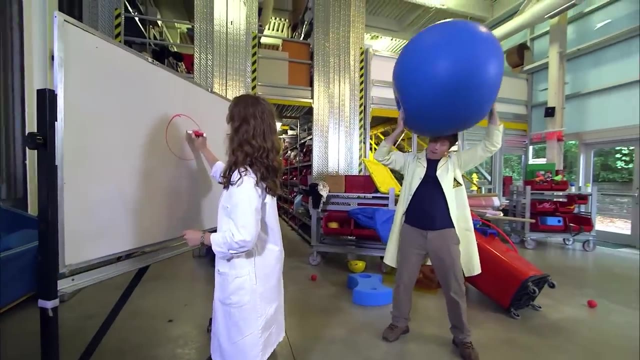 Okay, and then we could maybe stick it to the wall or something. Yeah, I think, instead of a wall, we can even try on this whiteboard here. Oh, okay, great, Keep rubbing. I'm rubbing, Okay, ready. 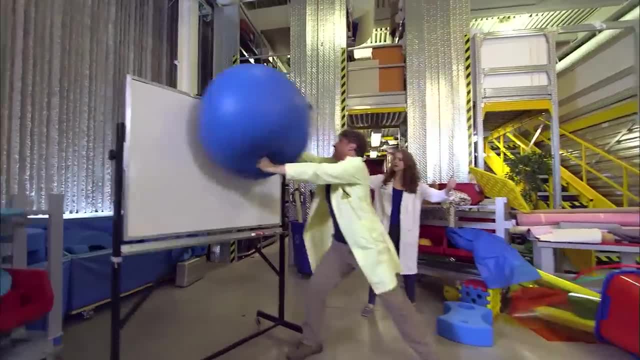 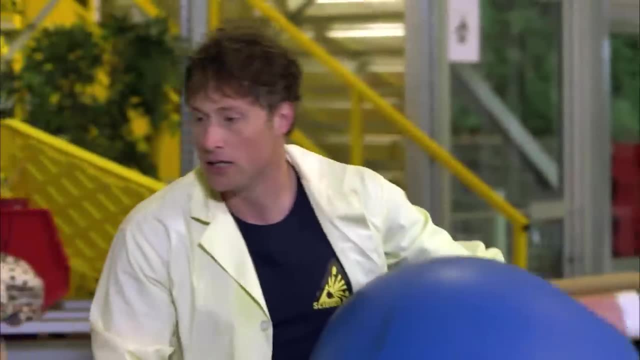 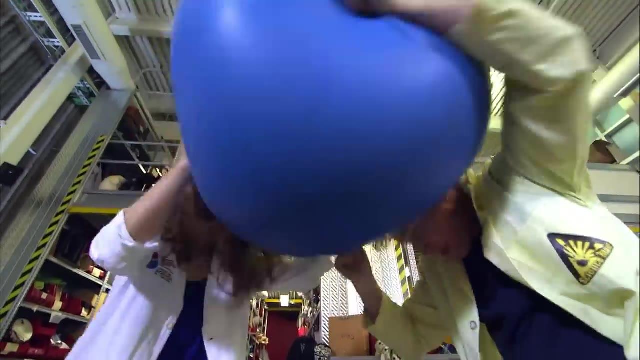 Yeah, Here we go, Give it a try, And So that didn't exactly work, Right? yeah, Both of us rubbing our heads on the balloon, Okay And Go. Wow, That was a whole lot of nothing. Well, we've got a really heavy balloon here, so 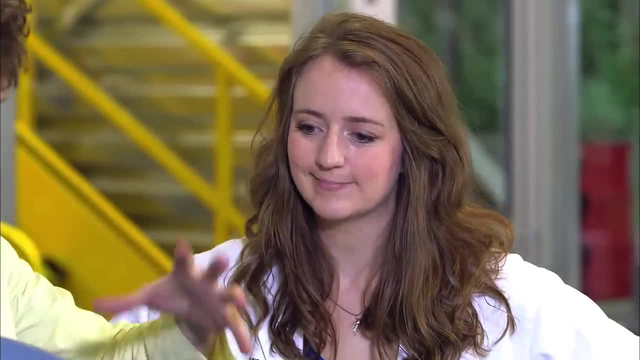 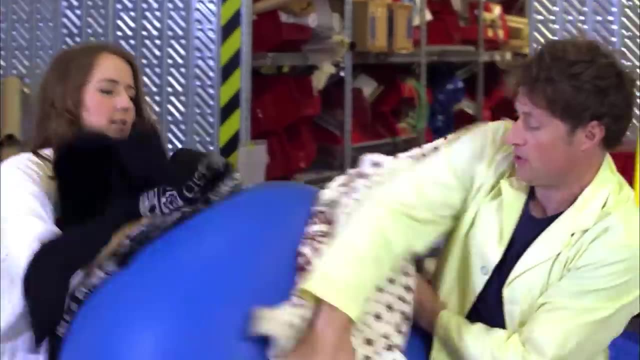 And I feel like our heads are only this big, so we can't cover as much surface area of the balloon. Fortunately, you can also build up a static charge by rubbing a balloon on a sweater or, if your balloon is giant, rubbing sweaters on your balloon. 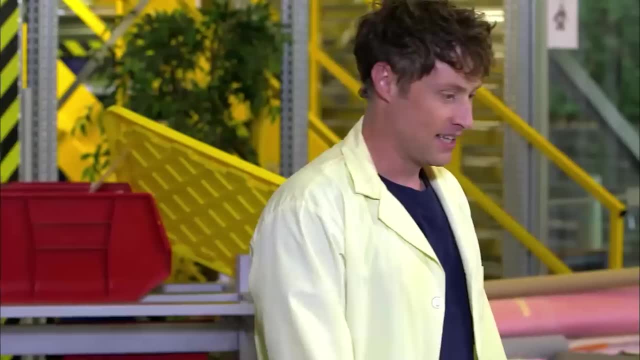 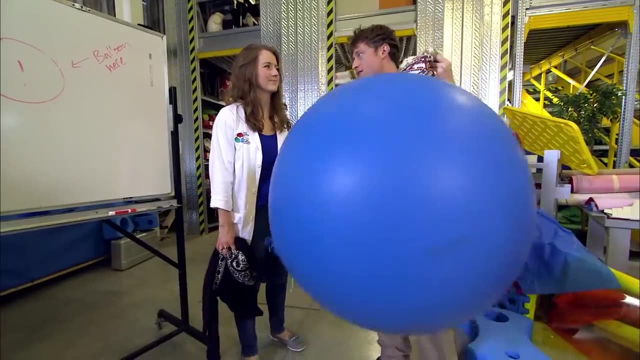 Yeah, But even that didn't work so well. I think what we need to do is come up with a better way to create a difference of charge. Yeah, yeah, Let's forget about the balloon. You have something else, I have something else. 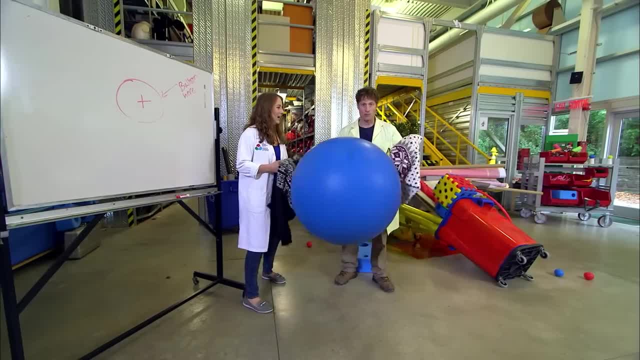 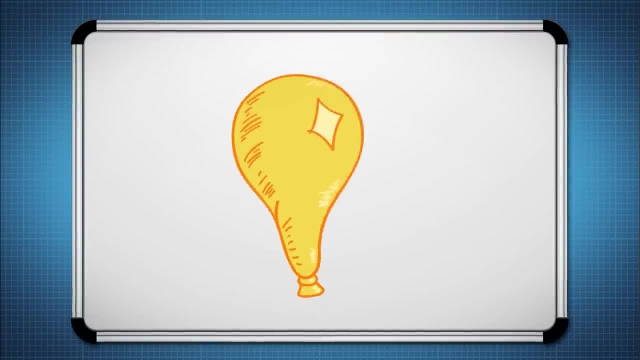 Really awesome here at the Science Center. You want to check it out? Yeah, absolutely. Yeah, right, Should we take the sweater and the balloons or should we leave them here? We'll leave them here, Okay. So here's how static electricity works. 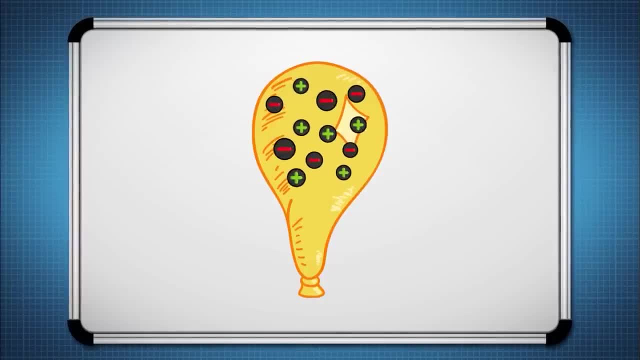 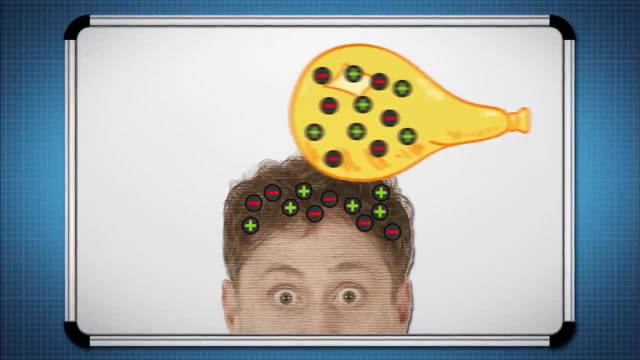 Normally everything has equal numbers of positive and negative charges. That's when things are said to have a neutral charge, But when you rub a balloon on your head, the balloon develops more negative charge than positive because it pulls electrons from your hair. 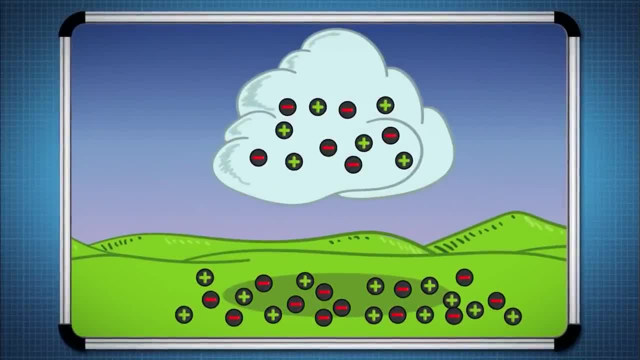 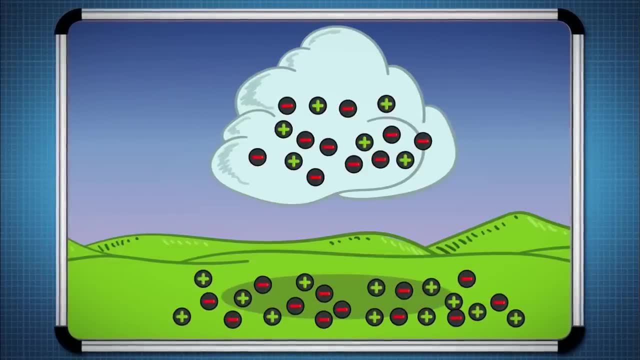 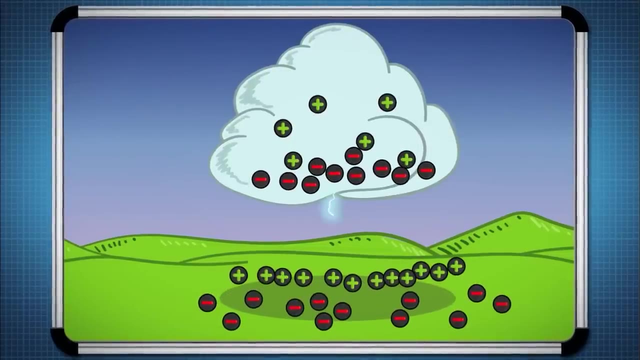 The same thing happens in clouds. during a storm, The cloud develops a negative charge. when water molecules start bumping into each other, A lightning bolt happens. when the negative charge in the cloud gets so big, the attraction to the positive charge in the ground gets strong enough that the electrons can make. 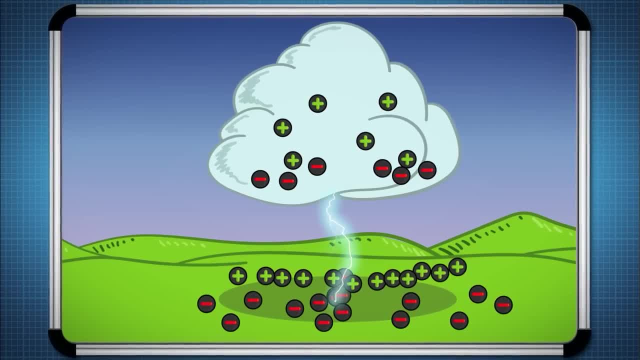 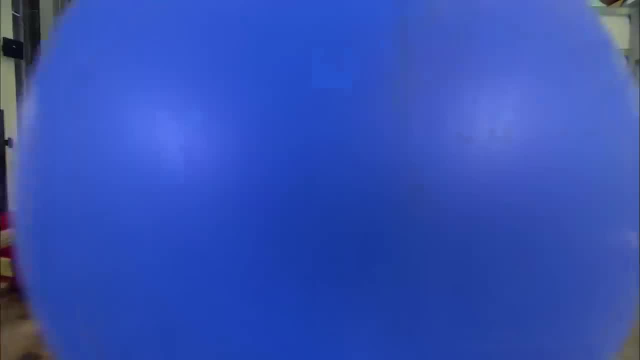 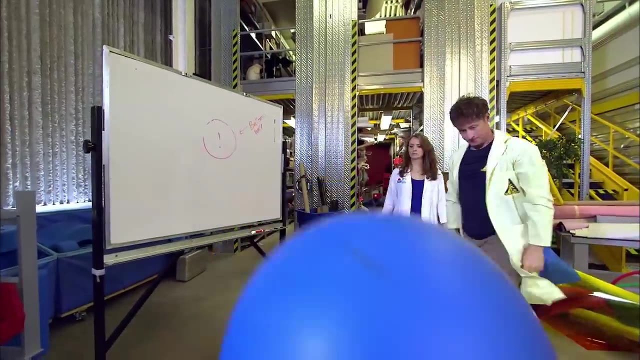 the jump all the way from the cloud to the ground and you get lightning. Heather and I tried to max out the static on a balloon, but a big, heavy balloon just doesn't hold the same charge. That didn't exactly work, Yeah. 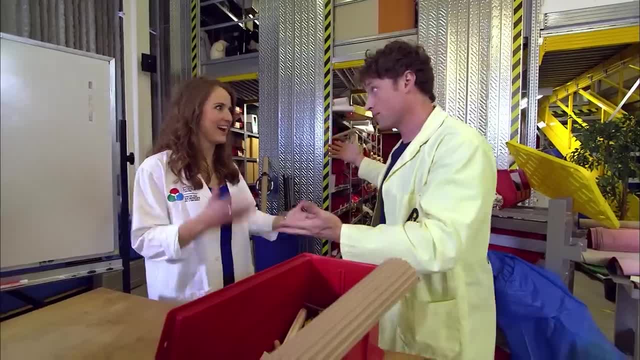 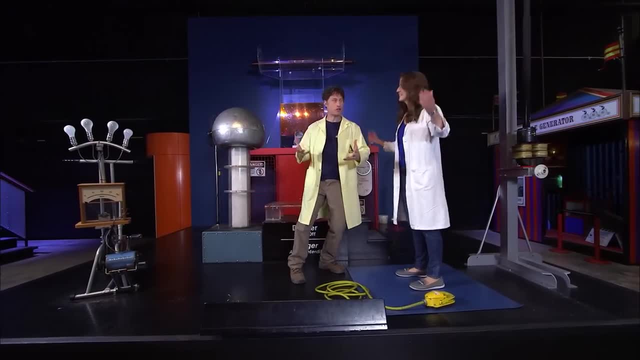 But we're only interested in maxing out the static charge, and Heather knows just what to use. Wow. So this is the Ontario Science Centre electricity show, Yes, Okay, so where's the electricity part? The one we're going to be playing with is right there. 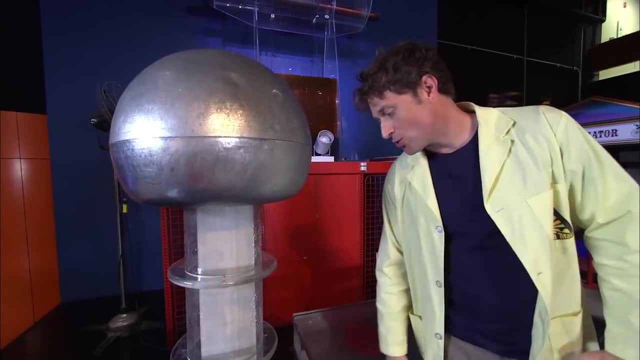 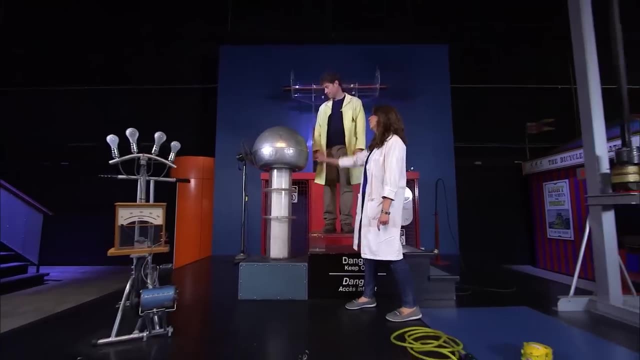 So the giant mushroom? Yeah Well, it does look like a mushroom. We're going to make some sort of electricity salad. All right, Head on up onto that platform right there, Okay, And I need you to put one hand on that silver ball. 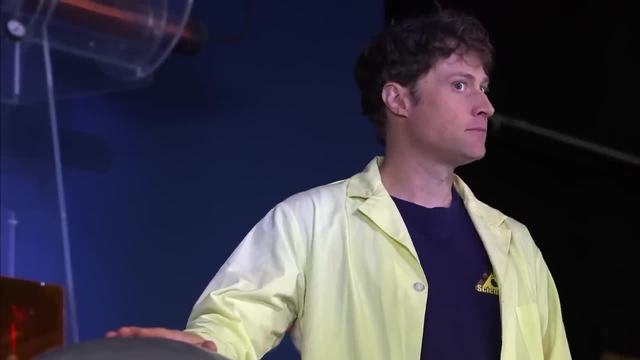 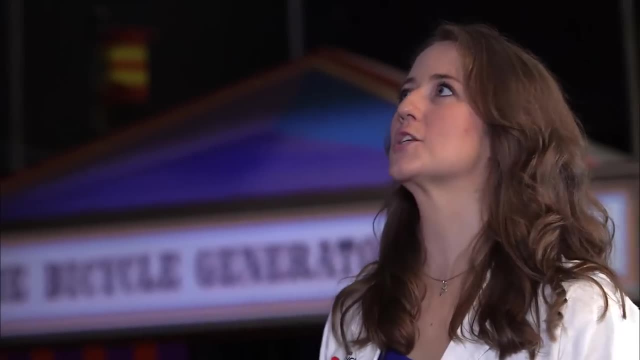 Yes, So the way it works, Nothing is happening. Patience, Okay, Once I turn it on, when I engage it, this is going to steal your negative charge, So it's going to steal your electrons. So if it steals electrons, you're going to be positively charged. 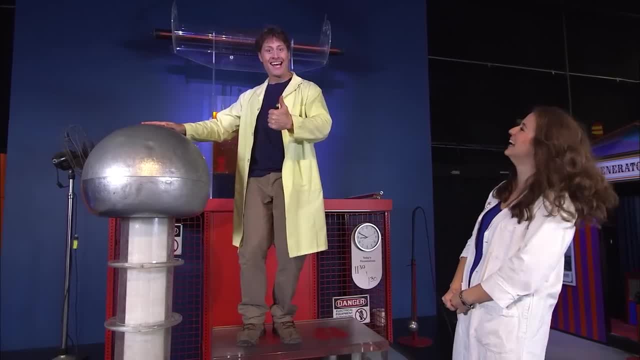 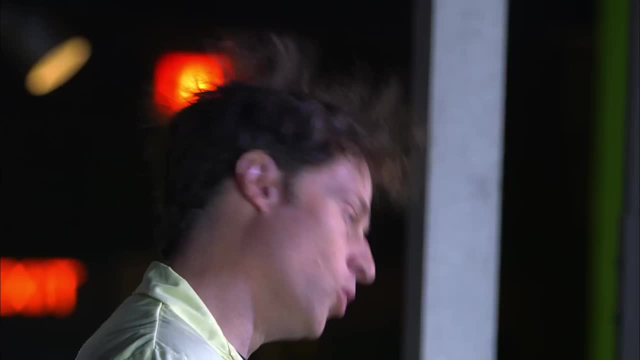 So it'll make me more positive, Even more positive. Yay, Woo-hoo, I am positive, Here we go. Woo. This machine is called a Van de Graaff generator and it pulls the negative charge away from the person touching it. 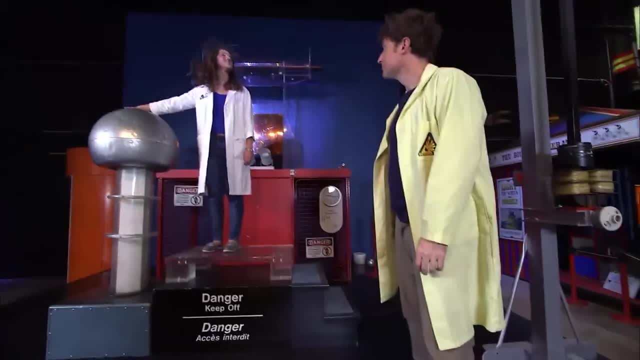 That is great. Instead of having equal amounts of positive and negative charges, you become positively charged. Woo-hoo, Science hair. Yeah, Like when you try to put two positive ends of magnets next to each other. each hair on your head starts to turn into a magnet. 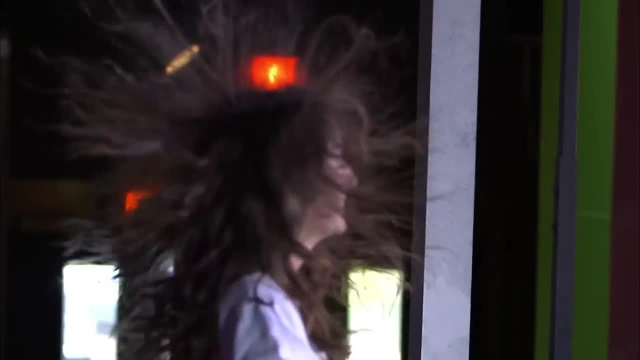 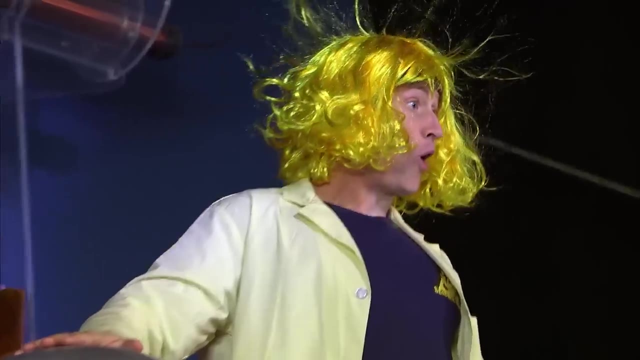 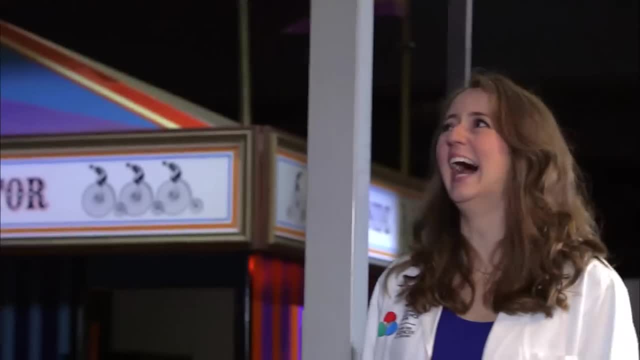 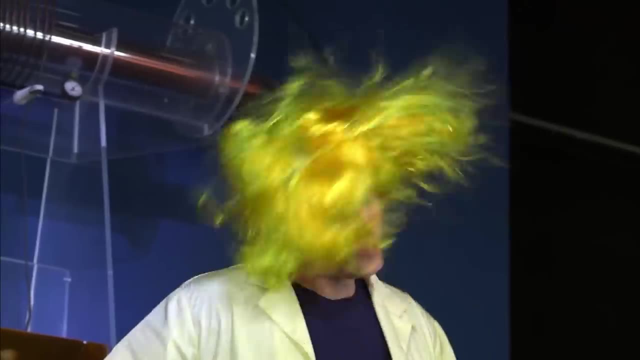 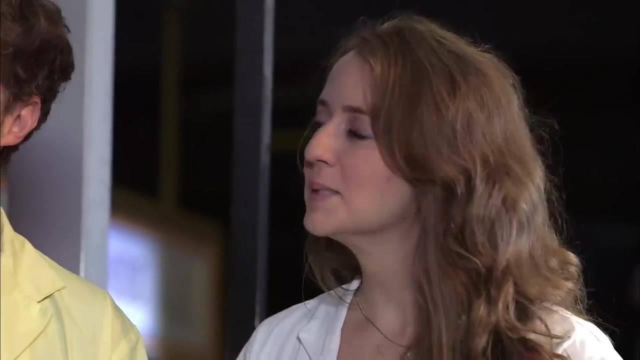 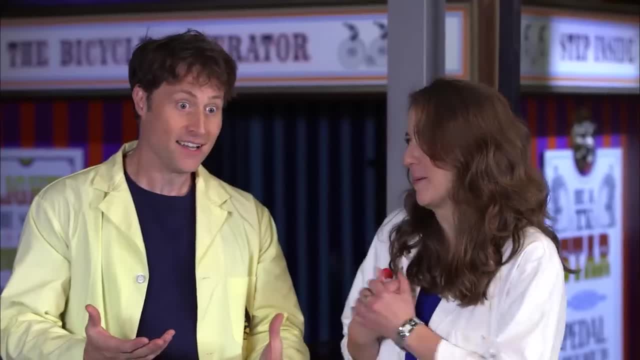 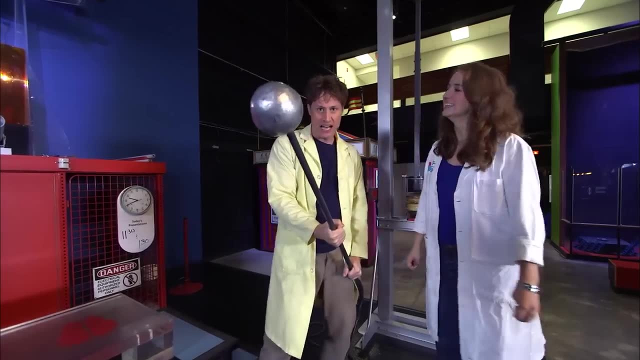 Oh well, actually I have a demonstration in my back pocket. This is going to help us, Okay, To create lightning. This is our grounding rod, It is my scepter of science, Science, And so we're going to use this to continuously provide that negative charge. 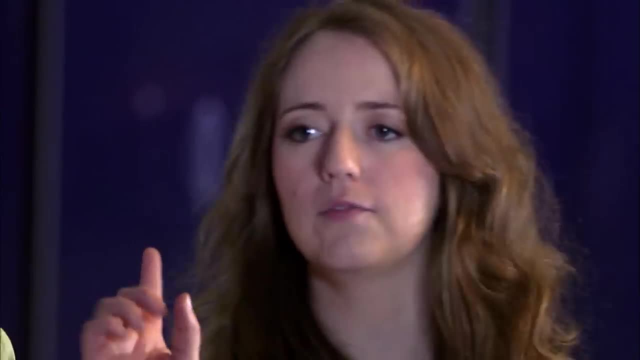 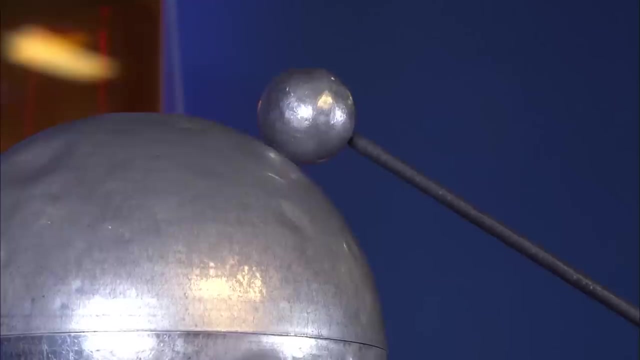 That's why it's plugged in. That's why it's plugged into the ground. Yeah, Okay, Okay. So then, if you touch it to that metal ball, got it not too exciting, right? So pull away and let's see what happens. 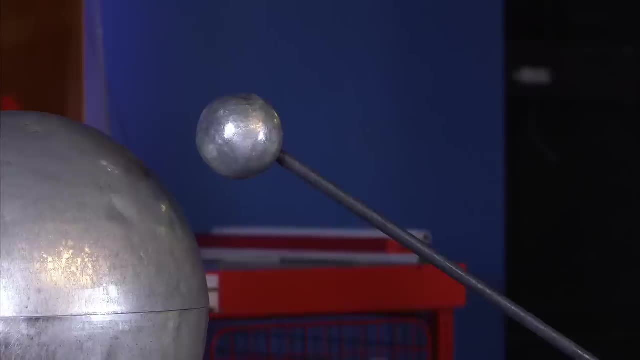 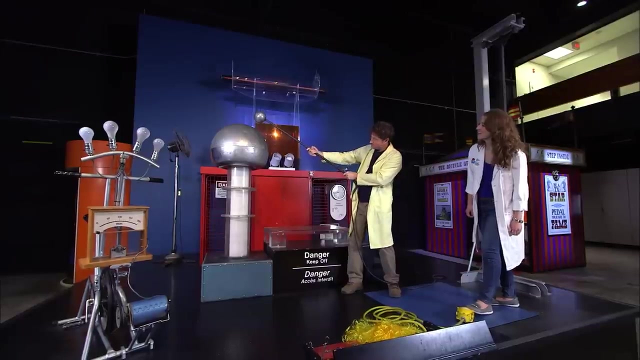 Whoa, This is what I'm talking about. Very good, The Van de Graaff creates a positive charge. The rod has a neutral charge. When the difference becomes big enough, the charge jumps the gap. Behold, I have the power of lightning. 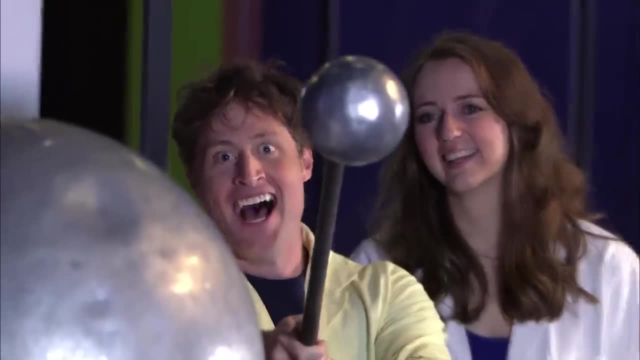 So it's the difference between the positive and the negative. is what we want. when we want to make a lightning bolt, Yes, So is there something we can use to make that happen? Large difference of charge: Yeah, I think I have just the thing. 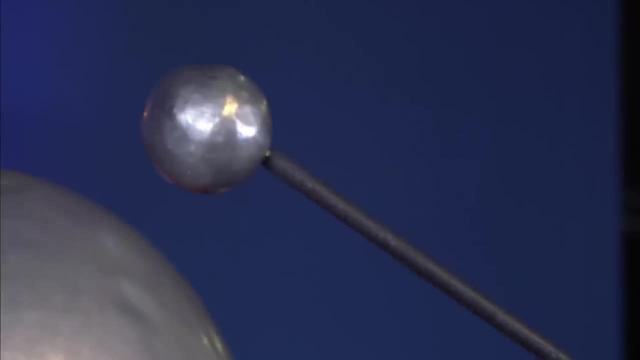 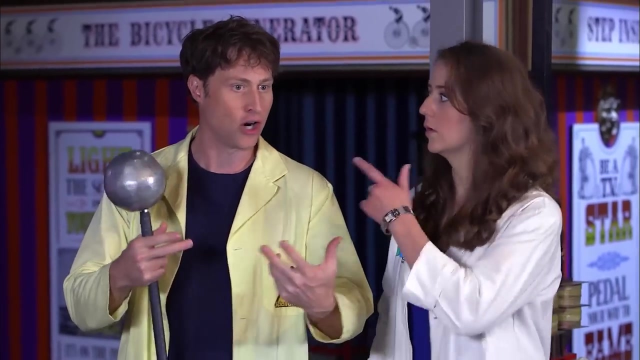 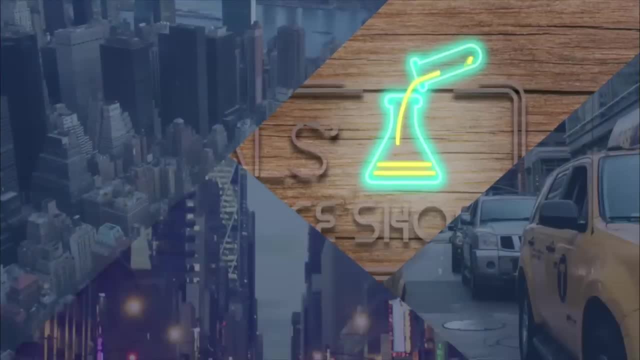 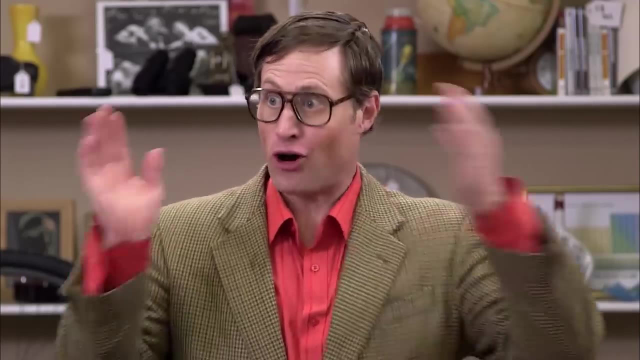 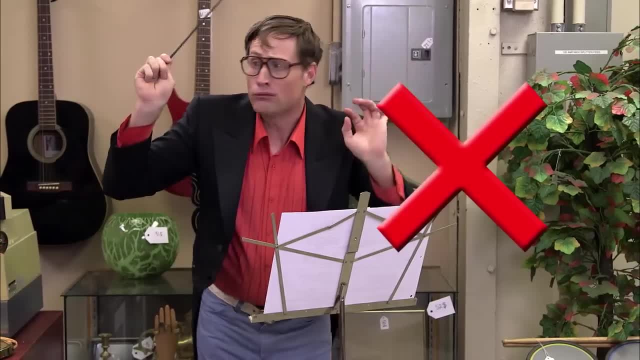 So do you want to do this? I'll get an electric wire. Okay Okay, You can pay, I'll go there, Okay, Okay. So you would like to move electricity from here to there? Well, what you need, my friend is a conductor. 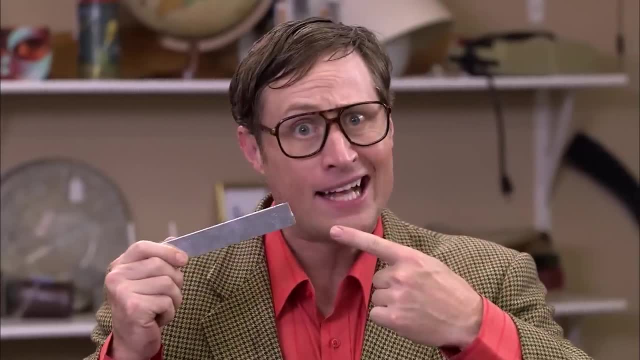 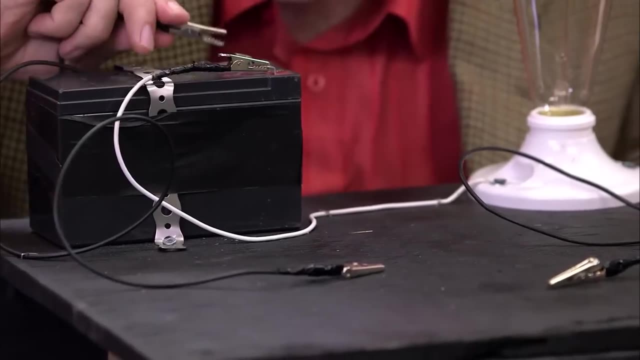 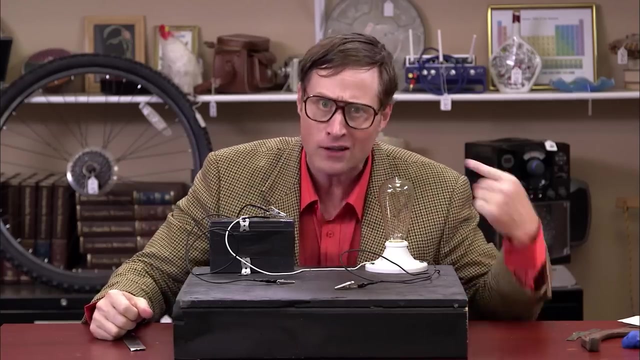 All right, A little more arpeggio this time. No, Not that kind of conductor All aboard. No, This is a circuit. Electricity flows from this battery along the wires and into the light bulb. But, Sal you cleverly observe, the light bulb is not lit. This is true. 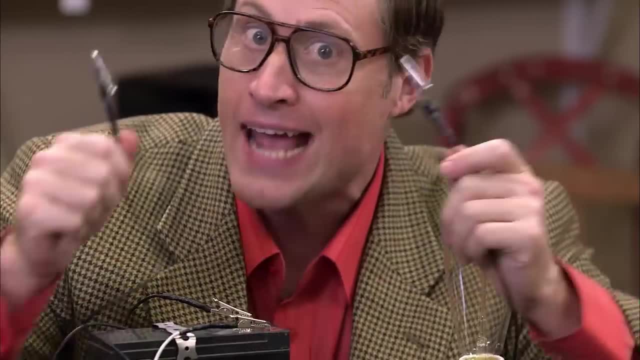 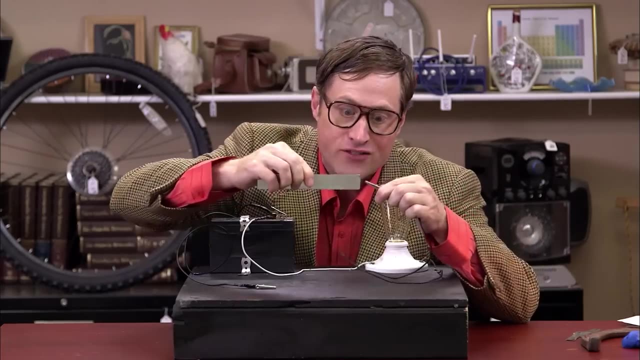 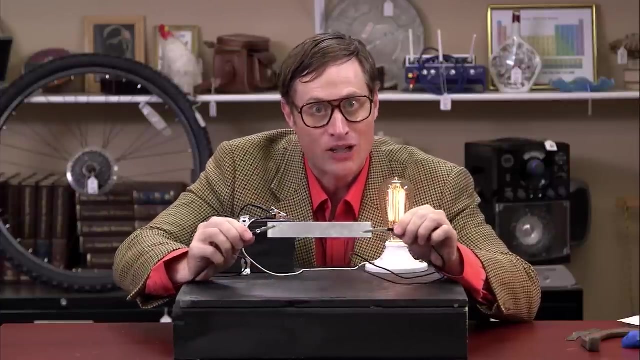 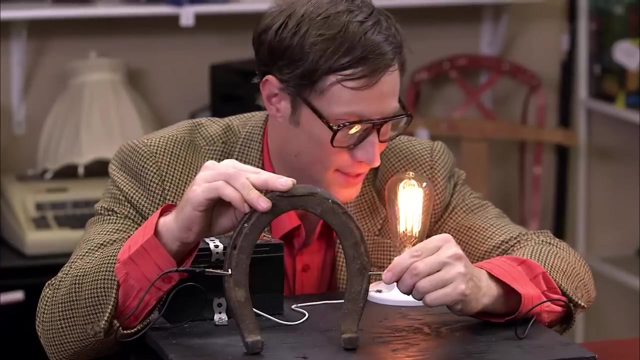 That is because we have a gap in the circuit and air is not a good conductor of electricity. Is metal a good conductor of electricity? Let us find out. Ha ha ha, metal is a good conductor of electricity. What about boy nope? What about this Horseshoe is a good conductor. will this sandwich conduct electricity? 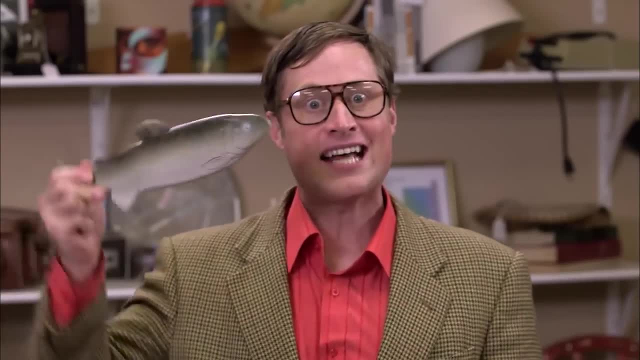 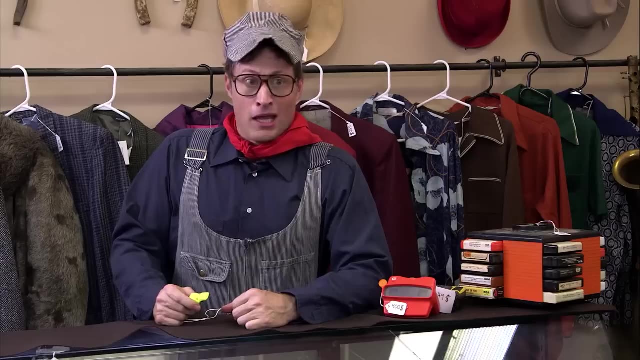 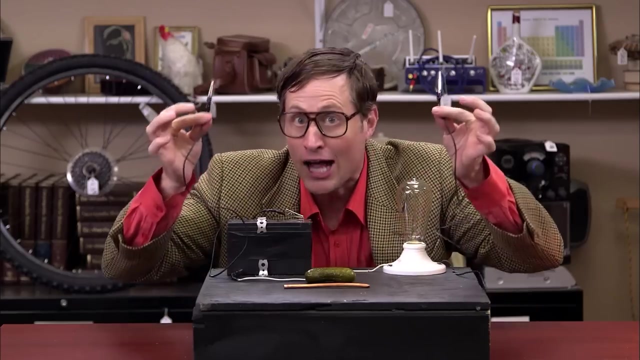 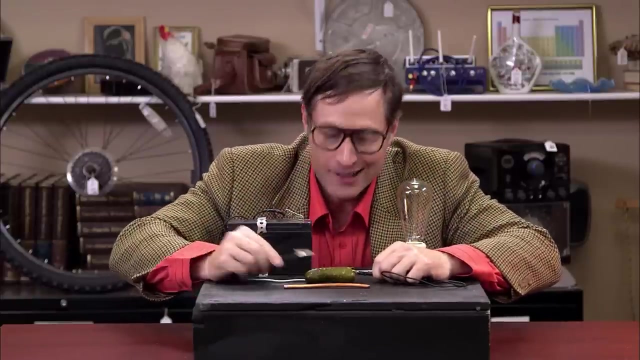 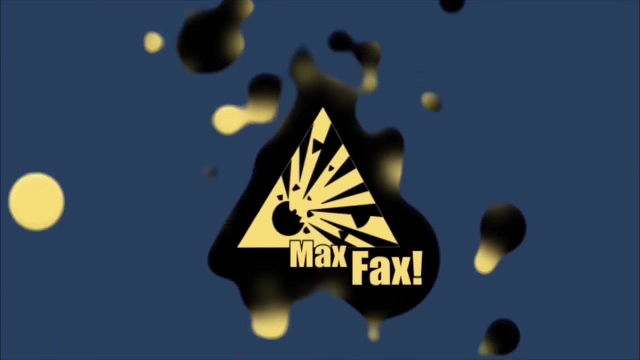 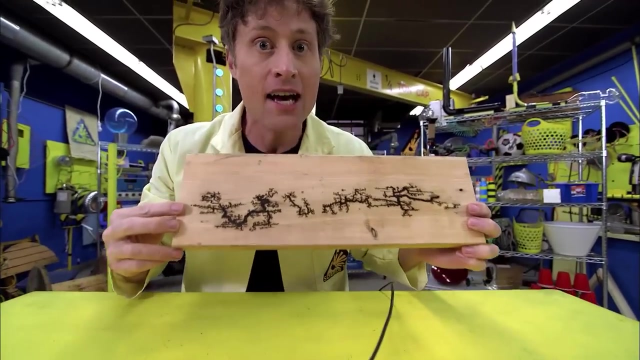 Nope. what about this plastic fish? Nope. What about this pickle? No, Pickle is not a good conductor. That's why we make electrical wires out of copper and not Pickles. you know, in case you were wondering, Lightning bolts make interesting patterns. That's because the electricity is searching for a way to get from one side to the other. 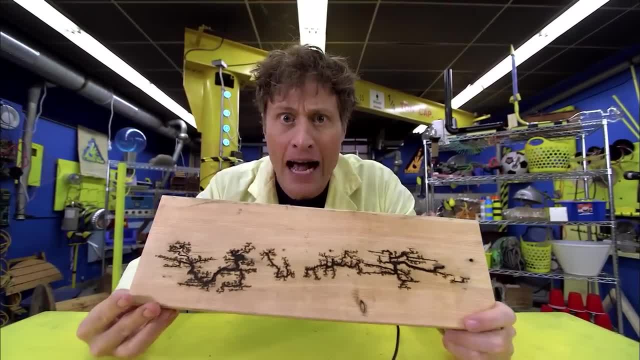 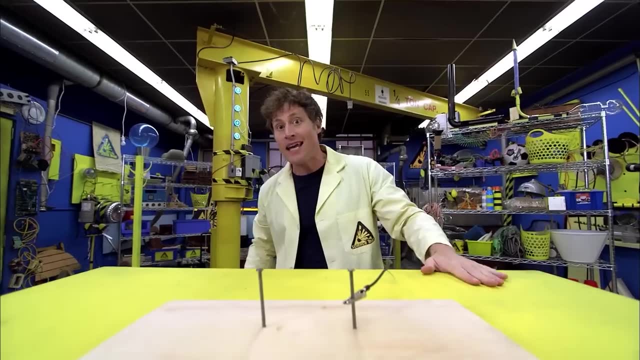 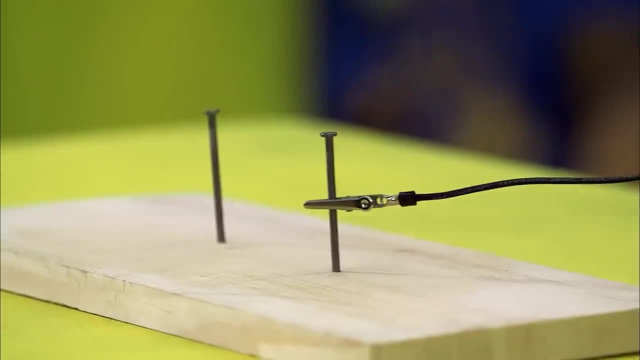 But it's hard to see The patterns of lightning bolts because they happen so fast. fortunately, using the power of science, We can observe these patterns for ourselves in a motion we can perceive. I'm going to use Electricity to recreate a lightning bolt pattern. I've got two nails in a piece of wood here and I'm going to attach. 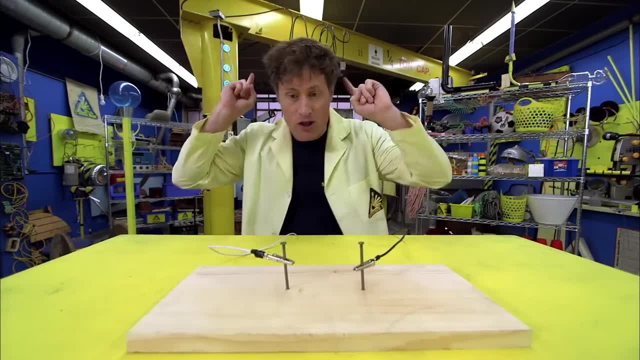 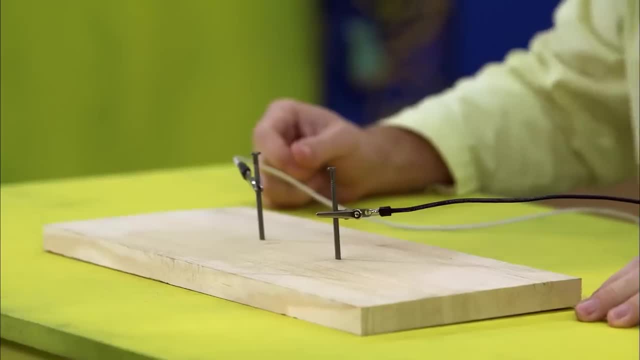 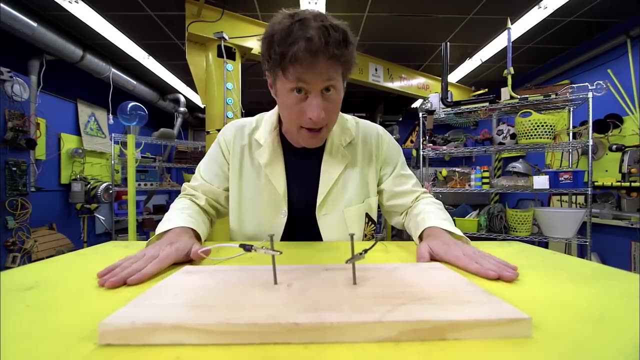 Electrical leads to both nails. now the electricity wants to go from that side to that side, But it can't. it has to go through the wood, and wood is not a very good condition. I'm going to use a special machine called an electric conductor of electricity. now, This is very dangerous. 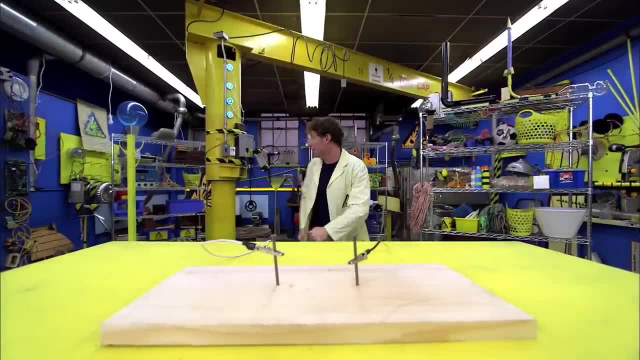 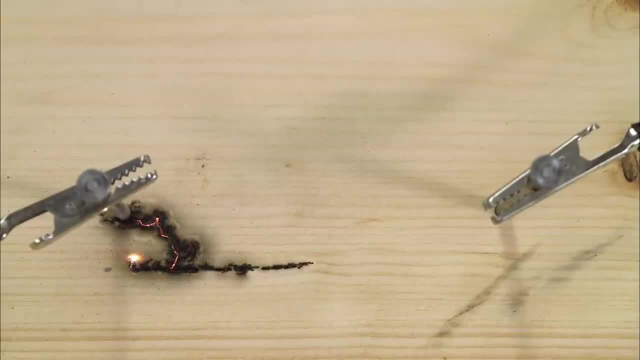 I need a special machine even to pull this off, So this is definitely not something you want to try at home. in fact, I'm going to stand way back here when I turn it on. Like water, electricity tries to find the easiest route to get from one place to another. 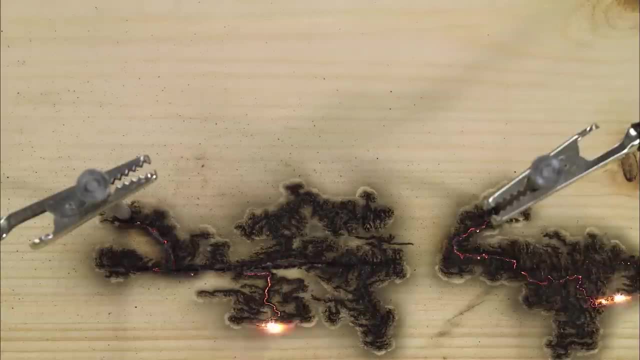 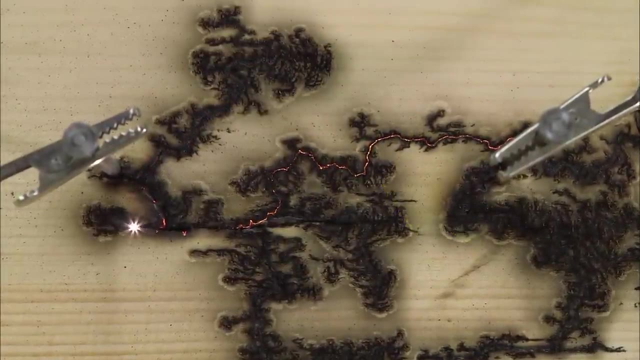 But sometimes that involves branching out until the right connection is made. Lightning bolts do the same thing. when they branch out between the clouds and the ground, there's a spot where the branches meet and the circuit completes itself. Then the electricity follows this one path, ignoring all the others. 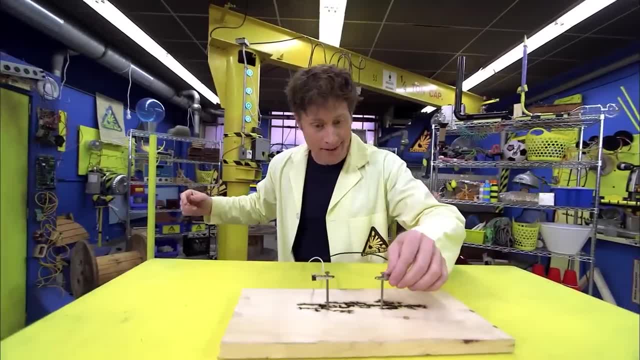 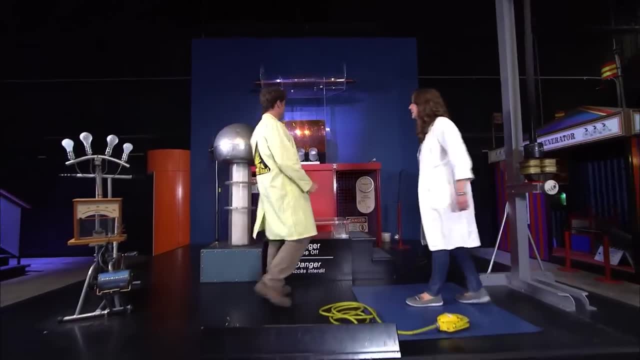 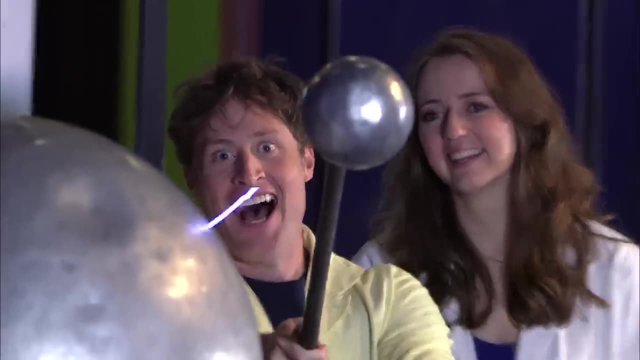 And there you go. We just watched a lightning bolt happen in slow motion. Ha ha, science. Back to our main experiment, where Heather and I are on a quest to use static electricity to recreate a lightning bolt: Our experiments with the Van de Graaff generator. 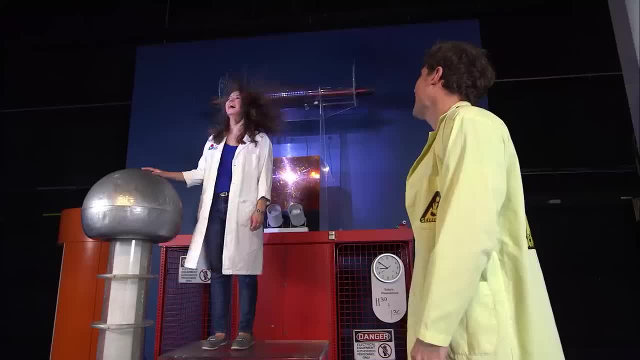 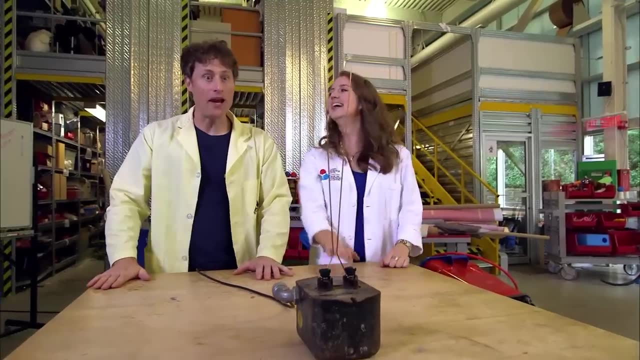 had some hair-raising results, but Heather has another experiment she wants to show me. This is Jacob's ladder. Oh, so this is another way to make lightning. Yes, Lightning. Let's see, yes, Let's do it All right. 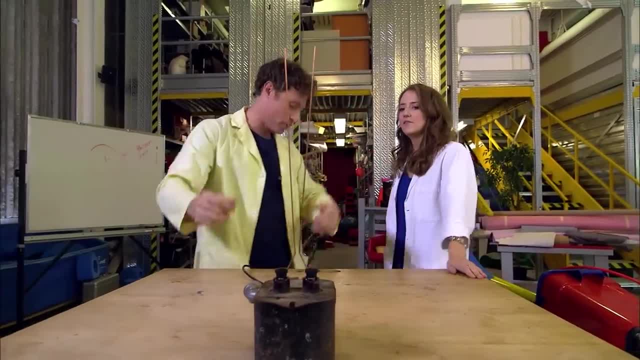 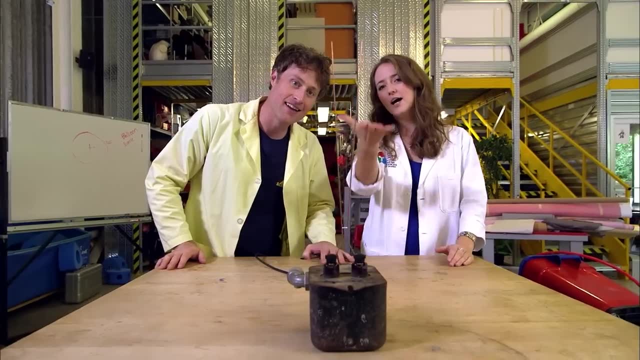 How do we get it to go? All right, so we want to turn it on. Behold, Oh, turn it on. okay, Go, Oh, Ooh. look at that. You can actually see that light climbing up between the two copper wires. 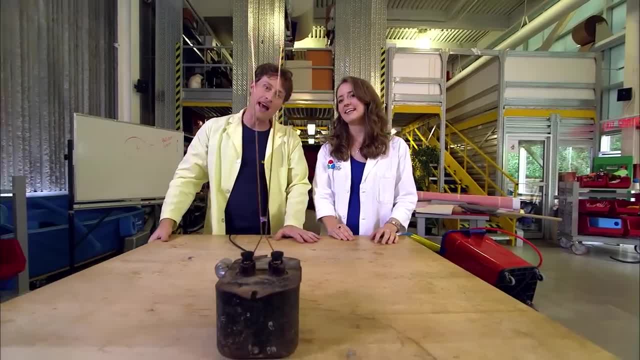 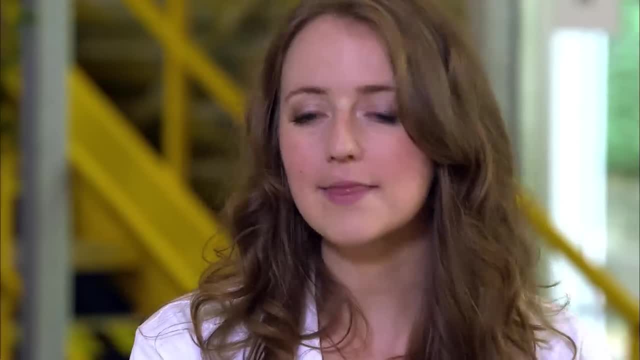 That's why you call it Jacob's ladder, because it's got the rungs of the ladder. Yeah, So at certain points there's a really great charge difference, right, Okay? so what's the difference? 10,000 volts, if you're looking at it. 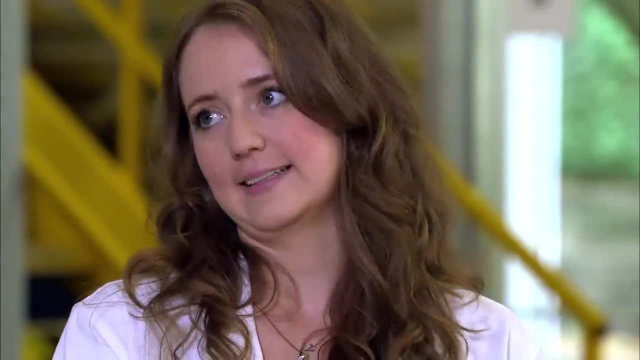 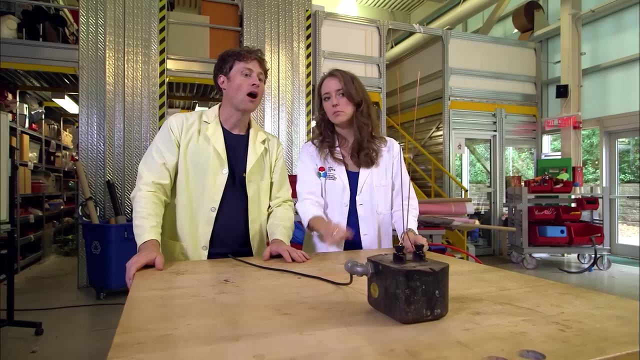 10,000 volts, And volts is how you measure the difference in charge Exactly. Why does it go up? So it goes up because, rather than just staying at the closest point, is because we're heating up the air. Oh, so hot air rises. 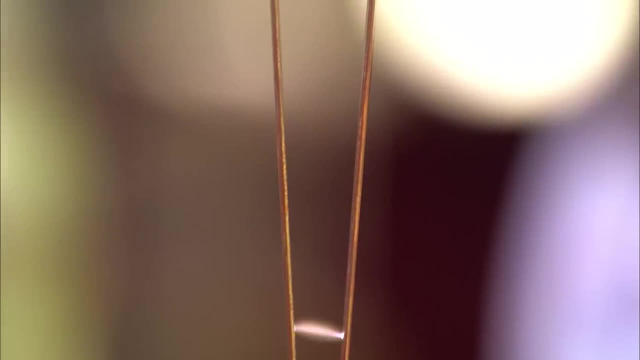 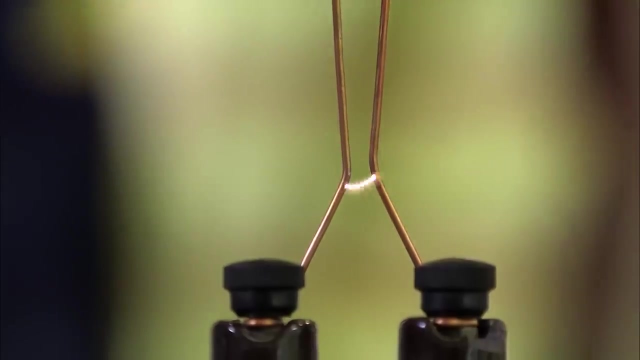 Hot air rises And it takes the electricity with it. So if we cooled the air it wouldn't go up, Wouldn't immediately go up, yeah, And there it goes and it heats back up again. Yeah, That's neat. 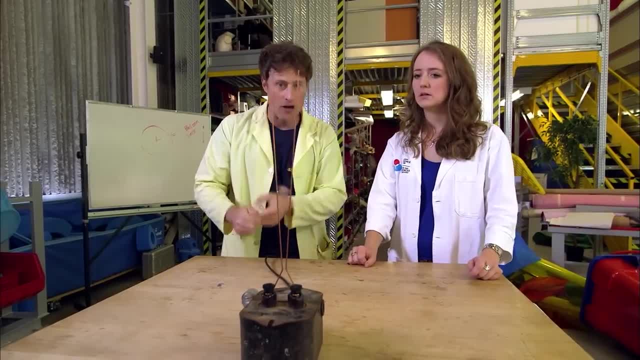 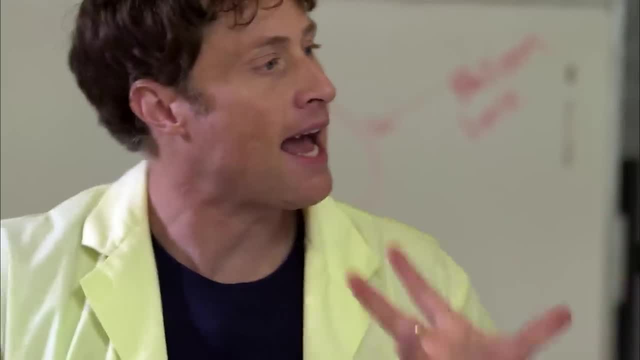 Okay, so we have a Van de Graaff generator, We've got a Jacob's ladder. Are there any other devices that make lightning like this? Ooh yeah, there's other things like the Tesla coil Really hot. Hey, I have a Tesla coil. 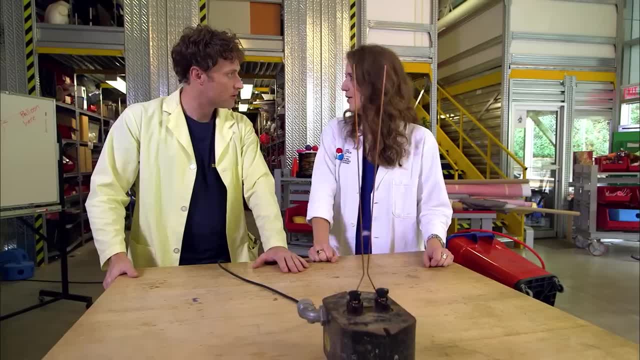 You have a Tesla coil? I do. I've got one at the lab, I've just never known how to hook it up. Oh, I can help with that. yeah, Really Yeah. Okay, let's do it. Let's go back to the lab. 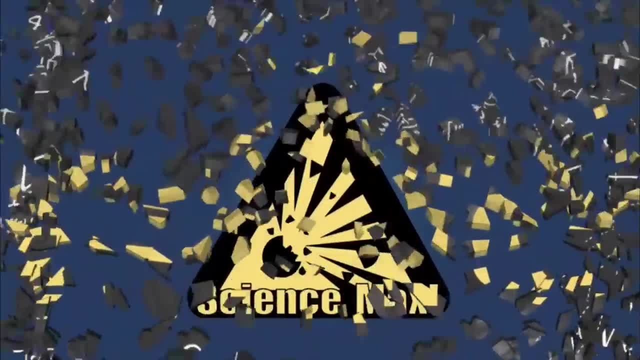 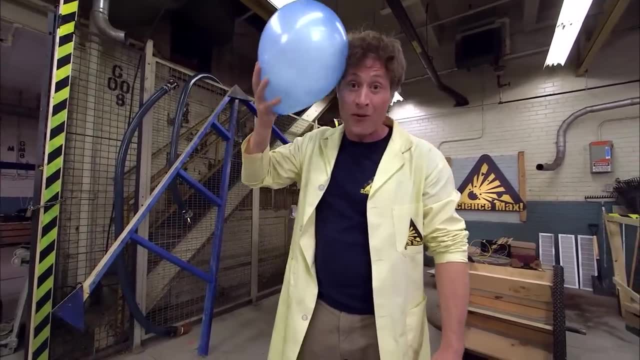 All right, well, yeah, no, yeah, I'll turn that off. okay, Yeah, safety first. Okay, By now you're probably an expert on what happens when you rub a balloon on your head right: The balloon becomes negatively charged. 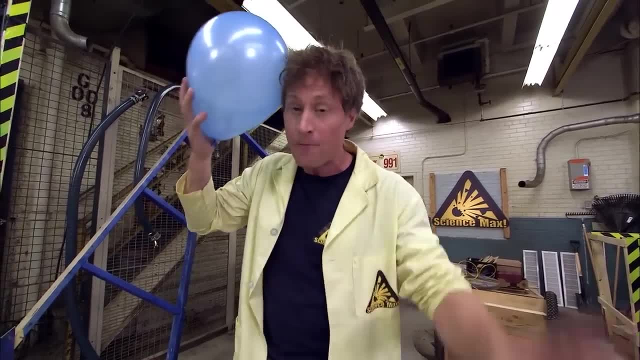 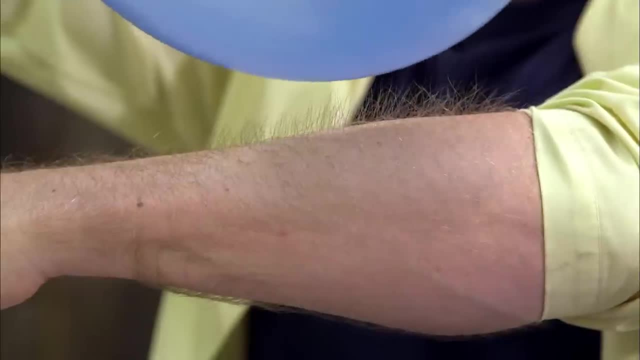 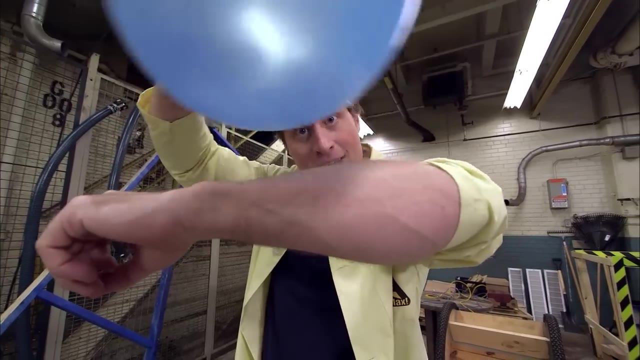 which means it will attract anything of an opposite charge or anything positive or anything that is neutrally charged like. well, like me, Look at the hairs on my arm when I bring the balloon close. Whoa, You see, the neutral charge in my body is being attracted. 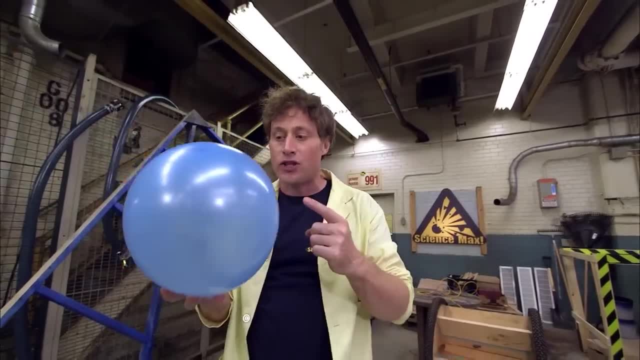 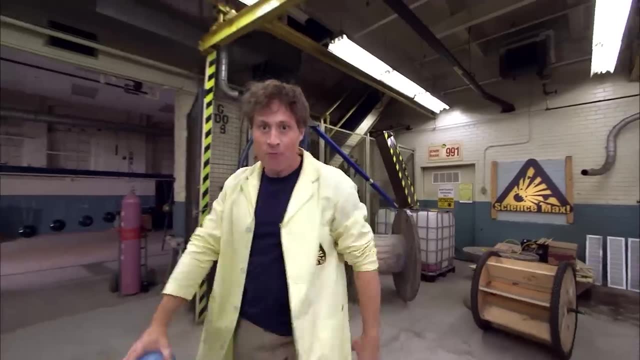 to the negative charge in the balloon. So if something is negatively charged, what happens if you bring something else negatively charged nearby? Well, they'll repel each other. And here's an experiment you can do to make something fly using static electricity. 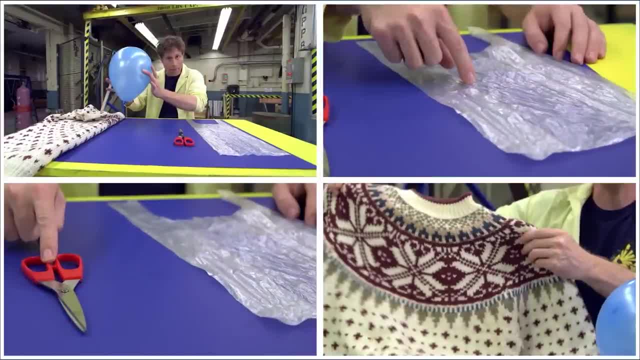 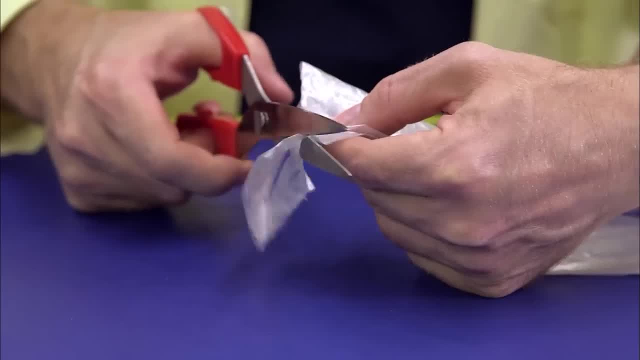 You'll need a balloon, a sweater, scissors and a plastic bag out of the thinnest plastic you can find. Fold the bag up and cut off the bottom. You don't want that part. Then cut another strip from the bag. 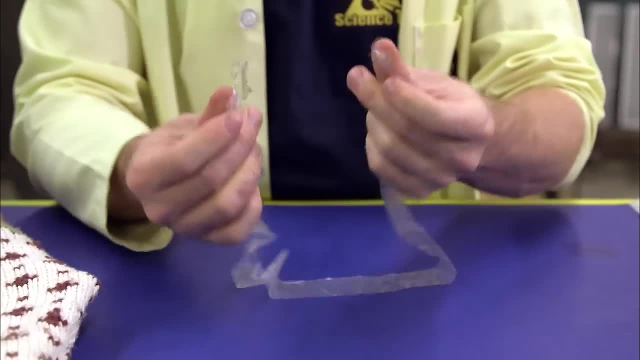 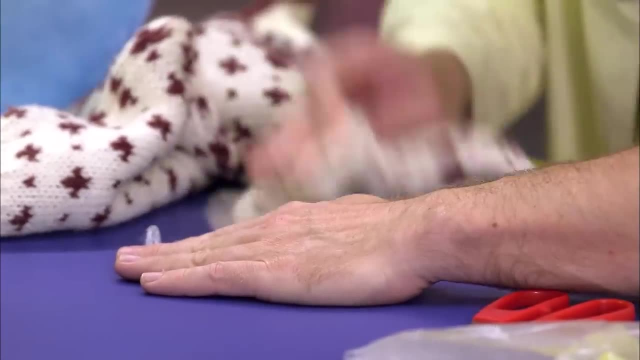 This will give you a hoop of plastic. I find it works better if you break it and tie it again. Lie it flat and rub it with the sweater. This will give it a negative charge. You'll know you've got enough of a charge. 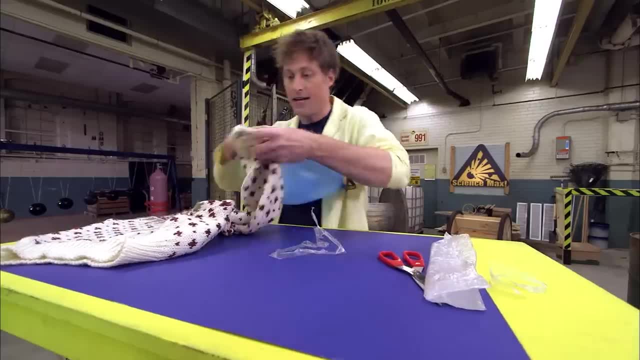 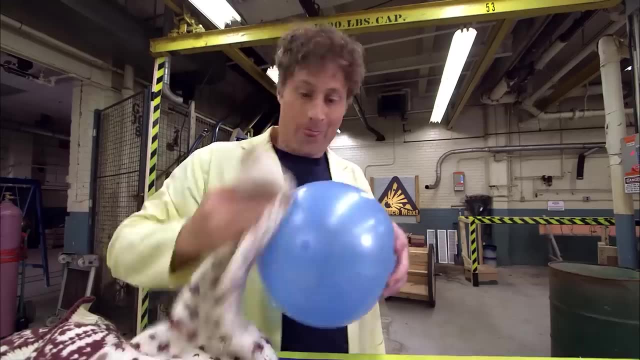 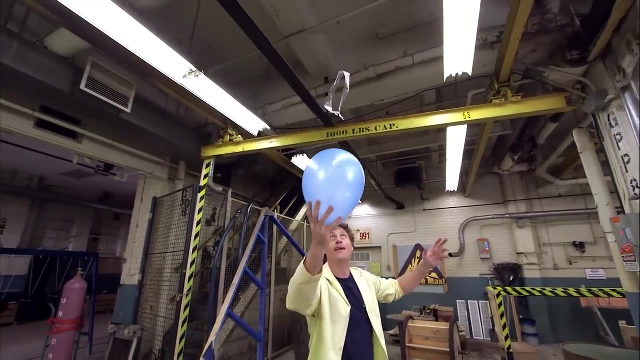 when it really wants to stick to the table. Then take your balloon and rub the sweater on the balloon to charge it up, Because both the balloon and the hoop have negative charges. they repel each other. Then put them together and it will repel. 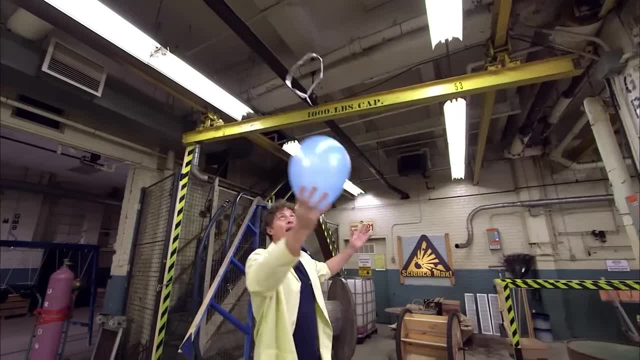 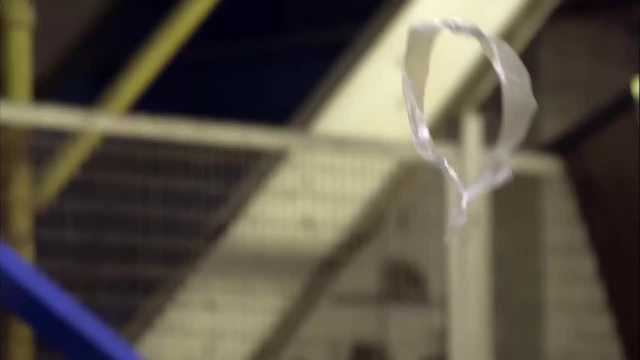 And you can get the hoop to levitate. Ha-ha, It floats, Floating bag of static charge. But here's the thing: You need to keep it away from your body Because if you get close, the bag will stick to you. 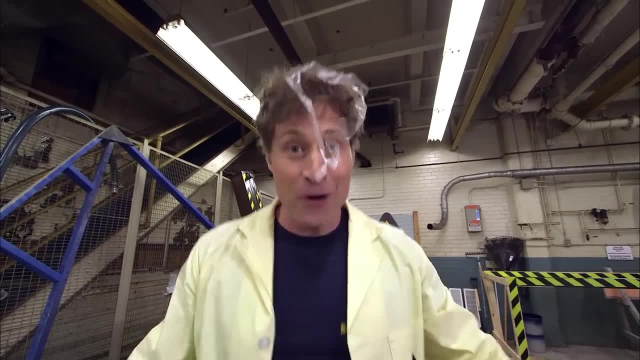 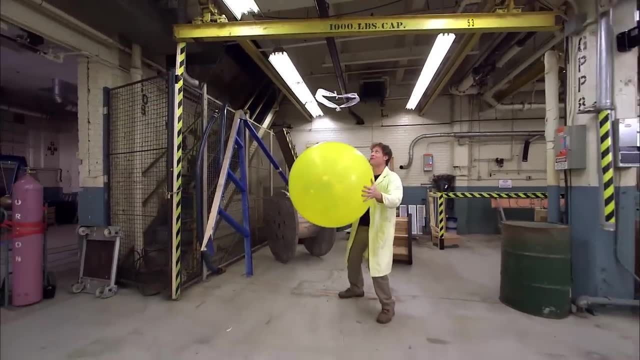 because you're neutrally charged and the bag is negatively charged. Pretty cool, right? Well, let's max it out. Ha-ha-ha-ha-ha. Maxed out floating static ring. Ha-ha, Whoa. 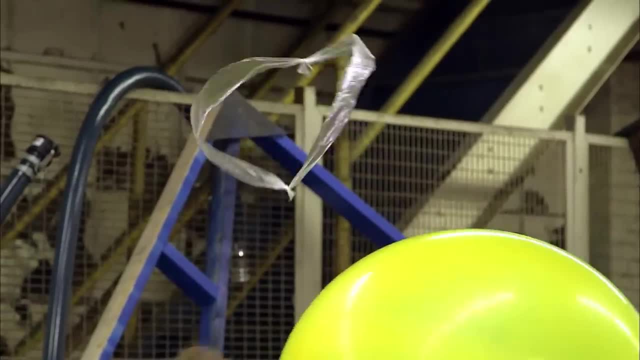 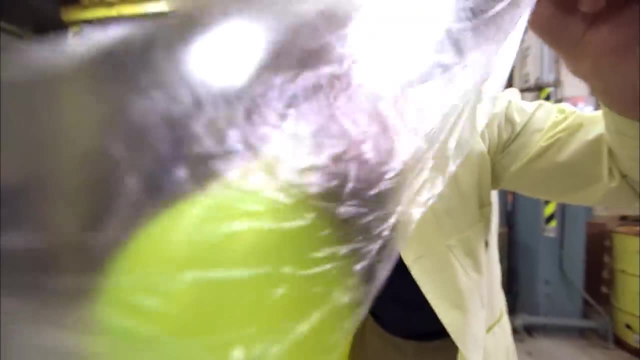 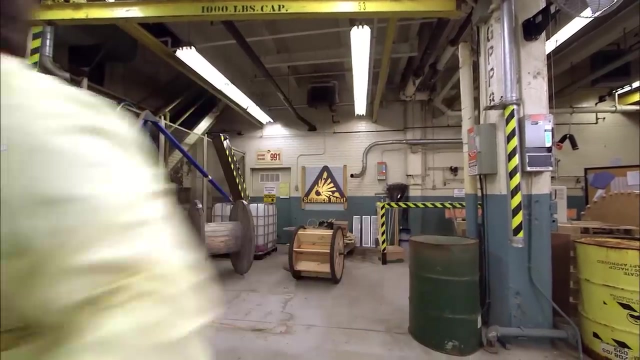 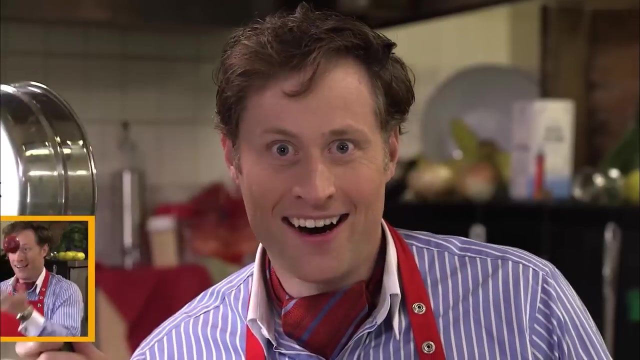 No, Yeah, Look out, look out. Oh no, Oh, sorry about that. Uh, oh well, It was. it was fun while it lasted. Ah, I've got to charge these up again. Being a chef is my absolute passion. 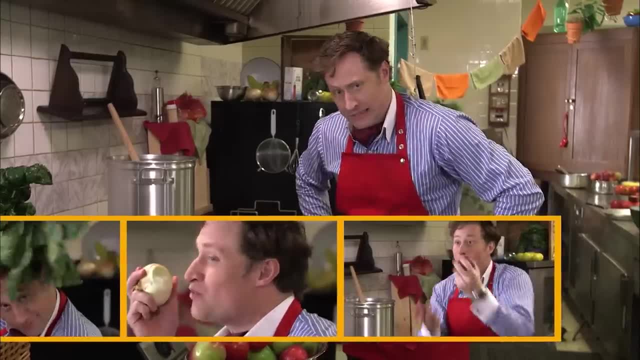 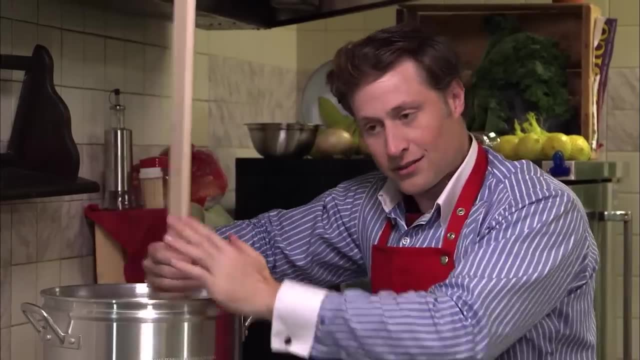 And cooking up science recipes is my speciality. I'm Buster Beaker and this is: Oh hello, I didn't see you there. My name is Buster Beaker and welcome to Cooking With Science. Let's say, for example, I've spilled the salt. 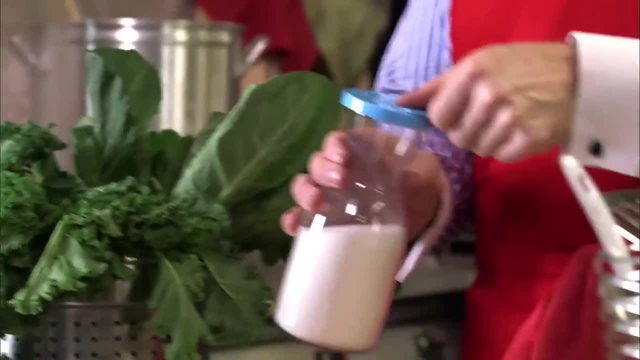 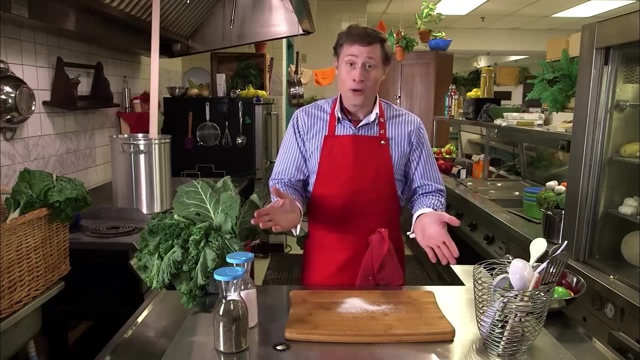 Oh no, look at me, I've spilled the salt. Oh, there's salt all over the place. Not really a big deal, right? All you have to do is clean up the salt, put it back in the container. But oh no, I've also spilled pepper on the salt. 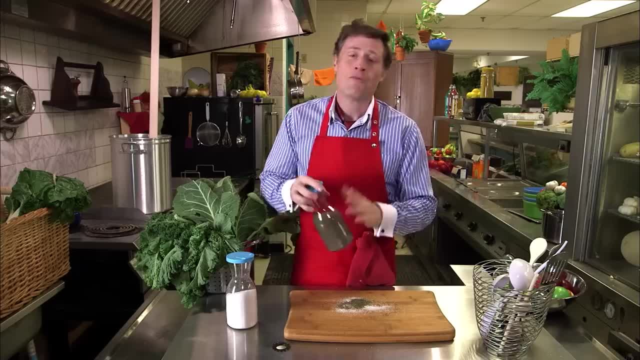 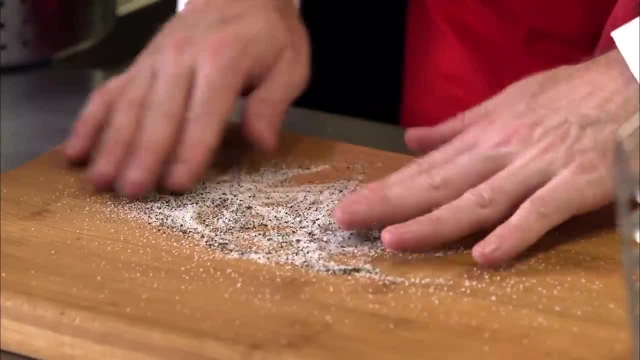 But that's all right. You might be able to carefully separate the salt, But no, oh dear, look, the pepper and the salt are all mixed together. What do I do? Well, here's how you can save the day. 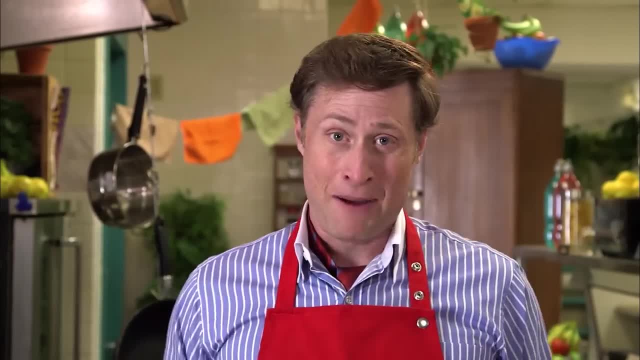 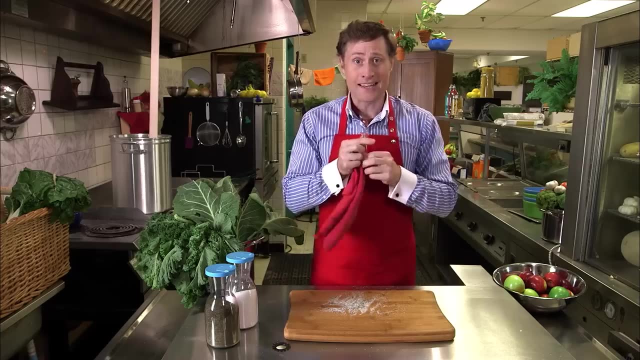 Using the power of science. All you need is a cloth and a plastic spoon Like this one here. Just rub the plastic spoon on a cloth and you'll be charging it up with a negative charge of static electricity, If it's got a negative charge. 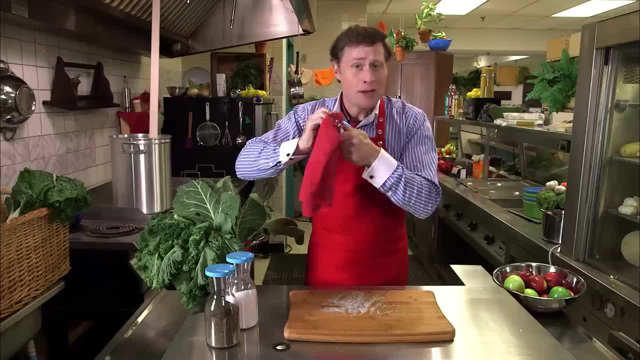 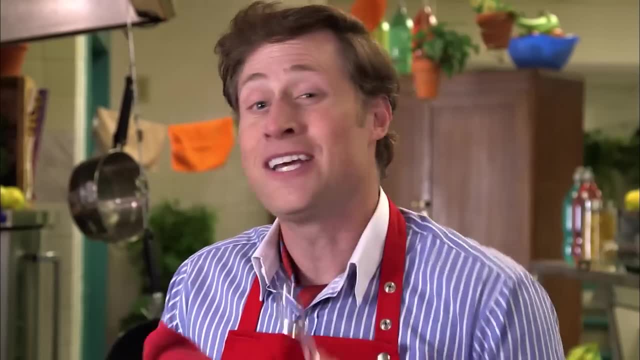 it will attract anything that has a neutral charge. If it's got a negative charge, it will attract anything that has a neutral charge, Just like the salt and pepper. But I know what you're thinking: How will we separate them? Well, here's the answer, my friends. 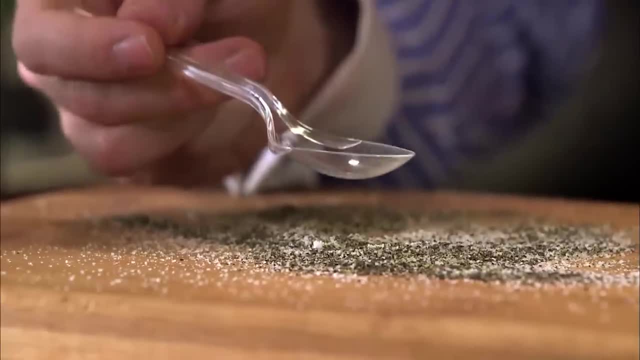 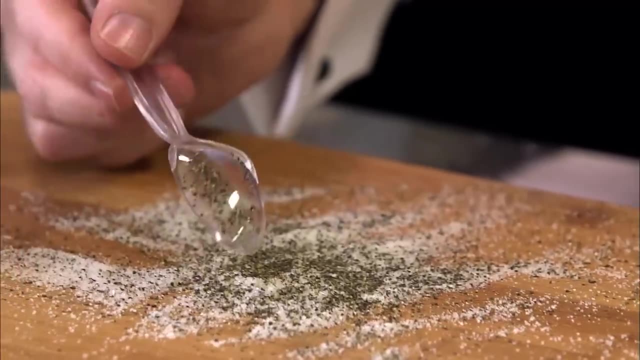 Pepper is lighter than salt. Observe: If you hold the spoon high enough, the pepper will be attracted and make the jump up to the bottom of the spoon, But not the salt, as long as you've got it high enough up, Because the salt is heavier. 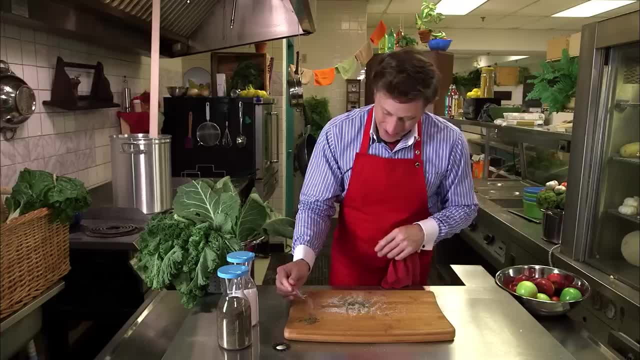 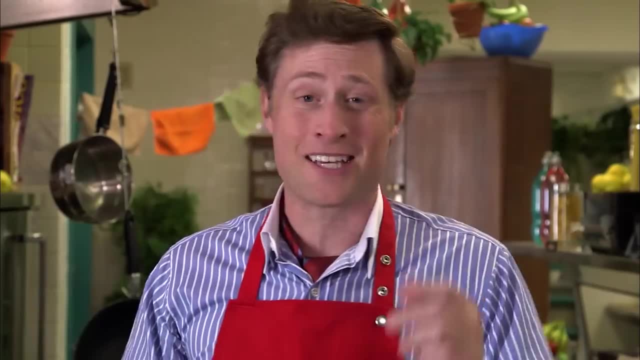 you'd have to bring the spoon closer, which we're not going to do, And if you tap it off to the side, you'll make a nice little pile of pepper. and there you go, separating pepper from salt, using the power of science. 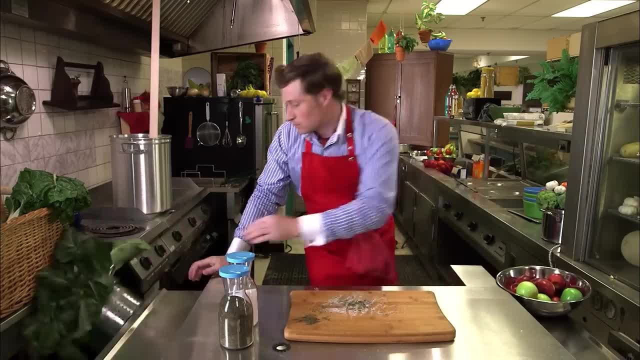 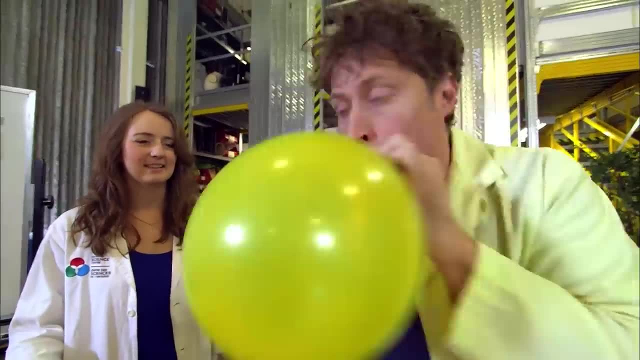 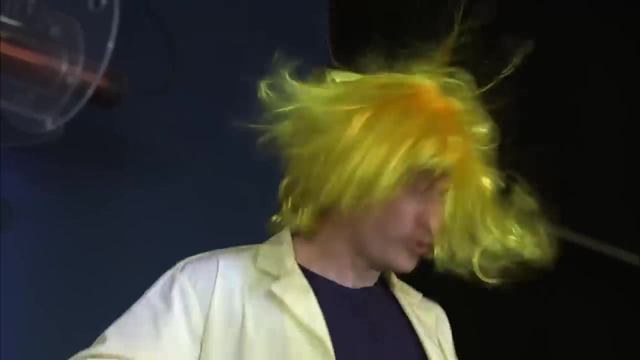 Thanks for watching. Cooking with Science. I'm Buster Beacon. Heather and I have been on a quest to recreate lightning using static electricity. We've gone from balloons to a bandograph, to a Jacob's ladder, each more lightning-y than the last. Finally, Heather suggests we use a. 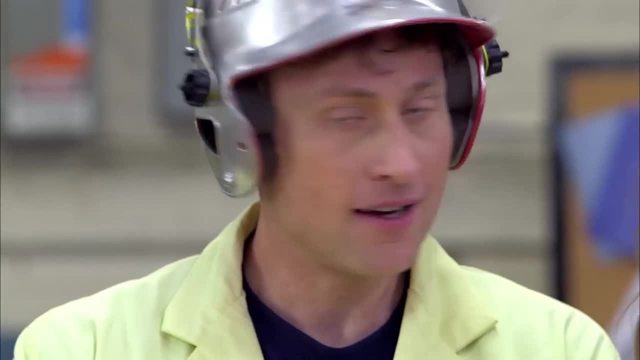 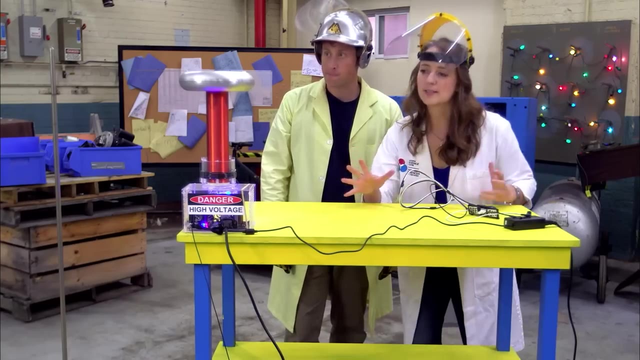 Tesla coil. Oh, is this named after Nikola Tesla? Yeah, he invented it. Oh, one of the founding fathers of electricity, right Right on. I love Nikola Tesla. He's cool. So how does it work? So the way this works is: 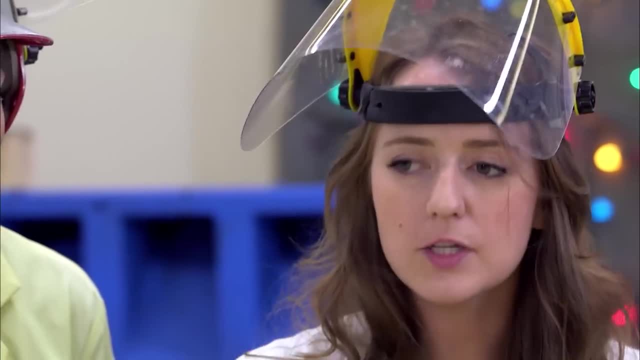 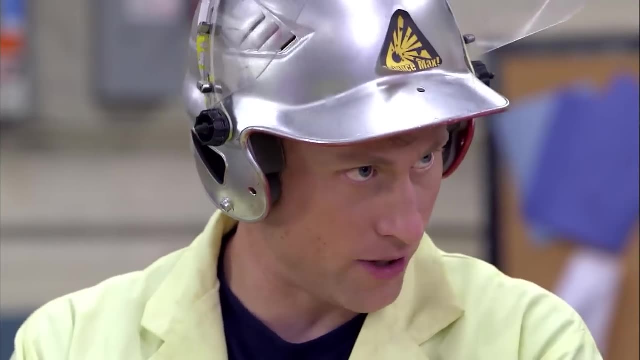 it is a step-up transformer, meaning we take a lower voltage and bring it up and ramp it up to a much higher voltage. Okay so, normal voltage is 120 volts. That's what we have- a normal plug-in socket Typically. we're getting it out of. 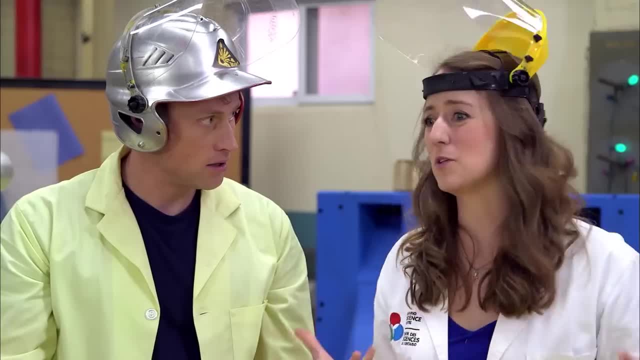 Yeah, exactly, And we're going to ramp that up to really high amounts, upwards of 25,000, maybe even 250,000.. Wow, Volts, That's a lot. And all that charge build-up, we're going to see something. 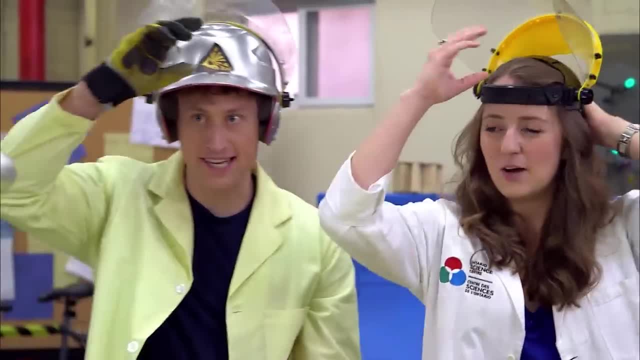 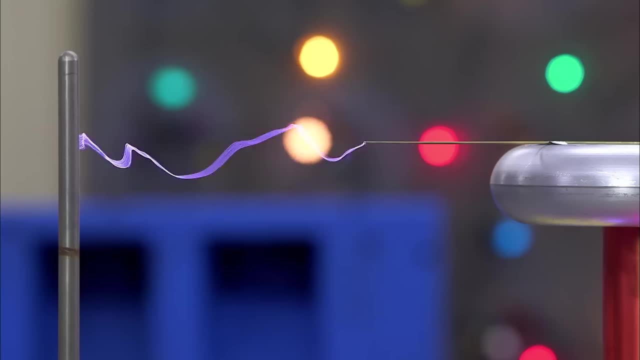 pretty amazing happen. Okay, Do you want to see it? Yes, We stand back there, right? Yeah, Let's check it out. And Whoa, The Tesla coil builds up a charge which jumps through the air to this neutral rod. 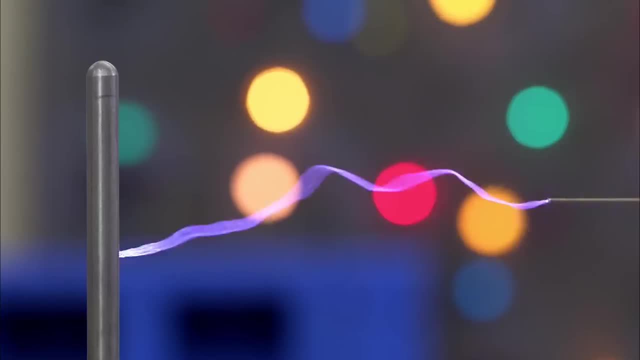 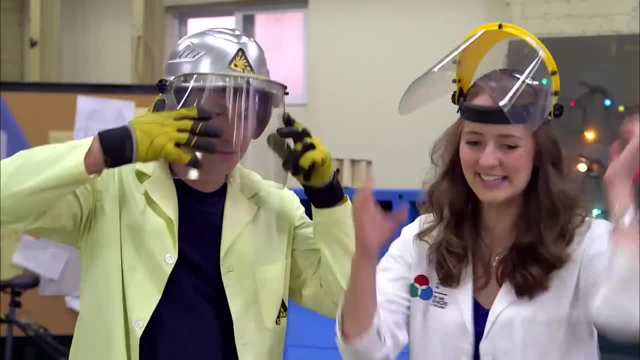 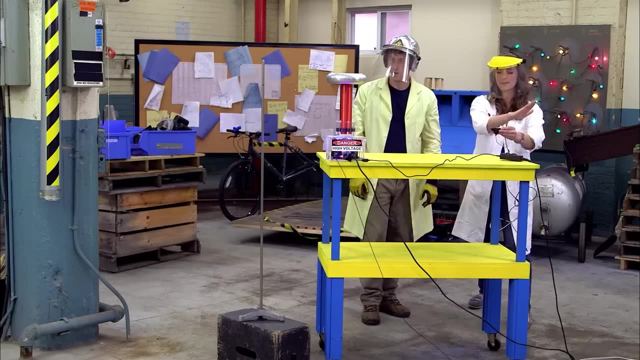 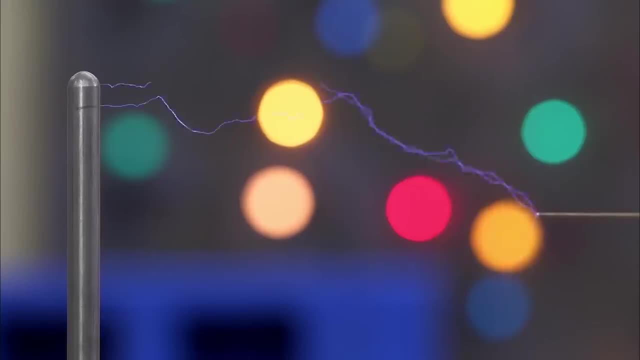 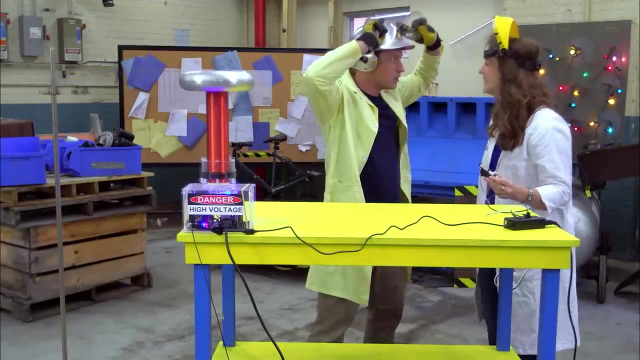 Oh, That's amazing. It's like a scattered lightning bolt. Oh, wait a minute So you can play different notes. Play different notes. I need five minutes. Hold on, Okay, Okay, All I need is five minutes. You know what I was thinking is. 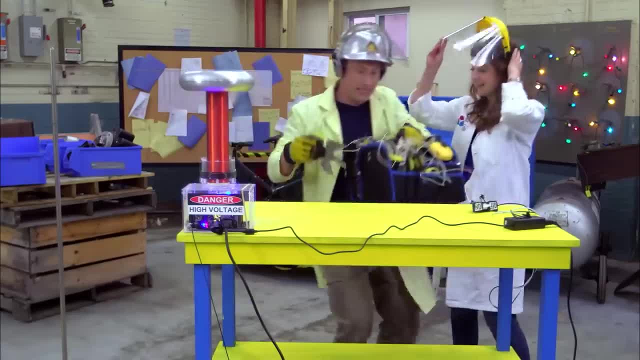 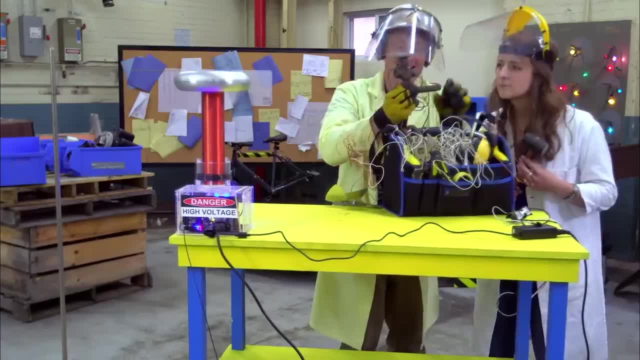 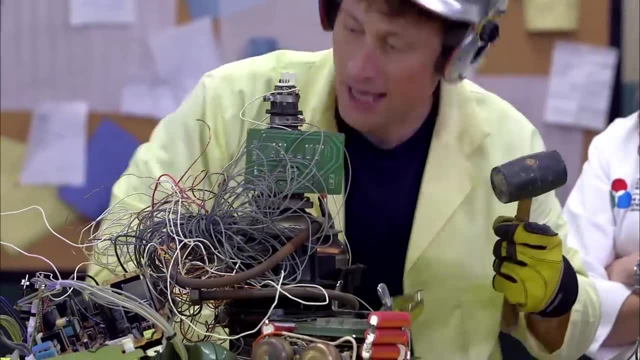 different notes, right, Right, So, Oh, I don't need that either. Hold on, Ah, That's not what I need. Okay, One more thing. Can I get that hammer? Yeah, Okay, Ready to go. So what is this?